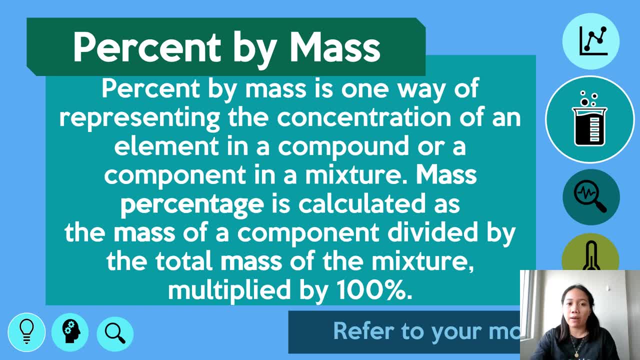 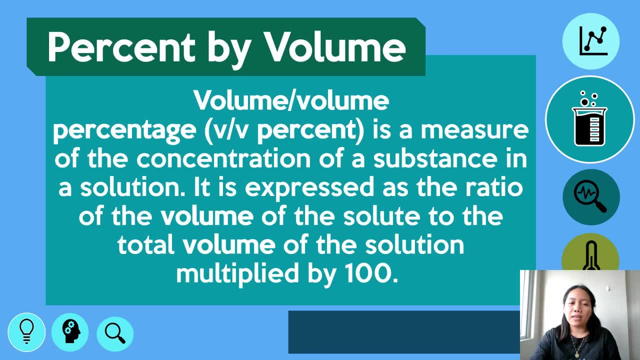 You could also refer to your module for you to read more about percent by mass. Now for percent by volume. It is also almost the same with the percent by mass. The only difference is, of course, we are dealing with volume, from the word itself, percent by volume. 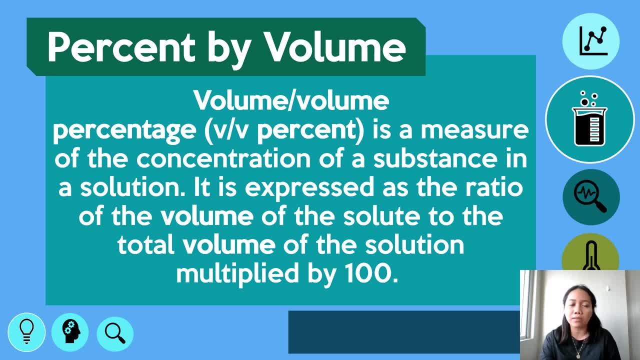 And we also have here a multiplier of 100, because still we are actually looking for a percentage, And if you're going to, If you're going to divide a certain component to the totality of those components, you will always get a value less than 1.. 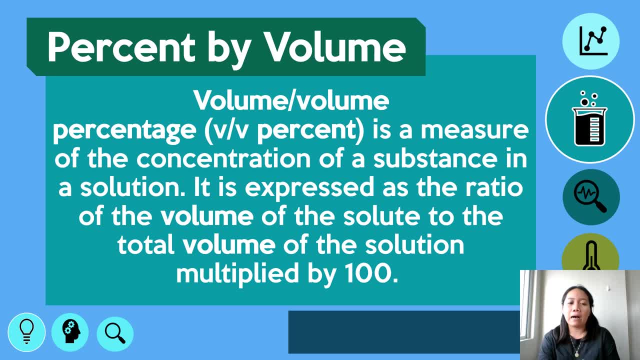 That's why we are always going to multiply. We are going to multiply it by 100 for us to get the percentage Again. you could also refer to your module for the other definition or for more readings about percent by volume and percent by mass. 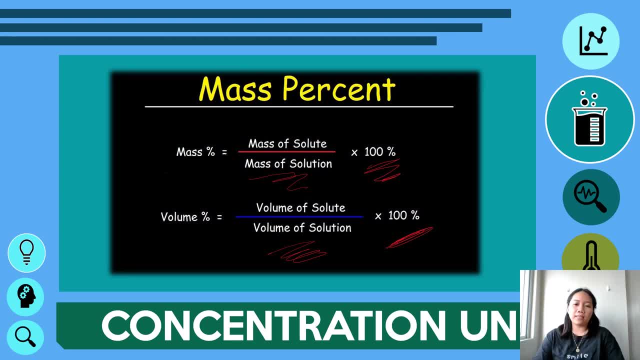 The formula of our percent by mass and the percent by volume. it is just simply, as mass percent is equal to the mass of your solute divided by the mass of your solution multiplied to 100.. And for the volume, you have volume percent or the percent by volume. 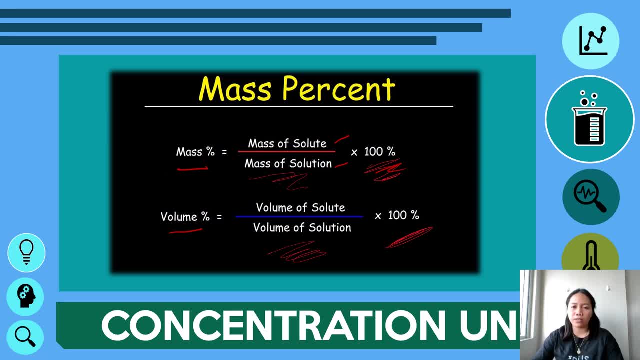 is equal to the volume of your solute divided by the volume of your solution, multiplied to 100%. Now again, please don't forget that in a particular solution, we always have our solute And we always have our solvent And, of course, if you're going to add these two components, 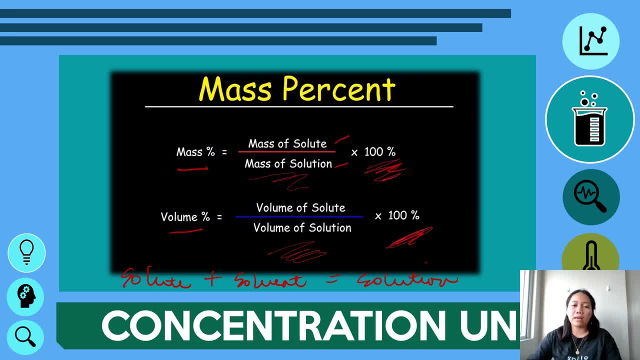 you will come up with a solution. Now, that would be one of the most important foundation if you're going to solve for solution-related problems, because it will need that particular knowledge, knowing that solute and solvent, or the addition of a solute and solvent, will give you a particular solution. 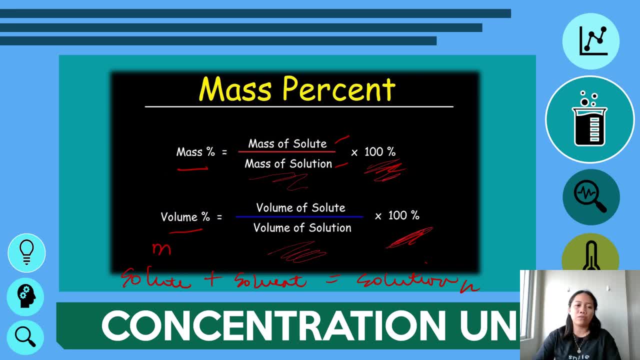 In this case, if you're going to have a mass of your solute and a mass of your solvent, you will always have the total mass of your solution. Now, why is it important? Because, as you can see in the denominator, you were not asked what is the mass of the solvent. 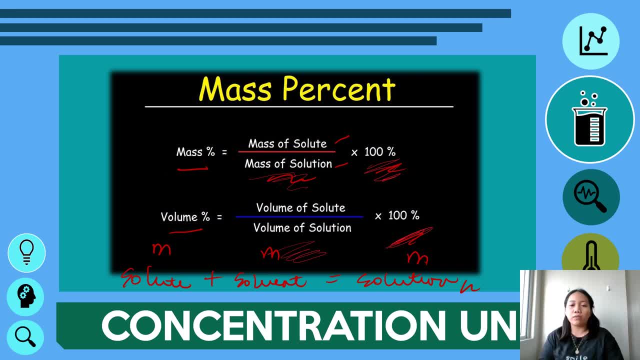 Instead, you were asked: what is the mass of the solution? So there are some problems wherein it is so tricky: it will just give you the mass of the solvent and you will just have to write it down, Thinking that it is the mass of the solution. 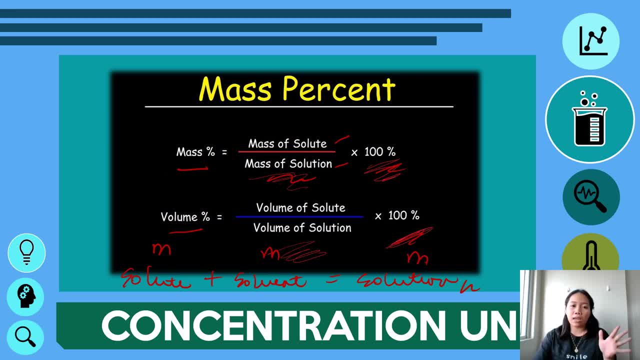 But no. So make sure that you read the problem very carefully, because there are problems that are very tricky. So in that case all you have to do is to add first the masses of your solute and the mass of your solution for you to get the mass of your solvent. 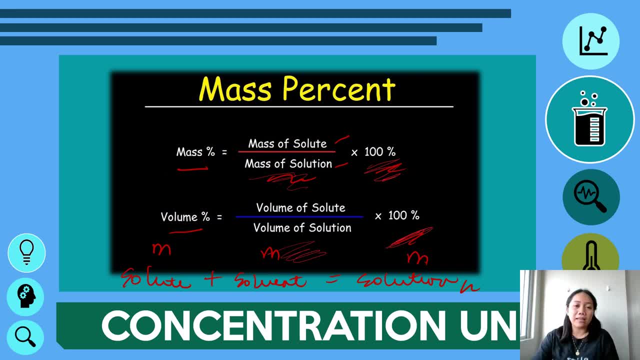 for you to get the mass of your solution. In that case you're denominator. This is also true to the volume percent or the percent by volume. So for the volume of your solution you have to add the volume of your solute and the volume of your solvent. 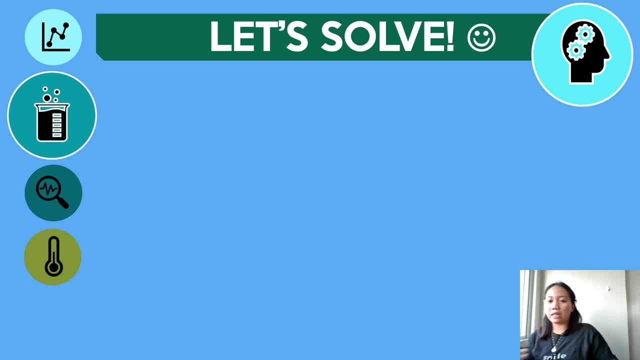 Now let's try to solve one problem that involves percent by mass. So I have here a problem: 6 grams of urea was dissolved in 500 grams of water. Calculate the percentage by mass of urea in the solution. So in this case it is very important. 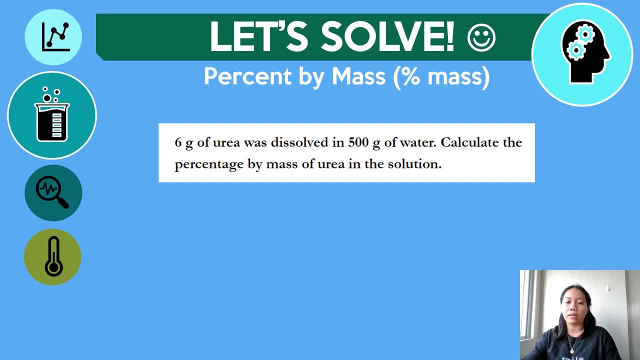 that you identify the mass of the solution. So in this case, it is very important that you identify the mass of the solution. So in this case, it is very important that you identify the mass of the solution, your solute and the solvent. 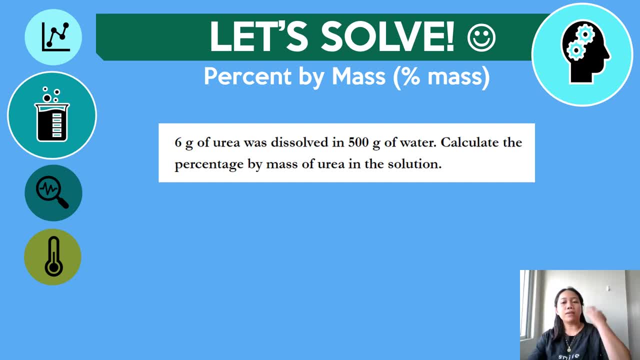 Remember what I have said on the previous slide, that knowing those two is very important, especially if we are dealing with solution-related problems. So you have: 6 grams of urea was dissolved in 500 grams of water, Since urea was the one being dissolved in water. 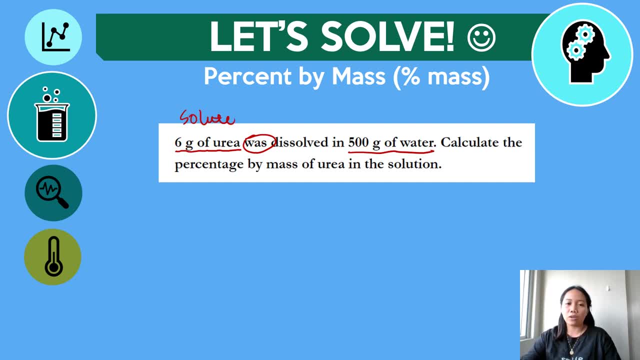 that means urea will be your solute and your 500 grams of water will become your solvent. Calculate the percentage by mass of urea in the solution. Calculate the percentage by mass of urea in the solution. Percentage by mass of urea in the solution. 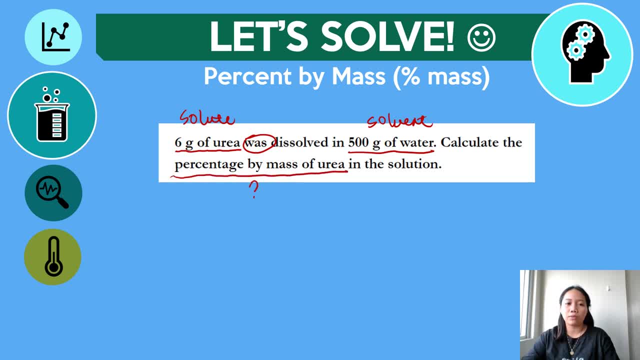 So the percentage by mass of urea, which is your solute, is the one that is being anode. So first you have to write first the formula, of course. So it's percent by mass is equal to, or m over m. then you have the mass of your solute all over the mass of your solution. 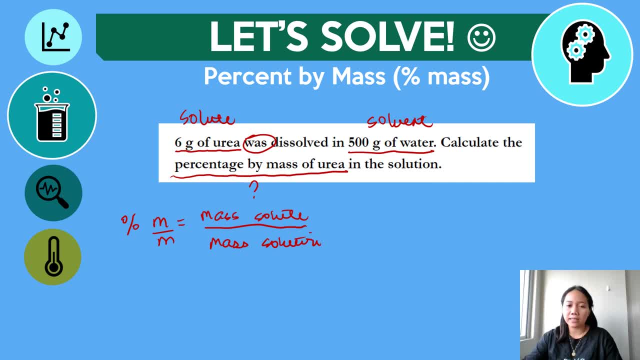 And, of course, since this is percent, you have to multiply it to 100.. Now, given that our mass of solute, it's very good that you label everything, because it will be very important if you're going to substitute now the values. 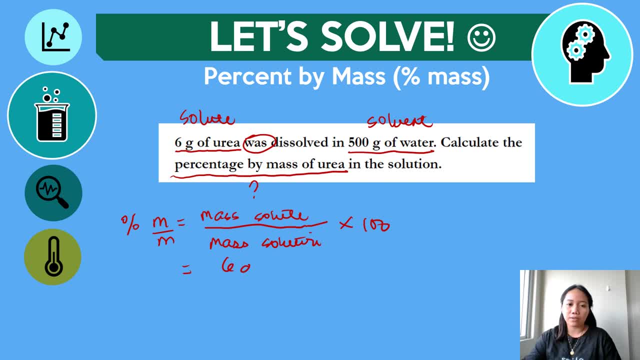 So you have the mass of your solute, which is 6 grams divided by. it would be 6 grams of urea divided by. we know that this is your solute and this is the solution. So if you're going to add that one, that will give you the mass of your solution. 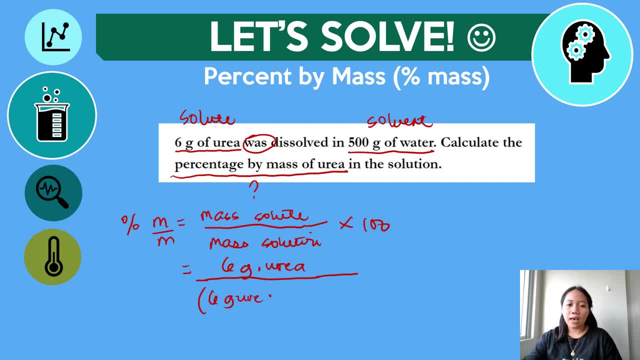 So you have 6 grams of urea added to, you have 500 grams of water. So that would be your denominator, because again, that is the mass of your solution Multiply to 100. So in this case, if you're going to solve, you're going to cancel now the grams. 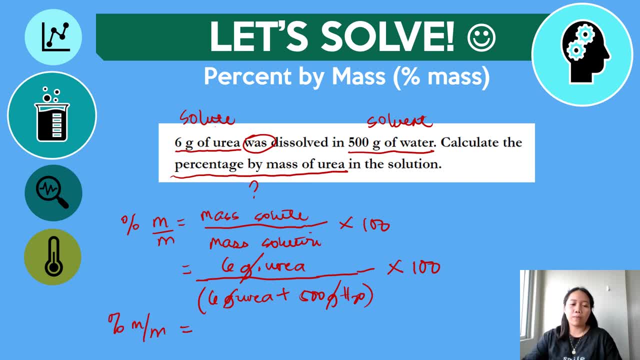 And the percent m over m would be 1.1.. So in this percentage we come up with, we come up with idea that we're going to have two decimal places okay in our class in the percent, in the percentage, for us to have the same answer. 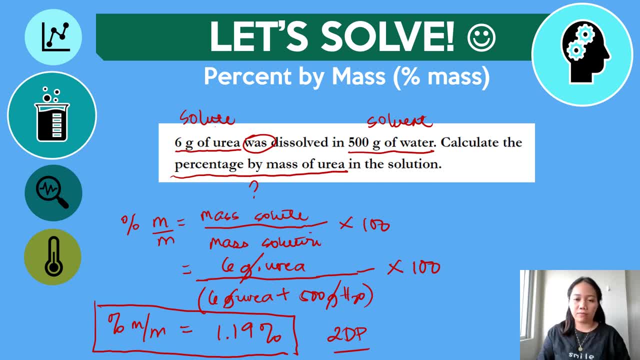 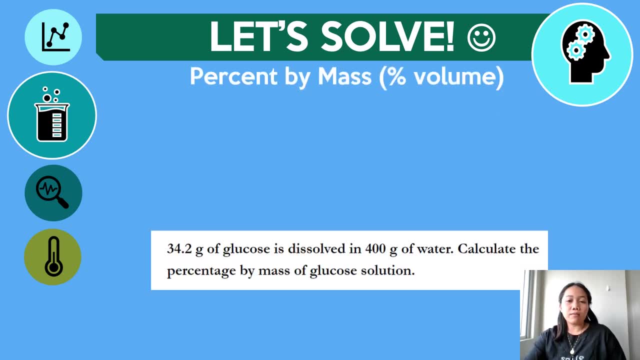 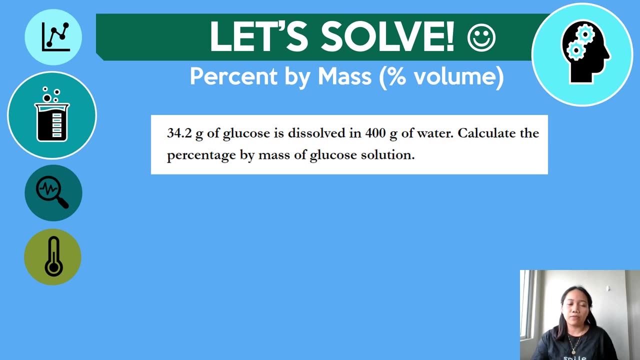 So later on, of course, we need to follow now the proper significant figure only here Now. another problem related to percent by mass is this problem: You have: 34.2 grams of glucose is dissolved in 400 grams of water. 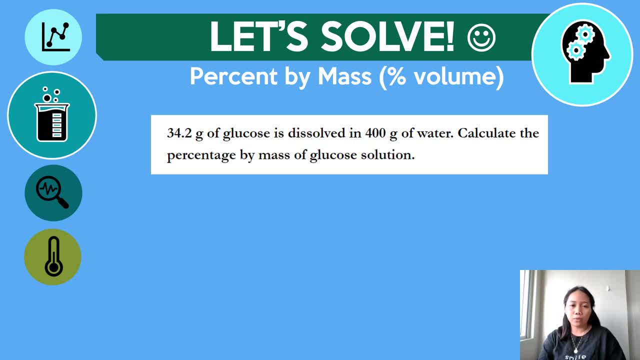 Calculate the percentage by mass of glucose solution. So the one that is asked or the one that is unknown, is the percentage by mass of your glucose solution. So this will be our X, or that is the unknown. You're 34 grams of glucose. 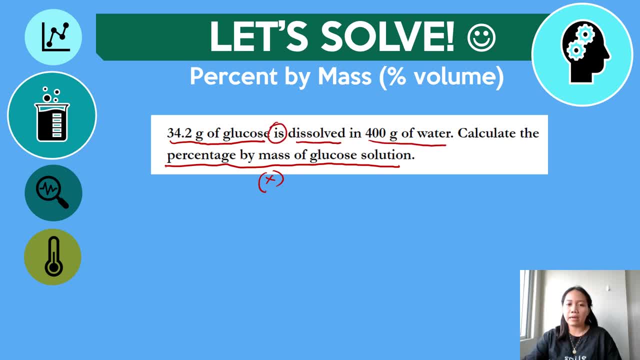 It's the one that is being dissolved in 400 grams of water, making your 34.2 grams of glucose your solute, And your 400 grams of water will now become your solvent. Now, writing the formula you have: percent m over m is equal to the mass- okay, the mass- of your solute, which is the unknown, because it's the glucose. 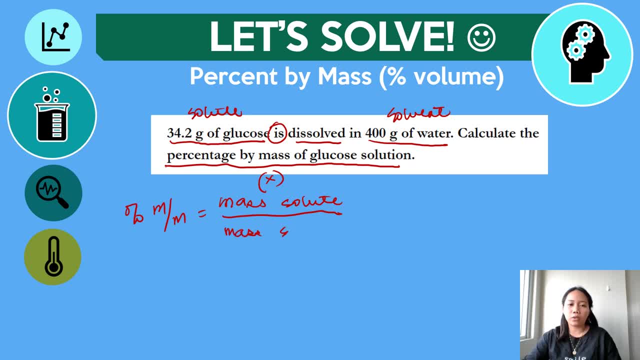 divided by the mass of your solution, Times 100, and you have now your formula. Then, for the mass of your solute, it is given in the problem, and that is 34.2 grams of glucose divided by. of course, we know that the addition of the two will give you the solution. 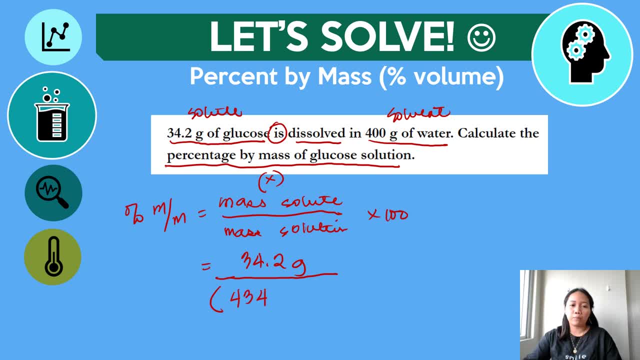 So if you're going to add that one, that is 434.2 grams, So cancel now grams, multiply it to 100. And that will give you an answer of 7.88%. That is now the percent by mass of your glucose solution. 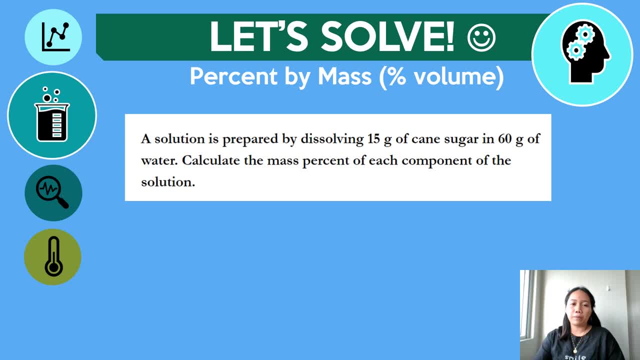 Another problem that we have here is a solution prepared by dissolving 15 grams of cane sugar in 60 grams of water. Calculate the mass percent of each component of the solution. So a while ago, the previous problems are just asking you one component of the solution. 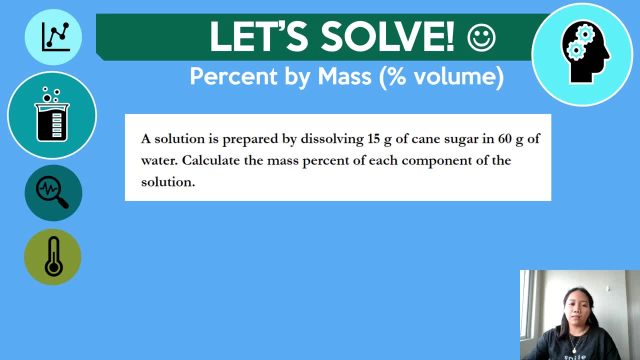 Wherein most likely it is the solute. But in this problem, you were asked now the percent, or the mass percent of each component, Meaning you have now an X and you have now a Y. So if you're going to add these two variables- because this is percentage- you should have an answer of 100%. 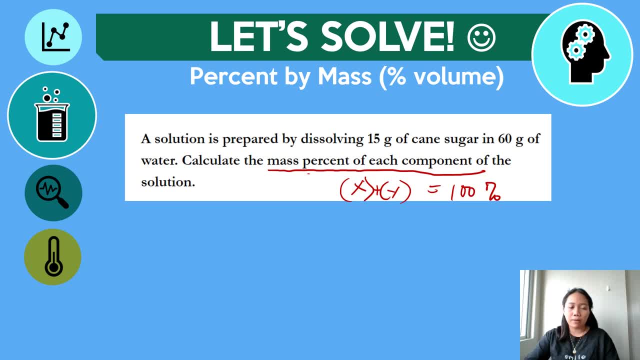 If not, then there will be a problem or there are problems that you have made with regards to your solution. So this is just for checking And we will try this one as we go along our discussion. So, since a solution is prepared by dissolving the 15 grams of cane sugar in a 60 grams of water, 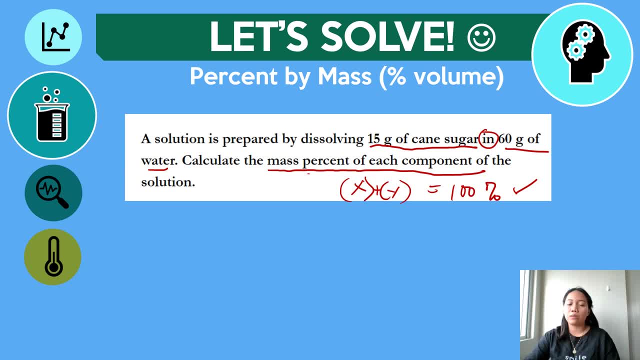 we know now that your 15 grams of cane sugar was the one being dissolved, That means this will become your solute And the 60 grams of water will now become your solvent. So in this case, writing down the formula, it's percent M over M is equal to. 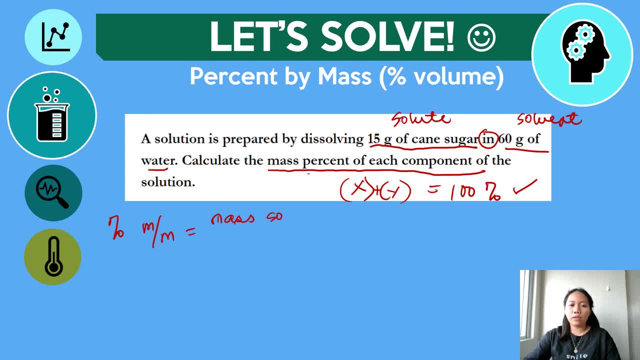 the mass of sugar, So the mass of your solute divided by the mass of your solution, multiplied to a hundred percent, Knowing that the mass of our solute is the 15 grams, then you will have 15 grams of the cane sugar divided by the total mass. 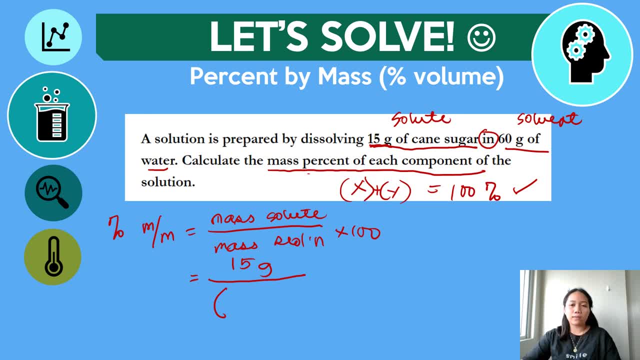 If you're going to read, you have 15 grams of cane sugar, which is the solute, and 60 grams of water, which is your solvent. So all you have to do is to add the two So for you to get 75 grams. cancel now grams and you will get a value of 20.00%. 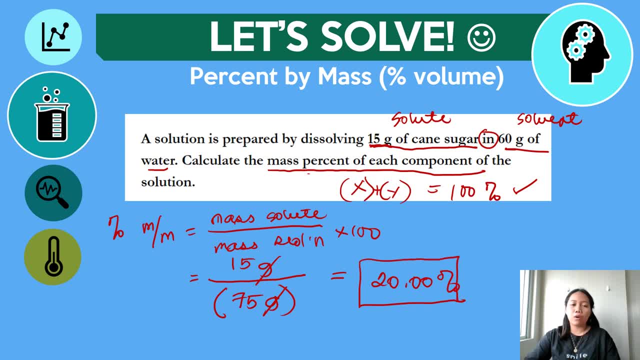 This is now the percent by mass of your cane sugar. Okay, this is just for the cane sugar. Now let me just write it down here, below Paramarantine space for the water. Okay, so this is for the cane sugar. 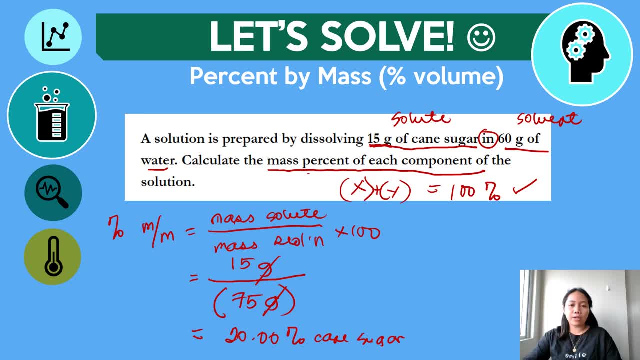 Now, how about for your other components? This is your component, which is water. So our water is 60 grams. okay, divided by your 75 grams, which is the total, then that will give you an 80.00%. 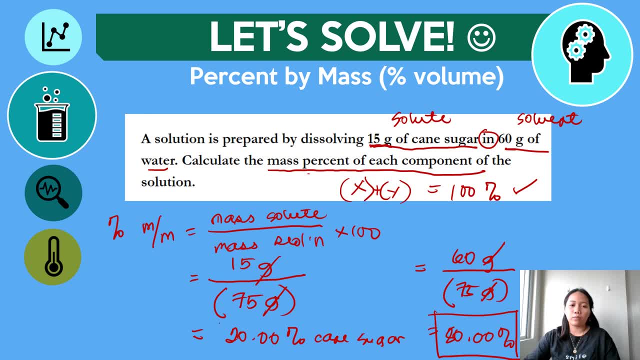 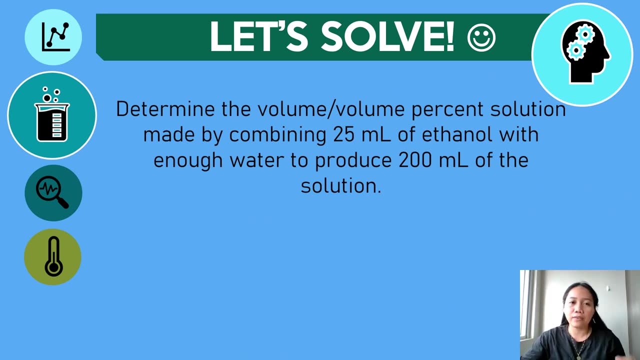 If you're going to add the two components, the 20% and the 80%, that will give you a hundred percent. That means that your answer is definitely correct. Now let's have a look at the other components. So let's have the percent by volume. an example of a percent by volume: 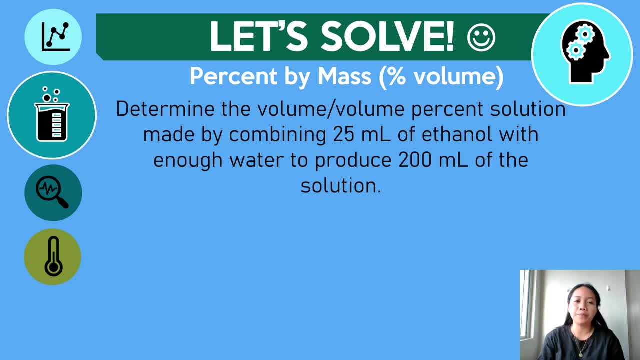 Sorry, that's percent by volume. So determine the volume to volume percent solution made by combining 25 ml of ethanol with enough water to produce 200 ml of your solution. So, as you can see, 25 ml is very clear. That would be your solute, because it is the one that is being mixed to another solvent. 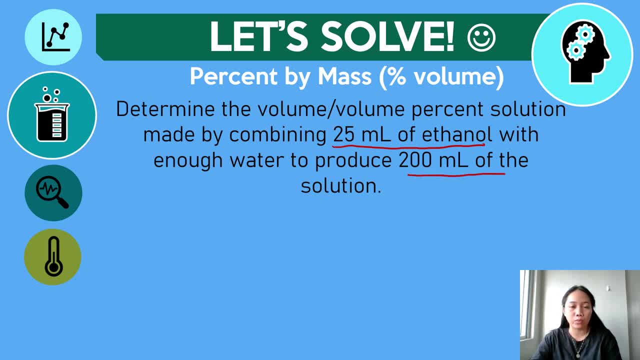 Okay For you to get a 200 ml solution. So again, there are some problems that are very tricky. So in this case, if you're going to read it very carefully, the 200 ml is already your solution, So you don't have to add the two. 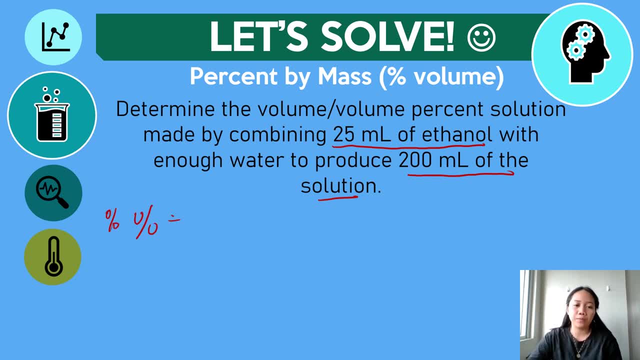 So you have: percent volume over volume is equal to the 25 ml of your ethanol. That would be divided by 200 ml of your solution. Okay, So instead of adding the two cancel, cancel and multiply it to 100, you will get now a 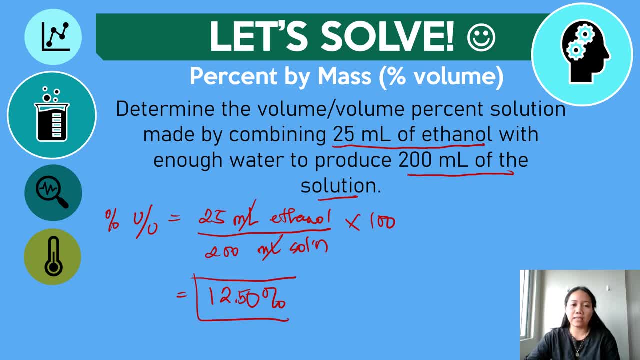 value of 12.0.. Sorry, 12.50%. So that is now the percent by volume of your ethanol. Okay, If you're going to look for the percent by volume of your water, then all you have to do is to minus 225.. 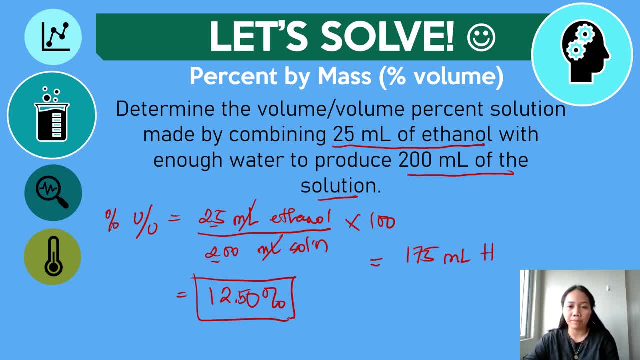 So that means you have 125 ml of your solution, 275 ml of water and that is your solvent, all over 200 ml of your solution and if you're going to solve for the value of that, that would be 87.50 percent, and to add the two percent that we have. 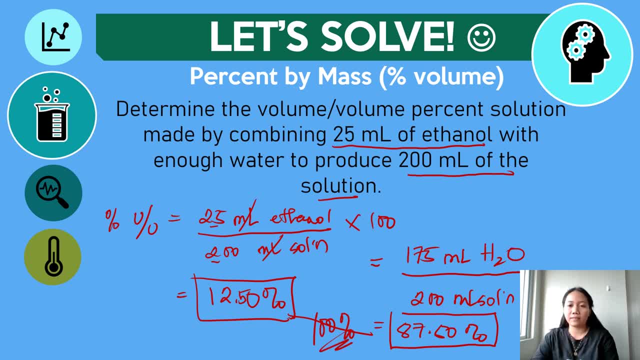 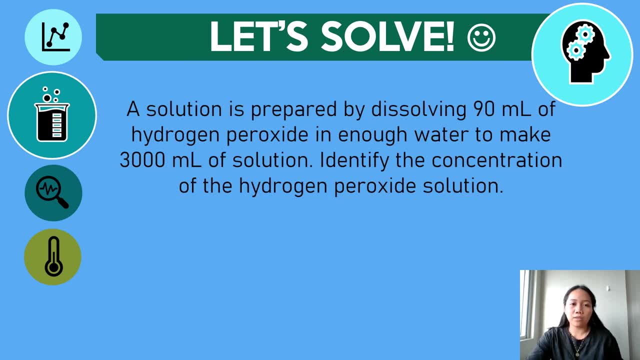 here it will total to a hundred percent. so that is now the percent by volume. another example we have. a solution is prepared by dissolving 90 ml of hydrogen peroxide in enough water to make 3000 ml solution. identify the concentration of hydrogen peroxide solution, so the one that is. 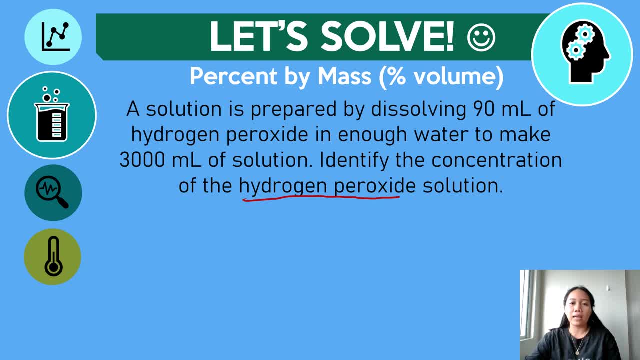 unknown- is actually your solute because, as you can see, it is the 90 ml of hydrogen peroxide that is being mixed to another solvent for you to get a 3000 ml solution. so again, you write the formula that would be: percent v over v is equal to the volume of your solute. 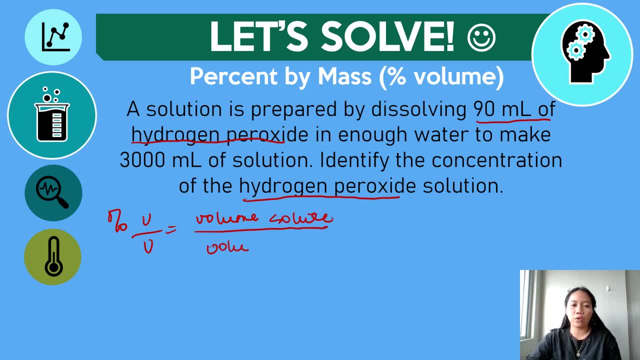 all over the volume of your solution multiplied to a hundred percent. so the volume of your solute here, which is the hydrogen peroxide, is 90 ml divided by the volume of your solution, which is already given, and that would be 3000 ml multiplied to a hundred. that will give 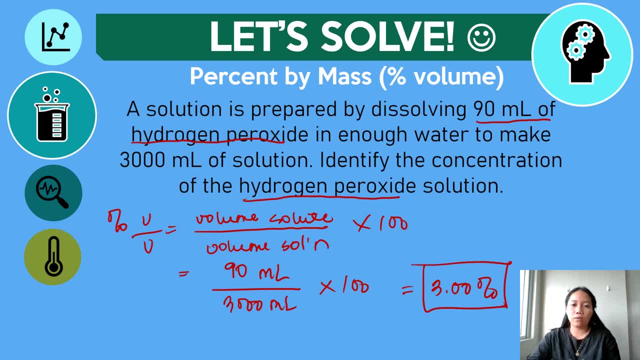 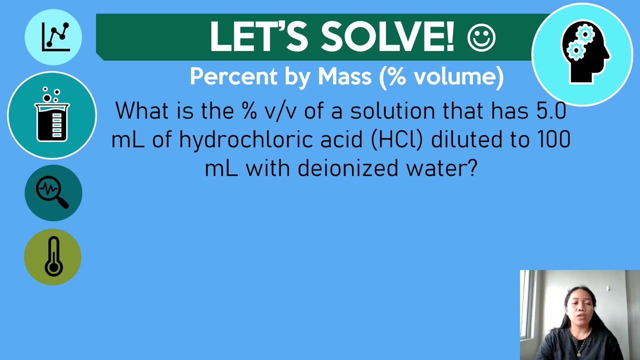 you: three point zero, zero percent. so the answer here, which is the hydrogen peroxide solution in a percent by volume concentration unit, will be three point zero percent. three point zero, zero percent by volume. how about this last problem that we have for the percent by volume? so what? 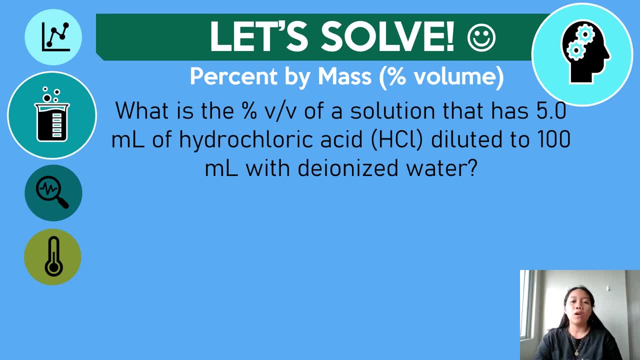 is the percent, volume by volume, of a solution that has five point zero ml hydrochloric acid diluted to 100 ml deionized water. now, in this problem you have, what is the percent by volume of a five point zero ml hydrochloric acid diluted to a hundred ml? 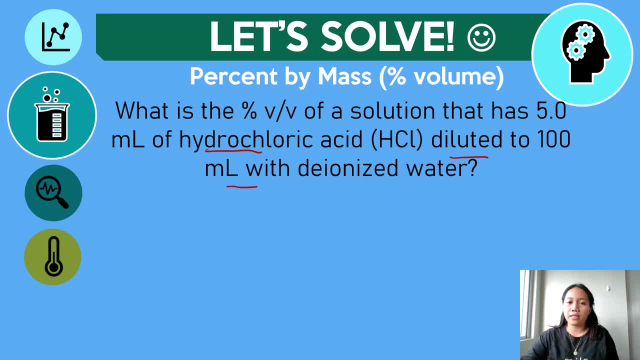 with the ionized water. so you can see the word diluted there and you might not be familiar with dilution. but if you're going to dilute something- take for example in a beaker- okay and you're, you have five ml of hydrochloric acid and when you say you're going to dilute it, 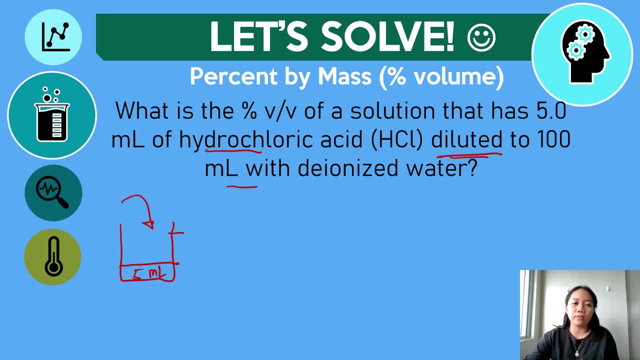 to 100 ml. that means you're going to add a solvent up unto the 100 ml mark of the beaker and in that case that would be the dilution. you are actually lowering the concentration of the acid okay, which is, in this case, hydrochloric acid. the importance of dilution: 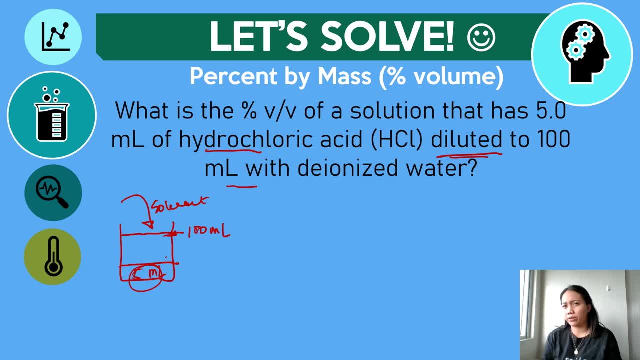 of course, to have compounds or, sorry, to make acid a little bit concentrated or not concentrated, rather okay compared to that of a pure acid. so, because there are a lot of problems, especially to acids that are very, let's say, volatile, it could actually hurt your skin. okay, nakaka, sooner shot. 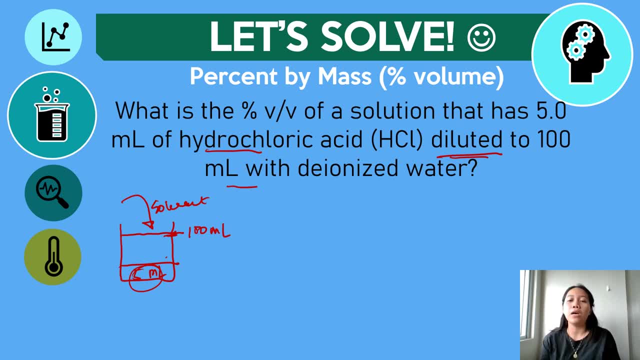 acid, sulfuric acid. that's why we are going to dilute some to avoid that kind of situation. so in this case, if you're going to understand the whole problem, um the 100 ml, there is already the volume of your solution. so the percent volume by volume would be: you have 5.0 ml of. 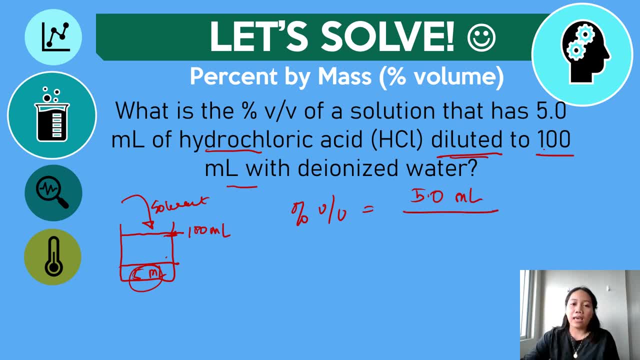 your hydrochloric acid- because it is the one that was asked- and divided by the 100 ml of your solution times 800, and if you're going to solve for that, the answer would be 5.00 percent. that would be the percent volume by volume of your hydrochloric acid in this problem. 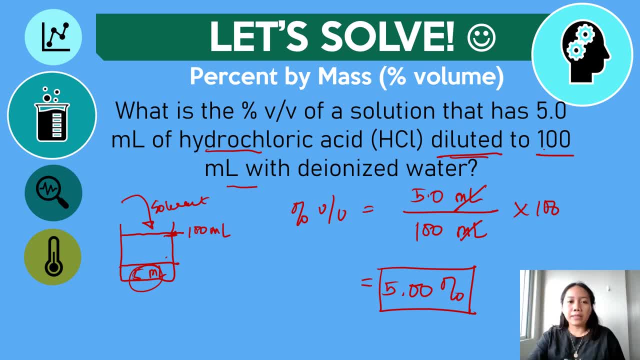 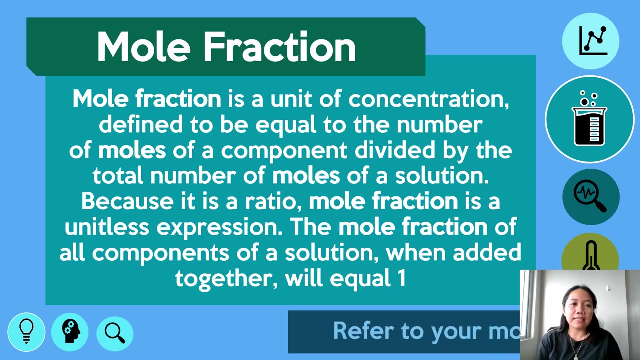 now we're done with the percent by mass and the percent by volume. so it's quite a bit easy compared to the others we will see later. so let's now have mole fraction. so again, you could also refer to your module for the definition of mole fraction and for you to understand it more. so in mole fraction it is again another unit of. 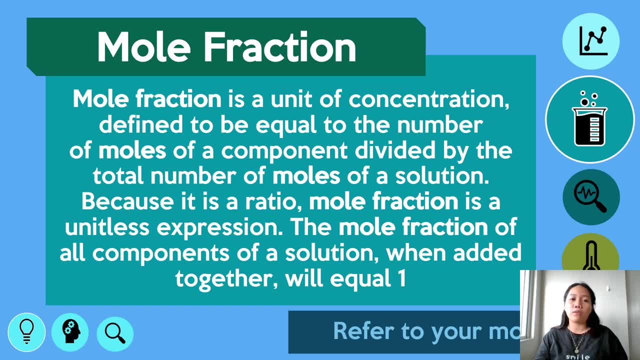 concentration that is defined to be equal to the number of your moles of component divided by the total moles of the solution. so in this case, when you say component, again that is just simply dissolute, and dissolvent, that is, the components of a certain solution. so in this case, when you 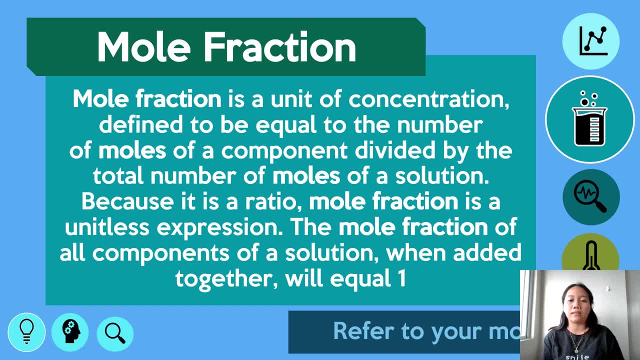 say component, again that is the components of a solution. so in this case, when you say component, again that is the components of a solution. so in this case, when you say solution is a combination of your solute and your solvent. now, if you're going to solve for the mole fractions of every 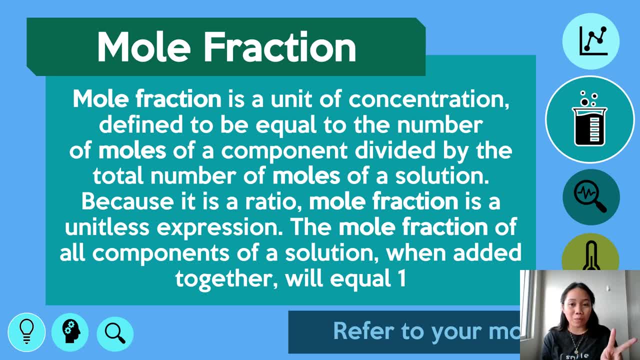 components of a solution. i'm not just saying there are only two components in a particular solution, but there are also cases wherein you have three, four or five components of a certain solution or a mixture. in that case you will have also three, four or five mole fractions respectively. now, because you have a lot of convert in that case. 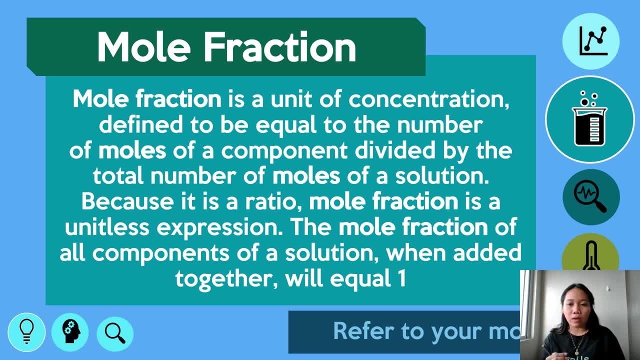 you have a lot of mole fractions. if you're going to add that one, it should sum up with one. okay, it should sum up with one, and in that case, that is the way. how are you going to check if your answer is correct now? if not, if there is a little bit of a discrepancy, like your answer is around 7.2. 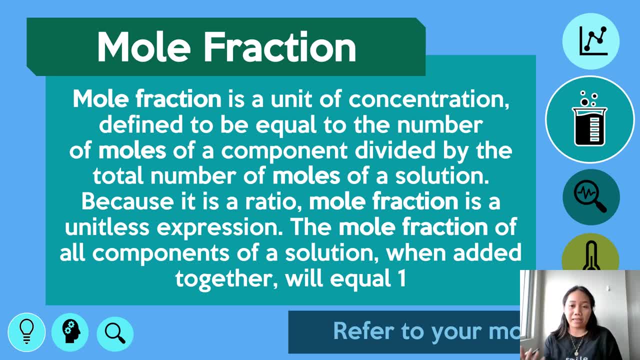 i know, sorry, 0.72, then that is already wrong because it's too far from one. so yung mga answer naman that could have 0.99 or 0.98 it it could be considered, but not lower than that. okay, now let's try to. 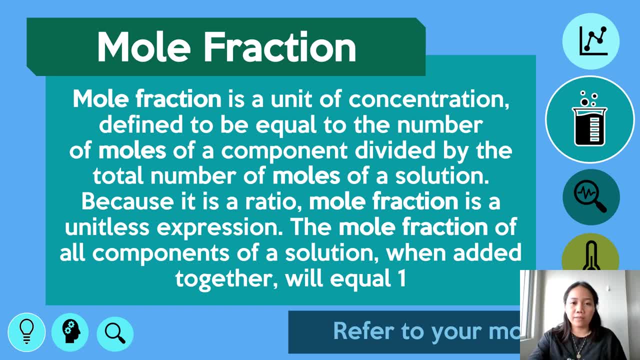 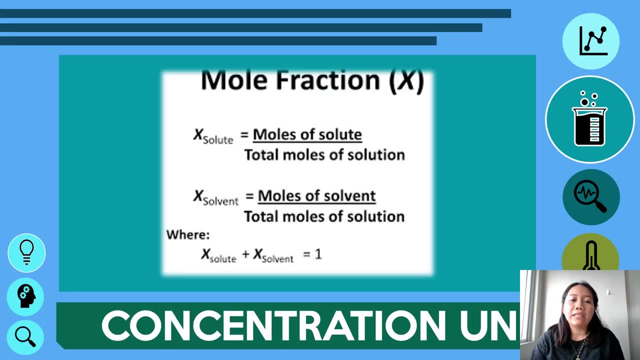 solve some problems regarding mole fractions. the formula for our mole fraction, so we have x by the fraction is denoted as x, so the mole fraction of your solute- in this case you have the moles of your solute divided by the total moles of your solution. so if in the percent by mass and in the 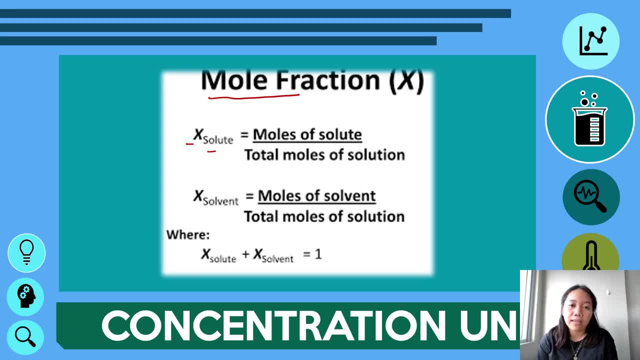 percent by volume. you will be needing the mass and volume respectively, in this case in mole fraction. all you have to do is to look for the number of moles of your solute and your solvent. okay for you to get the total moles of your solution. so again, that would be the case, and then you have to. 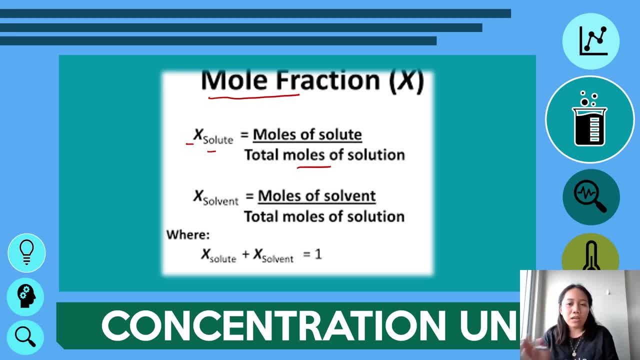 cases for our denominator. So, medyo, they're also similar with the percent by volume and the percent by mass. The only difference is that we're not gonna multiply it by 100, because this is actually fractional, okay. So that's why the total number of our answer should be equal to 1, which is 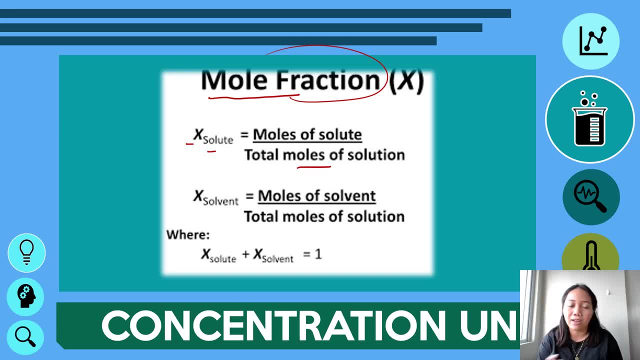 technically 100 in the percentage, okay, But this is not any more percentage. that's why there's no multiplier of 100.. So if your component, if you have two components, which is a solute and a solvent, if we're going to add their mole fraction, it should be equal to 1.. That is the one. 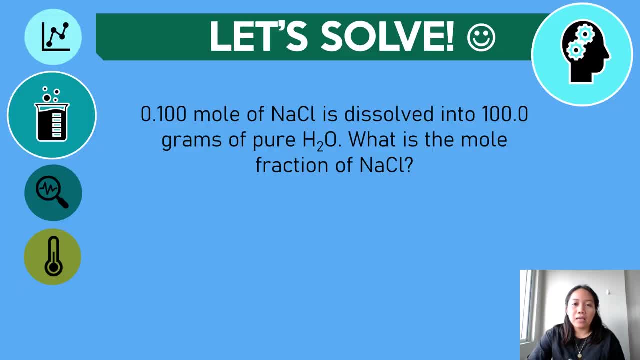 that I was saying a while ago. Now let's try to solve one problem. okay, with regards to mole fraction. So in this case, you have 0.100 mole of sodium chloride that is dissolved into 100 grams of pure water. What is the mole fraction of sodium chloride? okay? So at first, of course, 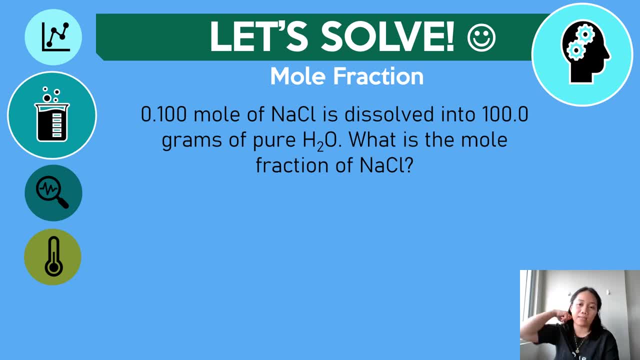 you need to identify what is your solute and what is your solvent in the cases, or what are the different components of the mixture or solutions in the problem. In this case, you have 0.100 mole of sodium chloride. that is the one being dissolved in 100 grams of water. That means your sodium. 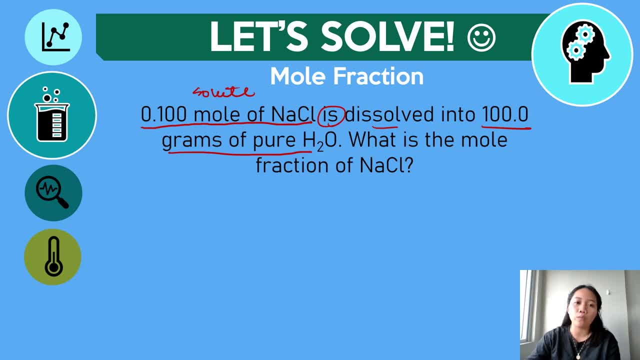 chloride is technically your solute and, of course, your solvent. So you need to identify your water. is your solvent, okay? So, because your sodium chloride is the one that is being dissolved in your water. Now we already know that our solute is sodium chloride and that our 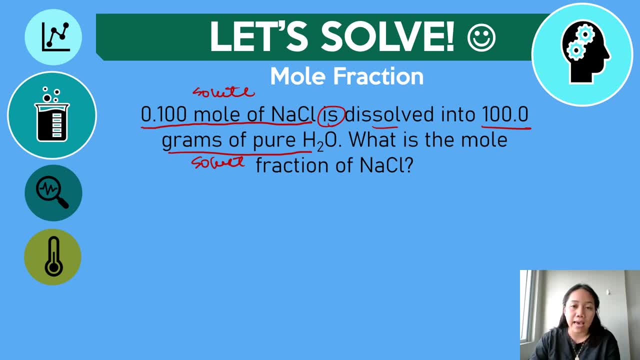 solvent is water. Now let's identify what is the ask problem: What is the mole fraction of NaCl? So the one that is just asked is the mole fraction, or sorry, that's not mole, but rather x. okay, So what is the x? 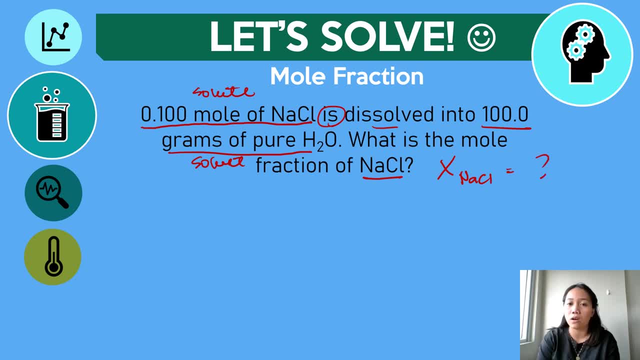 NaCl. okay, That is the mole fraction of NaCl. Now let's solve. Of course, we need to write first the formula. okay, The formula is x: NaCl is equal to the mole of your NaCl all over the mole. 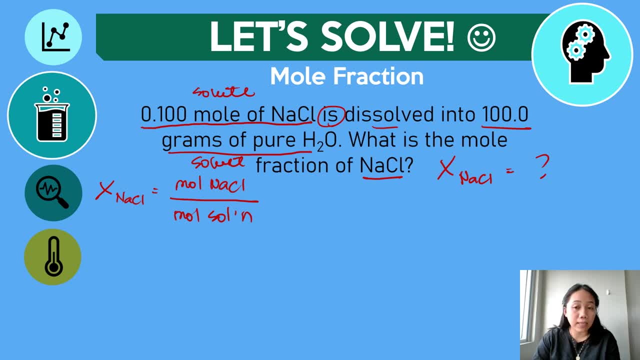 of your solution And, as you can see in the problem, the mole of your NaCl is already given, So we don't have any problem with that at all. Your solution that's a little bit mahirap because it's not in the problem. okay, What is only given? 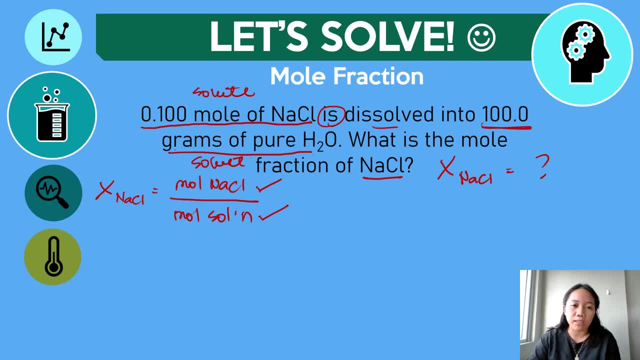 to you is the 100 grams of pure water, which is your solvent. So how are we going to find the mole of your solution? So, given that we have a solvent here, we can now use the value 100 grams of pure solvent, which is water in this case, for us to solve the mole of your solvent. Then, later on, 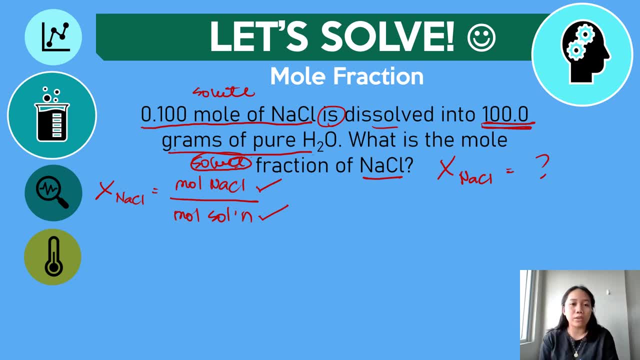 we're going to add now the mole of your solute and the mole of your solvent. So let's solve now for the mole of your solvent. So you have 100.0 grams of water multiplied to. okay, this is just mole. 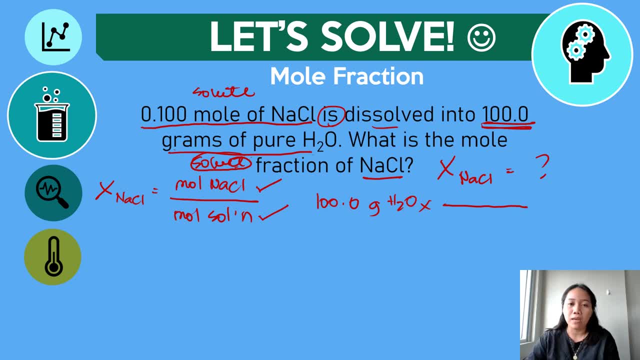 concept because you're changing grams into mole or mole into grams. So simply you put grams below or in the denominator for you to cancel the value And you have in every one mole of water. we know that the molar mass of water is 18.015.. Again, this is the molar mass And I will 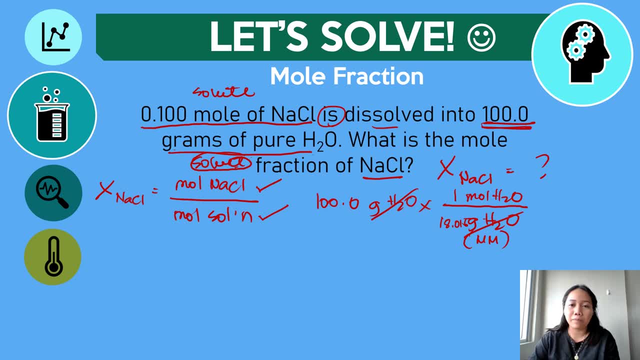 not discuss that one anymore because it will take time. So please review, how are you going to solve for the molar masses? It's just very easy. That's two times the molar mass of your hydrogen, then one times the molar mass of oxygen. I said I'm not going to say it because I already mentioned it Anyway. so you now have the 5.551 grams of water. 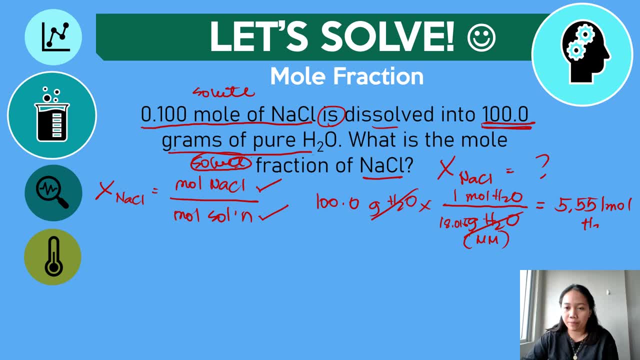 Now take note, guys, This is just the mole of your water. Okay, What we have, or water which is, in this case, is solvent. What we need is actually the mole of your solution. So what are we going to do now? So, since we have, okay, we need to find the mole of your solution. And how are we going to do? 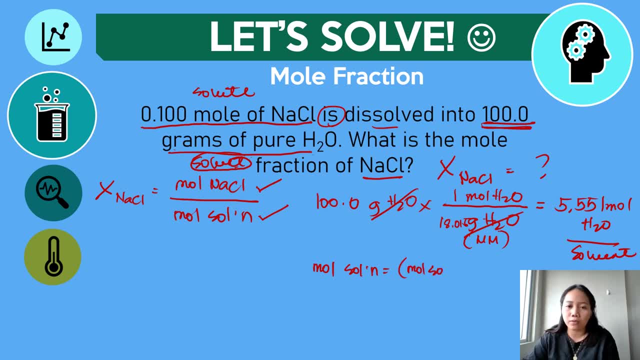 that We need to add now the mole of your solute plus the mole of your solvent. And what is the mole of your solute in this case? You have that in the given, which is 0.100 mole, plus the mole of your solvent, which is the 5.551 mole. 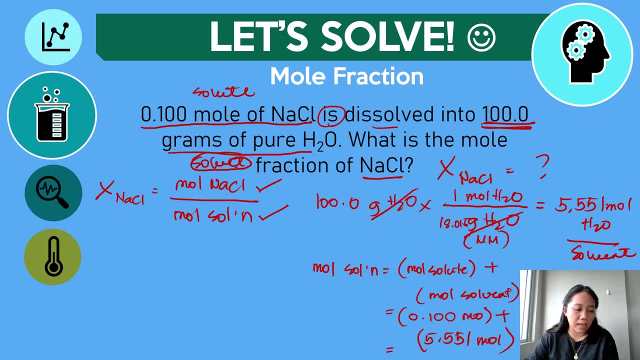 And if you're going to add that one, you will get a value of 5.651 mole. That is now the mole of your solution. Now can we solve for the problem? Yes, because the given or the variables that will be needed in the formula is already given. So the mole of your NaCl, which is in the 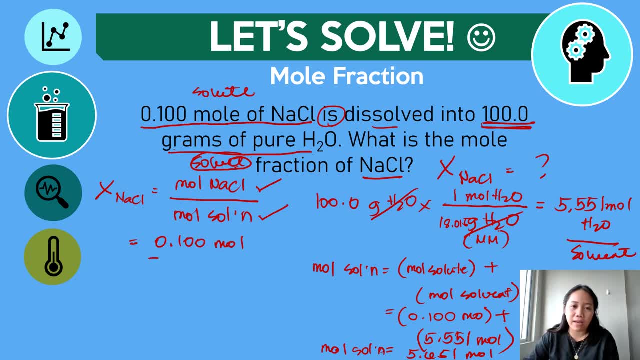 problem: 0.100 mole divided by the mole of your solution, which is in this case, 5.651 mole. Cancel now mole. You now have the value of your NaCl, which is 0.0177, and no unit because that is actually canceled during the process. So you have X NaCl only. 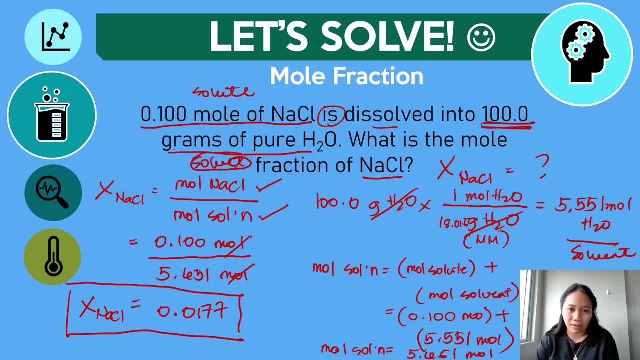 is equal to 0.0177.. Question: why do we have 0.0177 as our answer? Now, because of the value of NaCl, we have 0.0177.. So we have 0.0177 as our answer. 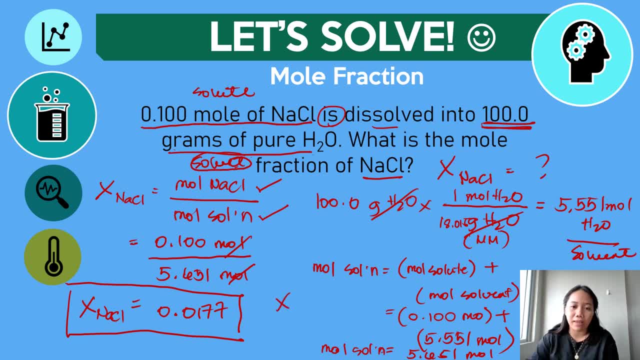 Now, because of the value of NaCl, we have 0.0177 as our answer. So we have 0.0177 as our answer Because in the process of solving this one, it involves multiplication or division. we need to follow now the proper ruling of significant figures. Go back to the problem. 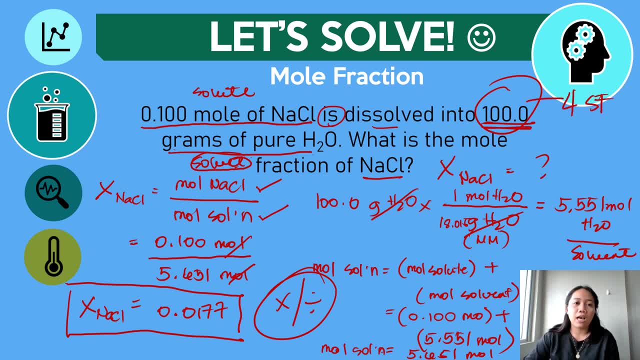 how many SF do we have here? It's 4 significant figure. How many SF do we have here? It is 3 significant figure. And because we are following multiplication and division ruling of significant figures, or, yeah, the ruling with the significant figures we need to follow. 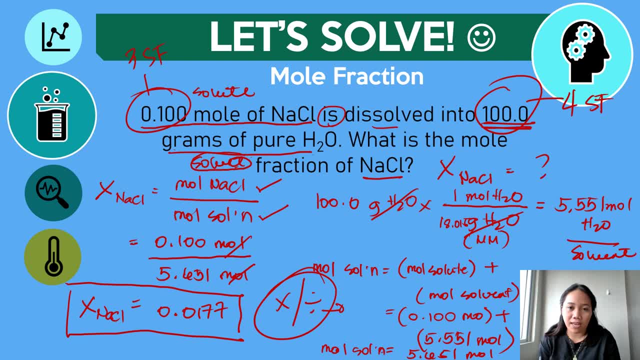 the least significant figure in the given. And because the least significant figure is three, then that means our answer should contain three significant figures as well. So that's why our answer is 0.0177.. Those two zeros that are before a non-zero number is not significant. 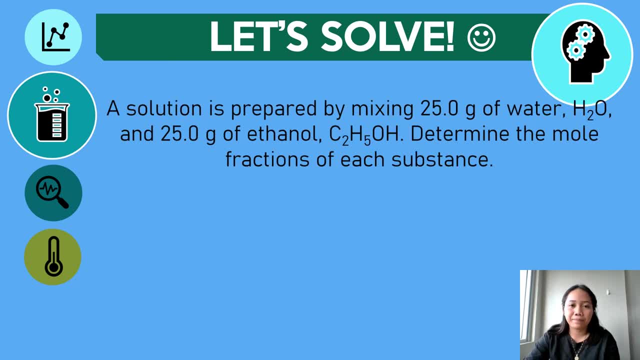 So that is the first problem. Next, let's proceed to another problem, which is a solution is prepared by mixing 25 grams of water and 25 grams of ethanol. Determine the mole fractions of each substances. So in this case we need two. The unknown is the two mole fraction, So x water and the x ethanol. 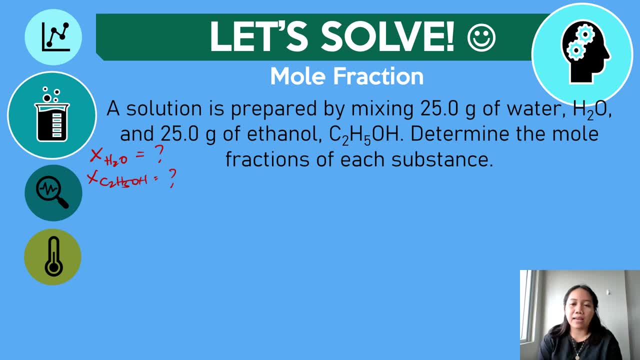 See, That is the unknown. Now let's identify what are the components. Of course we have now 25 grams of water and we have 25 grams of ethanol. So let's solve for the number of moles, Because of course this is mole fraction. we need the number of moles And since the given in our problem, 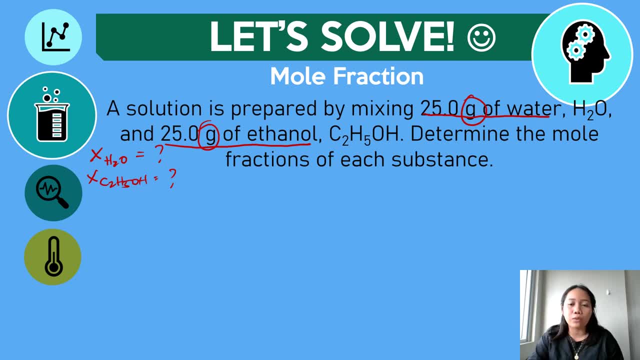 are not in moles but in grams. all we have to do is to follow the mole concept and change your grams into mole. So you have now 25.0 grams of water. x 2 in every 1 mole of water, you have 18.015 grams. 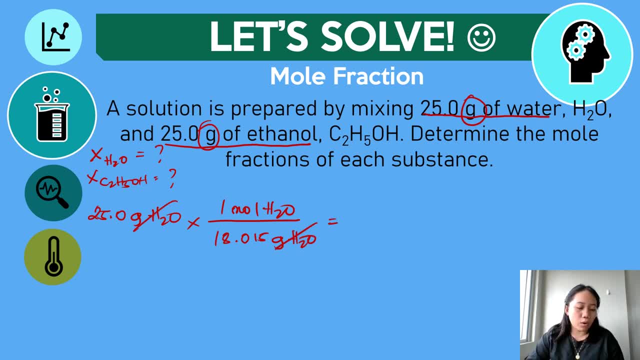 of H2O. So you cancel the grams. Your mole fraction of the water is 5.551 mole of water. How about your ethanol? So your ethanol is 25.0 grams of H2O, So your ethanol is 25.0. 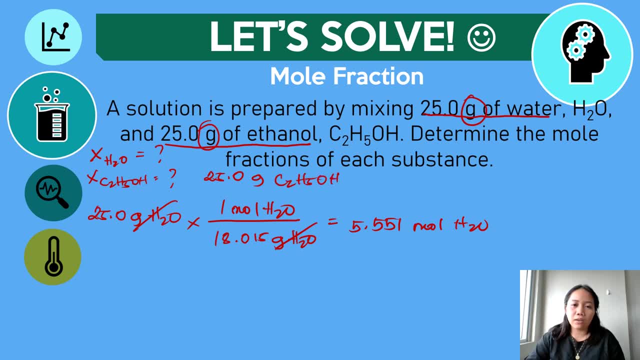 grams of C2H5OH And of course you need to multiply it by 1 mole of C2H5OH. And what is the molar mass of your C2H5OH? That would be 46.069 grams of C2H5OH. Now you cancel grams. 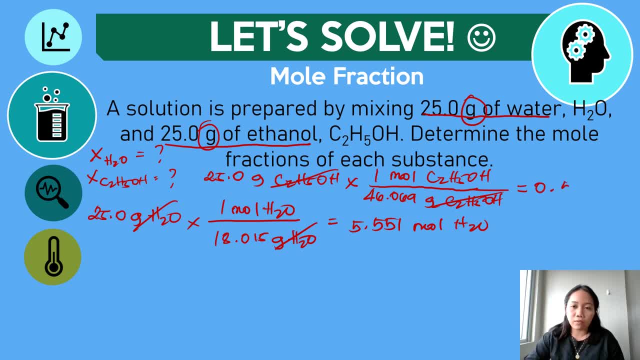 then you will get an answer of 0.543. mole of C2H5OH. Now we have 2 moles, as you can see: the ethanol and the water. So we need to add these 2 values for us to get the mole of our solution. So the mole of our solution is equal to 0.543. 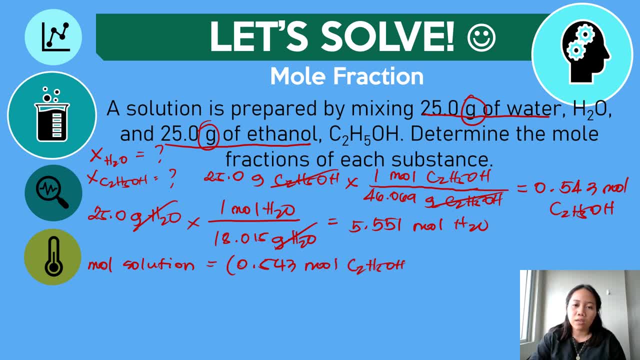 mole of your C2H5OH plus the 5.551 mole of your water, And that will give you 66.069 grams of C2H5OH. So that's it. Thank you for watching. See you in the next video. Bye. 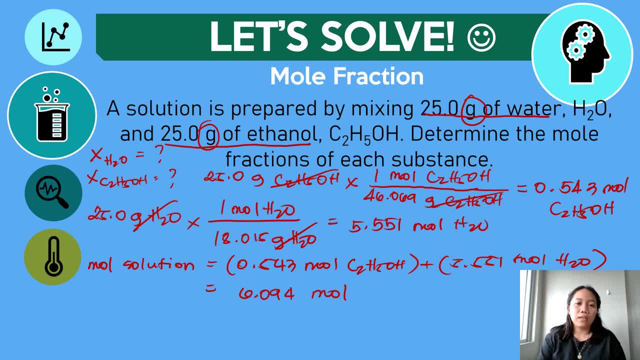 6.094 mole. Okay, so we now have the total number of moles. okay, of your solution. And what is the unknown? Determine the mole fractions of each substances. We need to solve for the x of water and for the x of your ethanol. So x sub water is equal to what is the mole? 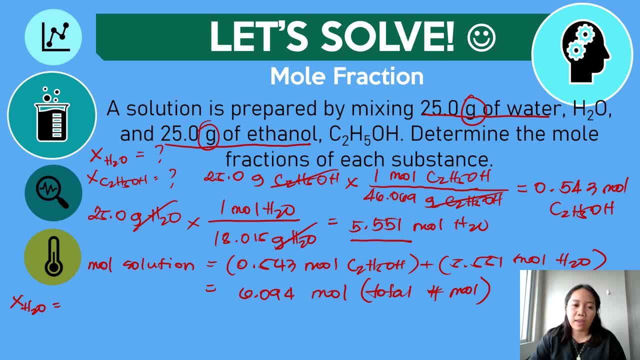 of your water. Just go back here. You have 5.551.. 5.551 mole divided by the total number of moles, which is 6.094 mole. All you have to do is to cancel the mole. then you will get the x of your water, which is 0.911.. I express my answer into: 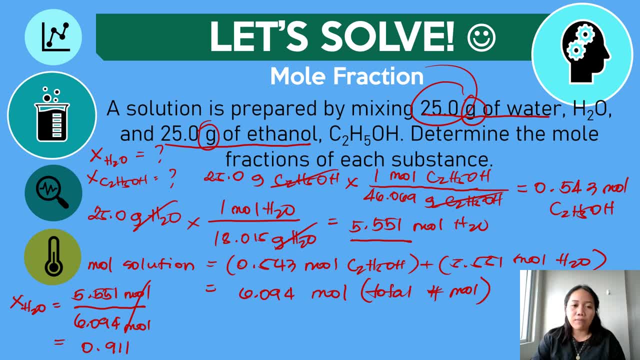 3 significant figures, because in your given you have 3 significant figures, which is the least significant figure. So you have 0.543 mole divided by 6.094 mole. So cancel now the mole and you will get a value of 0.0891. 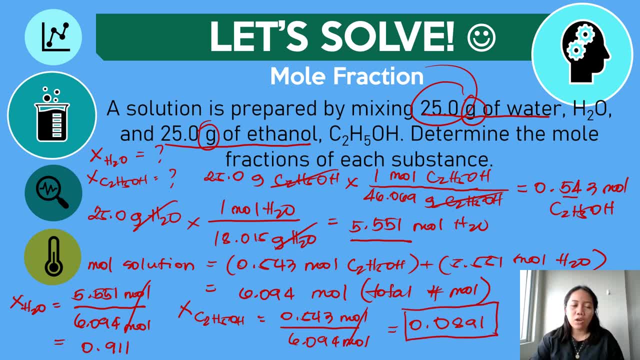 This is now the mole fraction Of your ethanol. this is the mole fraction of your water. To check if your answer is correct, add the two values and if it's equal to 1, then your answer is correct. That is how are you going to solve this problem involving mole fraction? 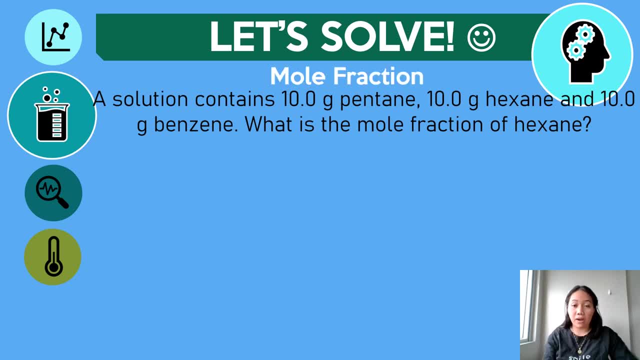 Okay, now we have another problem involving mole fraction. So, as you can see in the previous slide, we have a solution of mole fraction, of every solution or in every mixture, But in this case, in this kind of problem, we have three, namely 10 grams of pentane. Okay, we have it here. 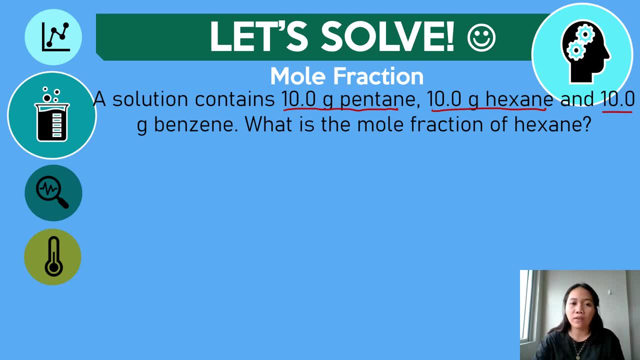 We have 10 grams of hexane and the 10 grams of benzene. So the only question in this problem is actually: what is the mole fraction of your hexane? Okay, we are only looking for one number of mole fraction in the three components. However, 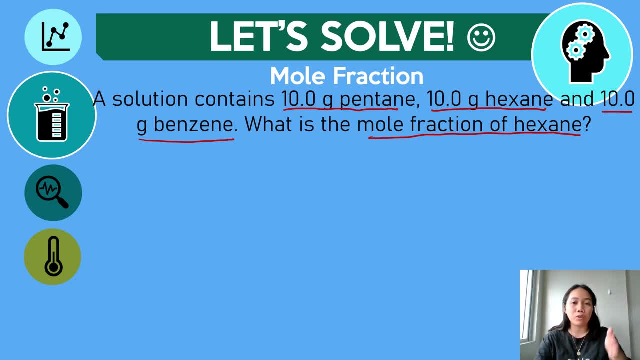 important to identify the different number of moles of every component, because we will be needing the total number of moles in your denominator, in the formula of mole fraction. So, since the given is all in grams, we need to identify the different number of moles of every component. Now let's 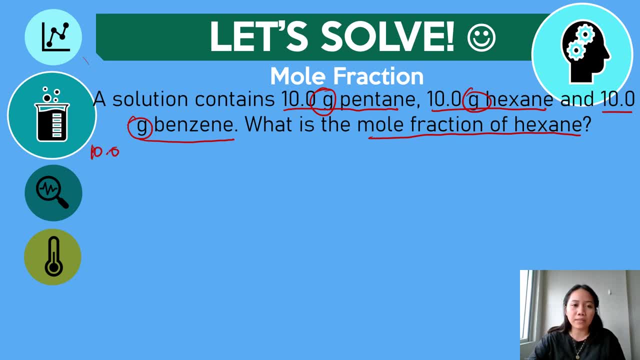 start with the pentane. So 10.0 grams of pentane, which is C5H12.. Okay, remember, in your mole concept, if we're going to change grams into mole and or mole into grams, you will be needing your what we call molar mass. So in this case I'm not going to discuss to you anymore. how did I solve? 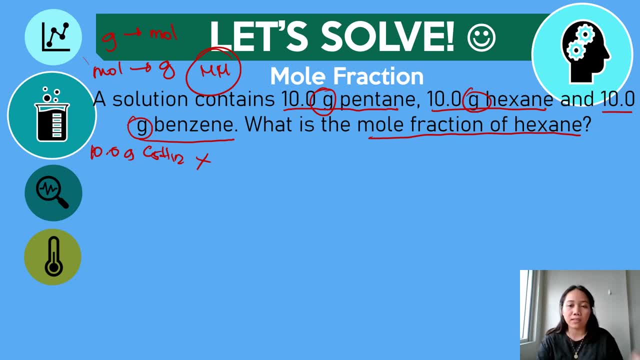 for the molar mass. All you have to do is take a pause in this video, then you can solve for the molar mass Of the pentane. okay, if you want, then you can just go back to the video itself. So here. so since 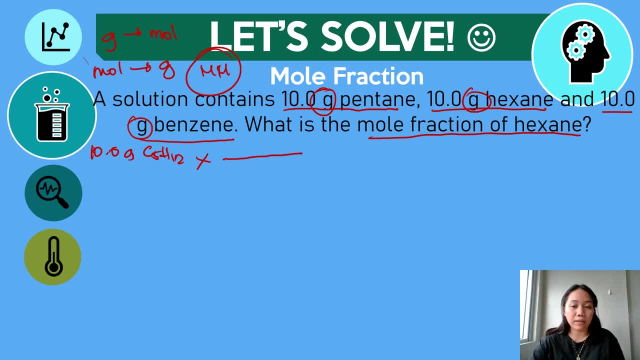 your grams is in the numerator part of this given. so you need to have your grams dito sa kabila in the denominator for you to be able to cancel the grams. So C5H12.. So cancel now grams, So in every one mole of your C5H12, solve for the molar mass. 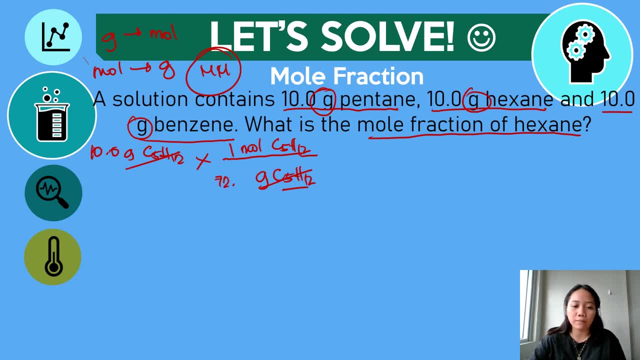 of your C5H12.. In this case it's 72.151 and that would be equal to 0.1386 number of mole of C5H12.. Next, the 10.0 gram of hexane, C6H14, times In one mole of your C6H14, you get a number of 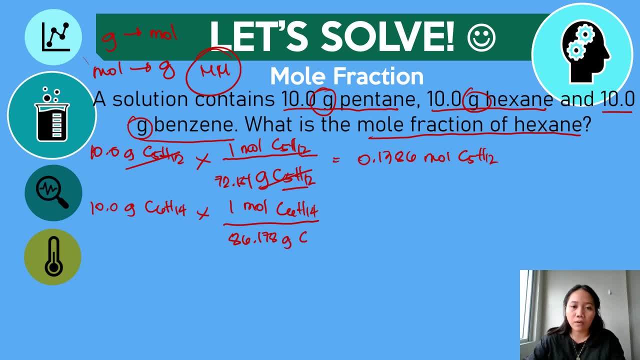 grams, which is 86.178 grams of C6H14.. Then you cancel grams, then you will get the value of 0.1160 mole of your C6H14.. Let's now have benzene. So 10.0 grams of benzene- C6H6 times- in every one mole. 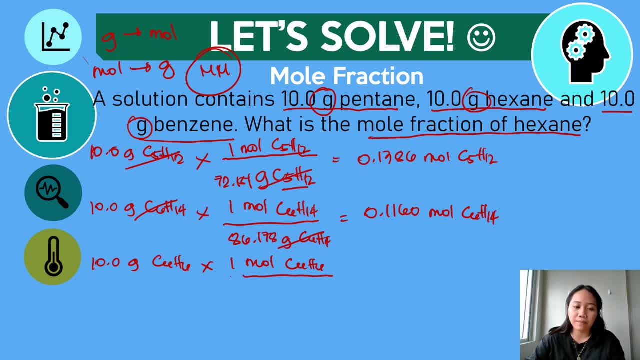 of C6H6 divided by 78.114 grams of C6H14.. So that would be equal to 0.1160 mole of your C6H14.. Next, general to the know, Gs which let us know, the regular Gs, Take Y. 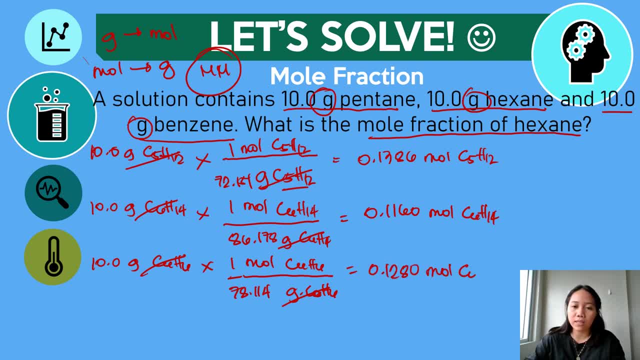 So, Angel, my friends, time out, Again, times out, And again minus C6H4 times N, And essentially this is what I went through here and what we got here. So at that time, whereração, little by little, by going through those numbers, what we got is that 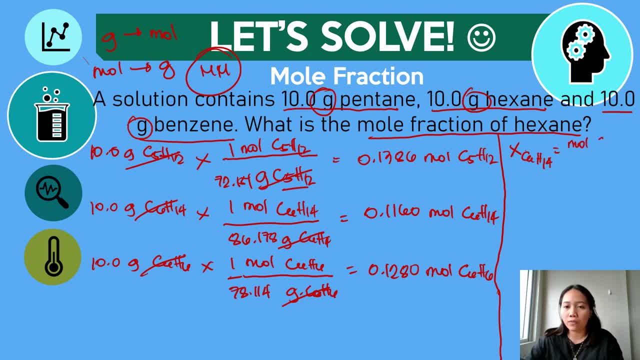 next ingredient that is coming. are you gonna put this? There we go: mole of your C6H14 divided by the total number of moles of your solution, But yet we still don't have the total number of mole. Okay, So what we need to do is to add everything, every number of. 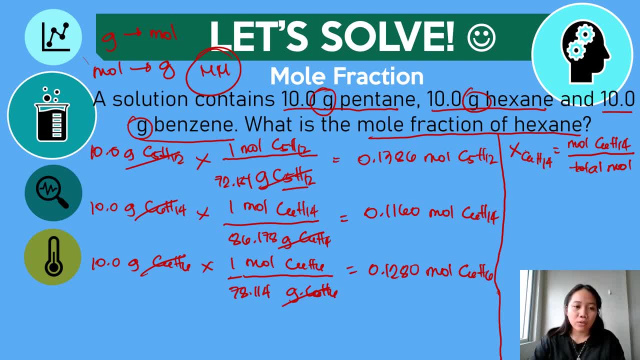 moles of the three components of this mixture. So you have mole of your solution is equal to 0.1386 mole of C5H12 plus 0.1160 mole of your C6H14, plus you have 0.1280. 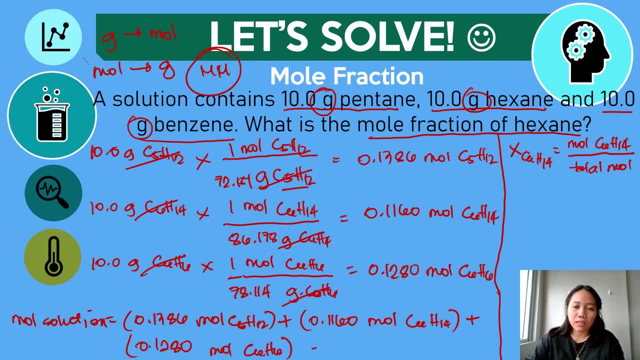 mole of your C6H6.. Then you will get an answer or a total of 0.3826 mole of your solution. So we need to do that. So now let's see what we do. So we need to do this. So we need to do this. 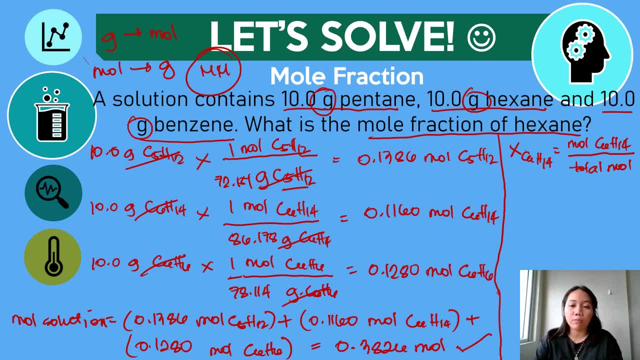 and then we need to do this. So let's see what we do, And then we need to do that. So we need to do: now: have the number of moles of your solution and we also have the number of mole of your hexane. 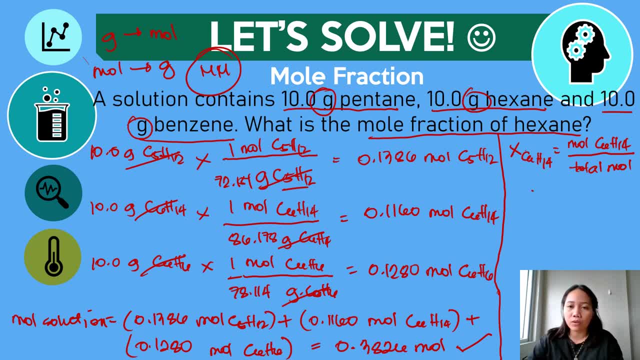 So all we need to do now is to solve for the mole fraction. So mole fraction of your hexane is equal to the mole of your hexane, which is 0.1160 mole divided by the total number of mole, which is 0.3826. 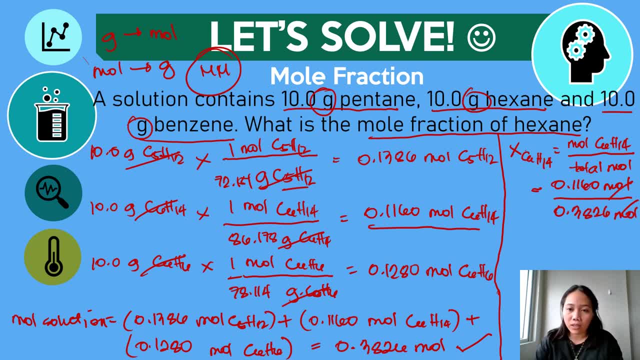 mole. All you have to do is to cancel the mole and now you will get the value of your mole fraction of hexane, which is 0.303.. Now, if you're going to take a look at the answer, it should contain three significant figure because, based on the given, all of our given contain three significant 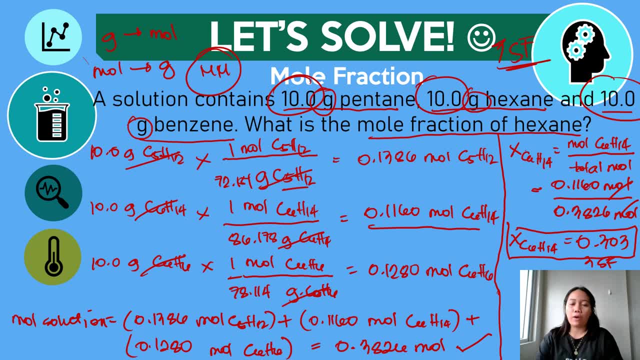 figures and we need to follow the proper significant figures in the final answer that we have. So that's it. That's: how are you going to solve for the different mole fraction Now? we're done with the percent by mass, the percent by volume and the mole fraction Now. 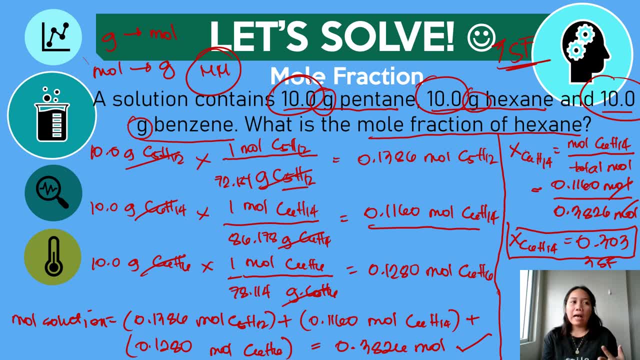 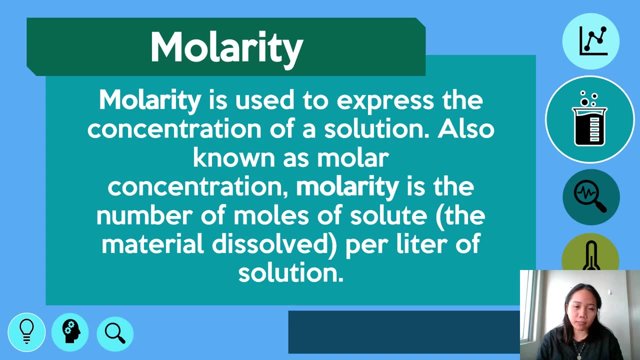 let's proceed to the most familiar unit of concentration in chemistry, which is the molarity molality, ppm and the ppb Molarity. we know that molarity is another used expression for the concentration of units and it is denoted as capital letter M and its unit will be mole per liter because its 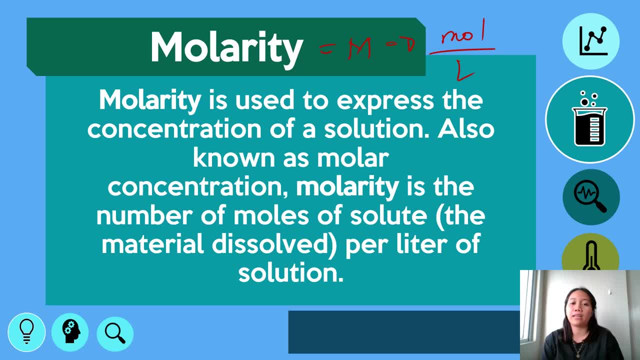 formula is actually the mole of your solute divided by the liter of your solution. That's why you come up with a unit mole per liter. Now, molarity is also known as the molar concentration. That's why, if you're going to have a value which is 0.6 Tm, okay, we call it 0.6. 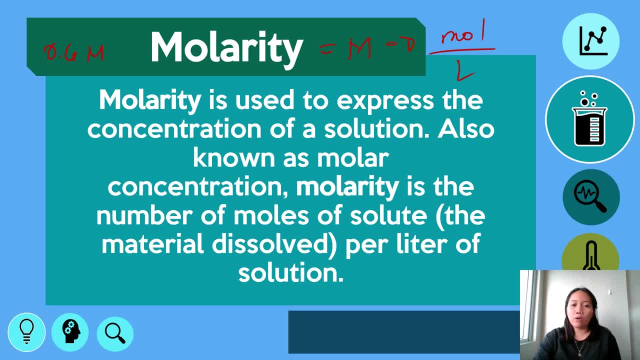 molar. okay, with an R. Now, please don't forget to refer to your module with regards to this topic, because there are also a lot of explanations with regards to molarity there, and as well as examples. But in this pre-recorded video, let's discuss five- or no, sorry, six- different problems involving 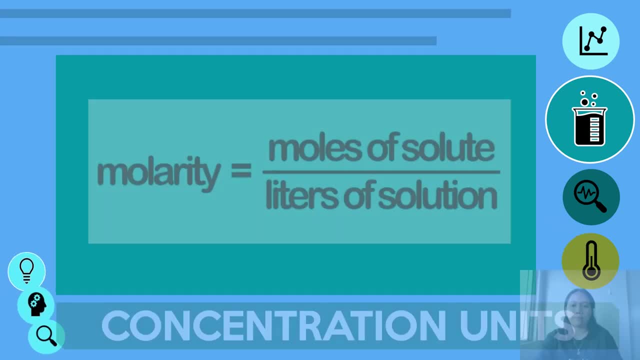 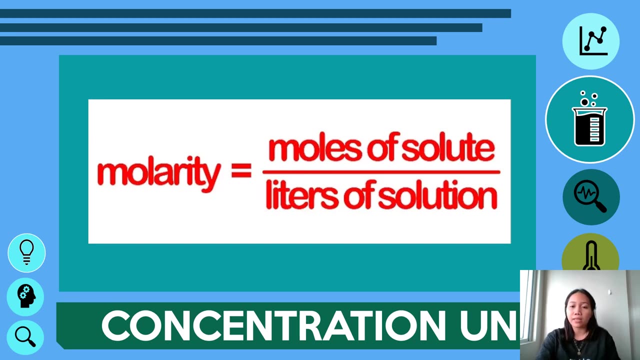 molarity. Let's start with the easy one, Of course. the formula for your Formularity is simply the moles of your solute divided by the liters of your solution. Again, it is very important to know that a solute added to a certain solvent will give you a solution. 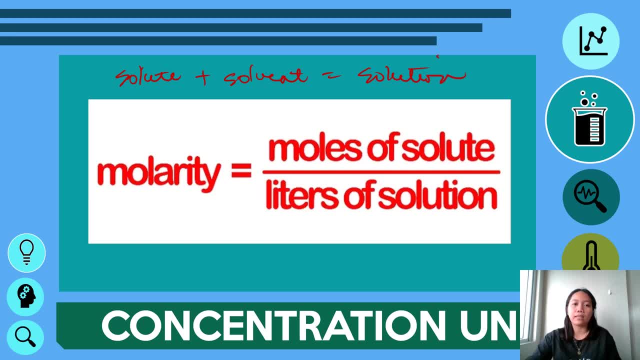 Okay, Regardless of what particular amount is that? it may be in grams or any unit involving mass. It may be in ml or liters, Okay, Or any unit of volume, Okay, You will come up with the number of solution. So, in this case, because you have here liters of solution and not all problems are giving you the value of the liters of solution in the problem itself, 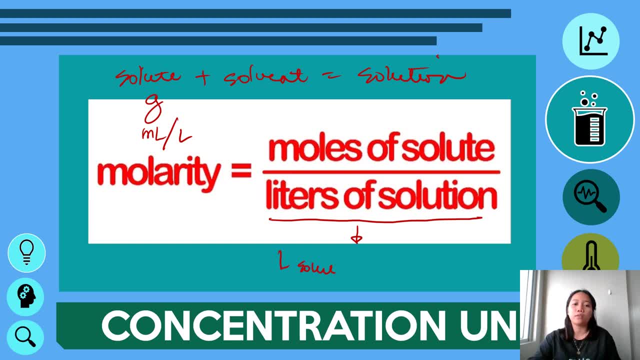 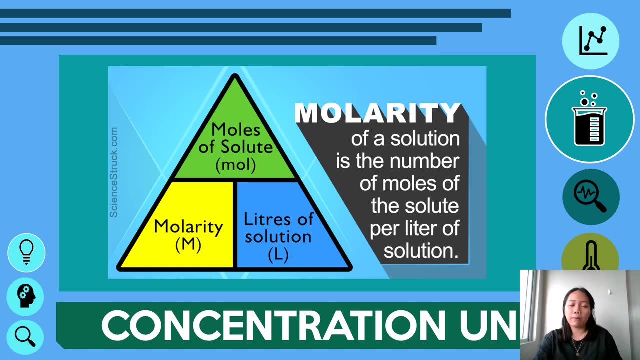 then please don't forget to look for the liters of your solute and the liters of your solvent. Add them, Then you will get the liters of your solution. Now let's proceed to one example problem. Okay Now, by the way, this is another way of actually solving formularity. 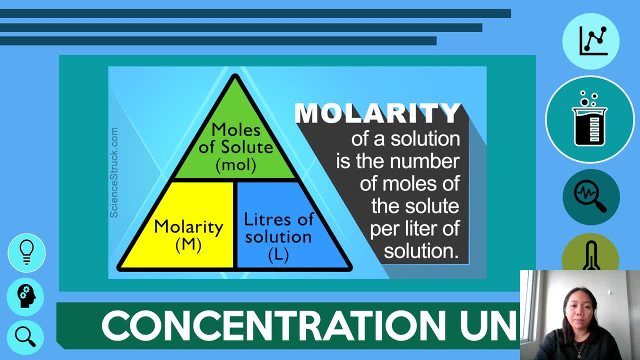 The using of the triangular formula, wherein you could actually derive any other variables that will be unknown in some problems. Say, for example, if the case is, the unknown is the number of moles of your solute, all you have to do is to multiply your molarity to the liters of solution. 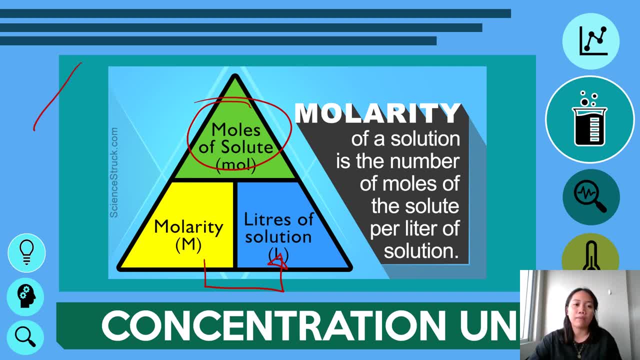 Then you will get the mole of your solute. It's actually the same with the one, that is with density. It's density, mass over volume. Okay, If you're going to solve for the mass, all you have to do is to multiply density and volume. 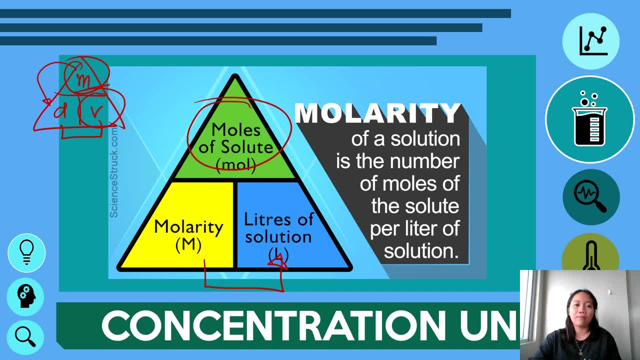 If the unknown is volume, all you have to do is to have mass divided by the density for you to get the volume, And so on and so forth. So the importance of this triangular formula is that you could actually derive without deriving the formula itself. 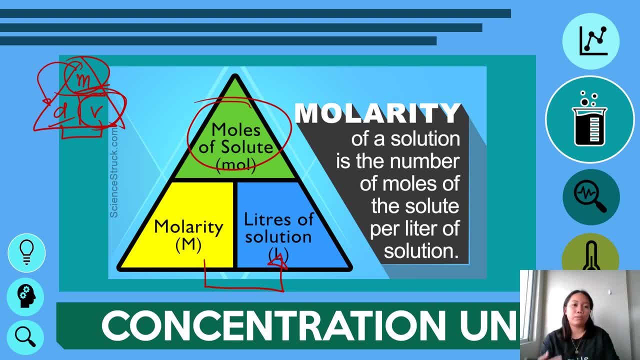 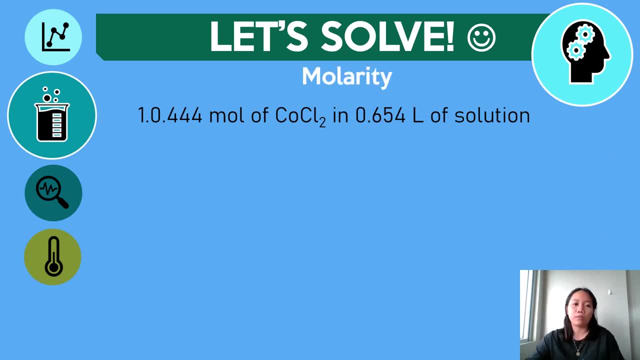 Because it is already written And it is readily available in those triangles. Now let's start solving different formularity problems, Starting with this one. This is actually just quite easy. If we have the synchronous discussion already, we have this problem, or we have this particular example already. 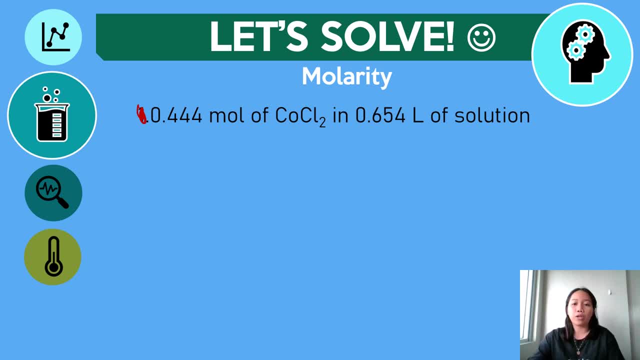 So you have 0.444 mole of your cobalt chloride and 0.654 liter of solution. Of course, the last question there is: what is the formularity? So the formularity, Of course, the formula is: M is equal to the moles of your solute divided by the liters of your solution. 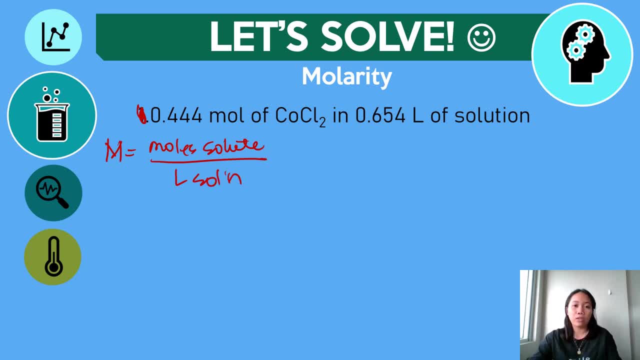 If you're going to take a look at the value that you have in your problem, you have 0.444 mole of your cobalt chloride And you already have the liters of your solution. So all you have to do is to actually substitute all the values. 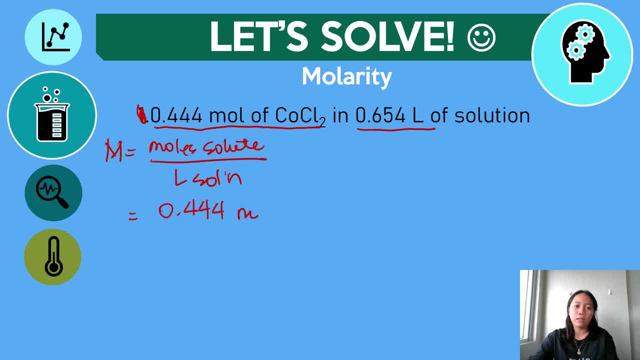 And you will get 0.444 mole over 0.654 liters And in that case, if you're going to divide those values, you will get 0.679 molar. Okay, So you could also write it in a way that you can see the formula. 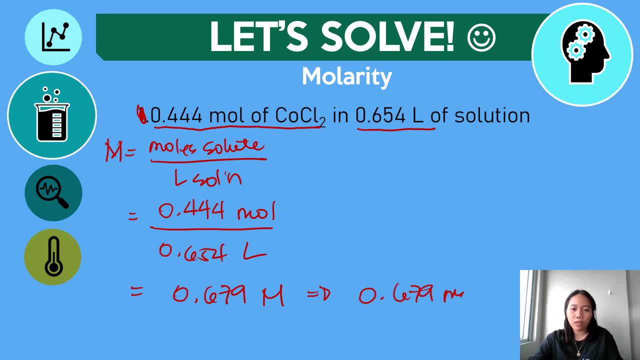 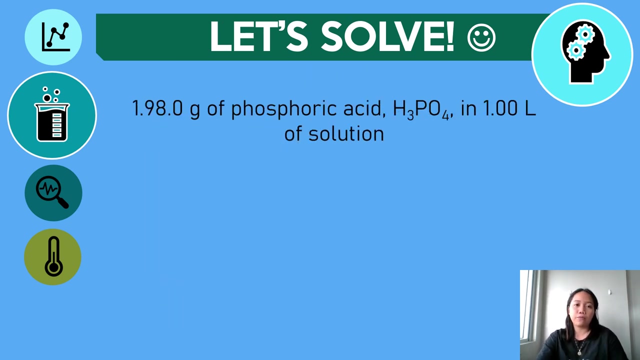 So that would be 0.679 mole per liter. Okay, There are two ways of writing the answer: 1., 2., 3., 4.. Let's now have another formula, or another problem rather, So in this case it's not quite easy as the one that we have a while ago. 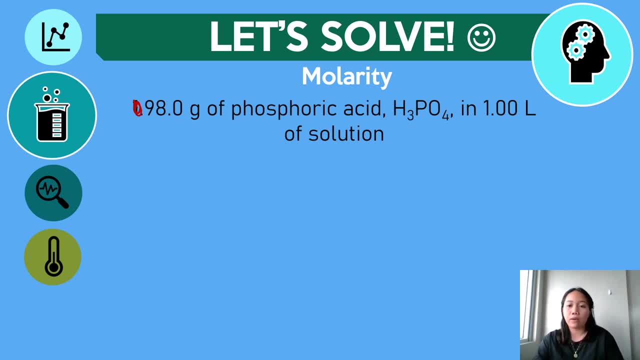 Because in this case the mole is not directly given to everyone. okay, The given is only the mass of your solute, which is 98 grams of phosphoric acid and you have one liter of solution. And because we don't have 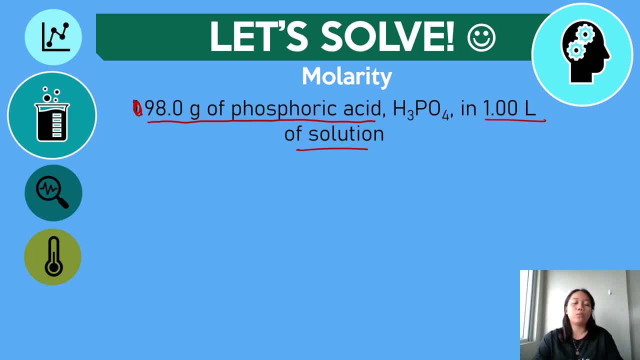 the moles of your solute. we need to do a mole concept or we need to have the mole concept wherein you are going to change a grams into mole or mole into grams by using the molar mass of the particular compound for you to get the unknown. So in this case, we know that molarity is equal. 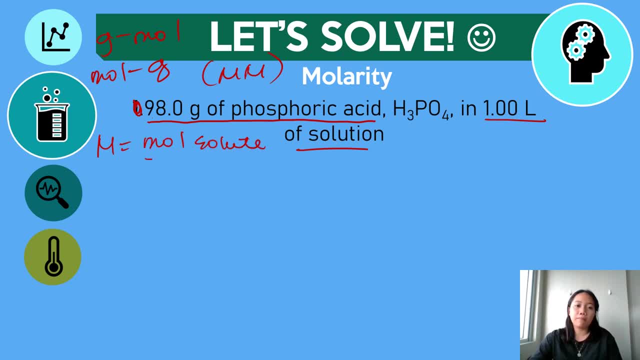 to the mole of your solute divided by the liters of your solution, And because you have 98.0 grams of phosphoric acid, all you have to do is to find the molar mass of your phosphoric acid and do the mole concept. 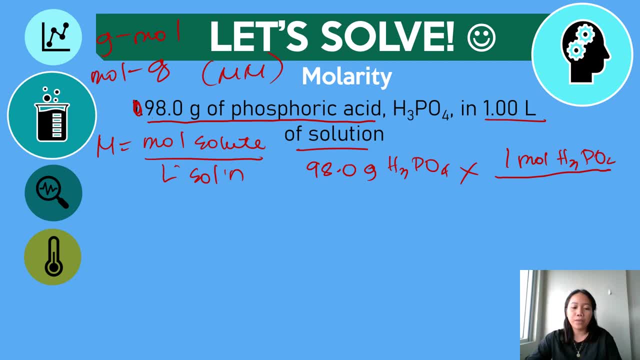 So in every one mole of your phosphoric acid you have 97.994 grams of phosphoric acid. This is its molar mass. So please pause this video and solve for the molar mass of the phosphoric acid. kung medyo nabibilisan kayo at hindi nyo alam kung paano nakuha yan. 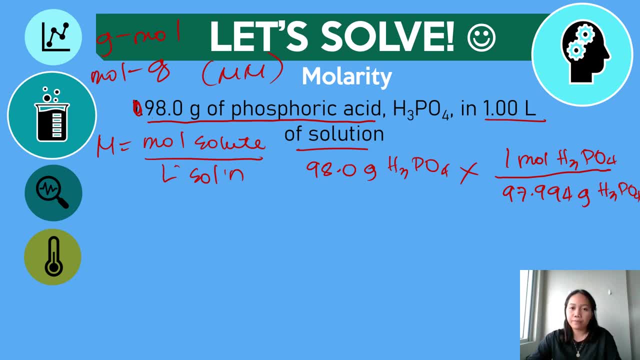 Recall your chemistry. 1. Cancel now grams. okay, Then you will get now the value of your mole of phosphoric acid, Which is, in this case, 1.00 mole of phosphoric acid. Now, it's not the end of our solving process. 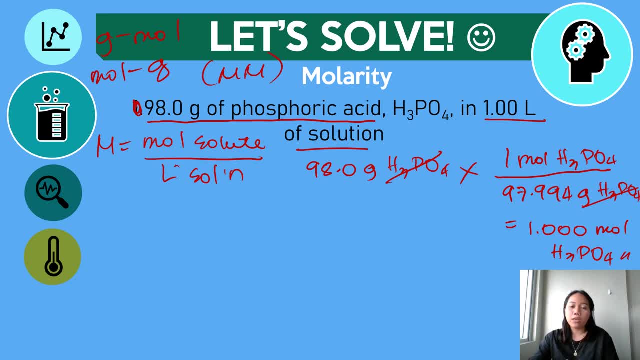 because what we just did is to find the mole of your solute. So we need to identify now the molarity of the solution, Since the solution is only one liter. so all we have to do is to write the mole of your solute, which is 1.00 mole divided by the one liter of solution, and you will. 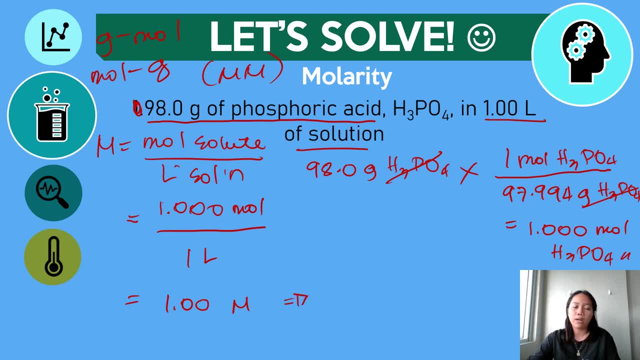 come up with a 1.00 molar solution or 1.00 mole per liter. And why did I have 1.00 as an answer? Because you need to have three significant figures here, because, going back to the given in the problem, you have three significant figures as well. So that would be for the second example. 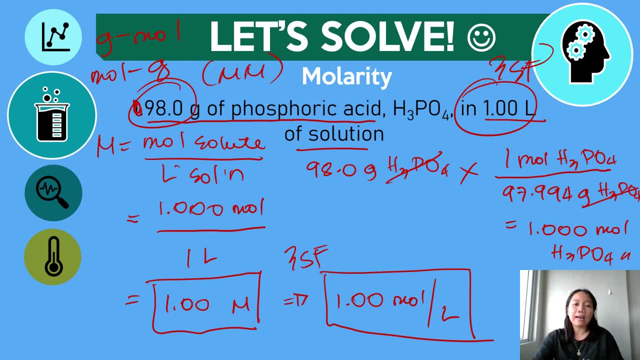 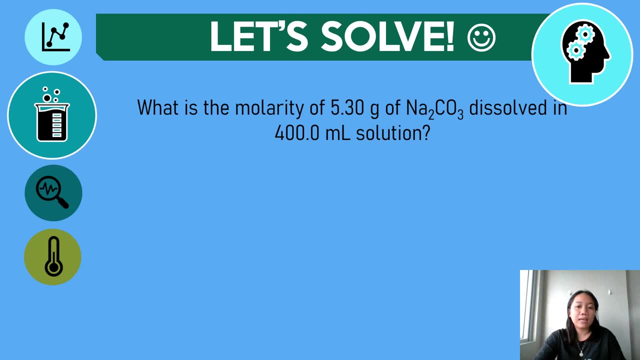 under molarity. Now let's have another example. Now let's have another example under molarity, wherein the given is not in liters. The given is in mL. So of course that would need a conversion unit or a conversion factor for you to be able to know what is the liters of the solution. 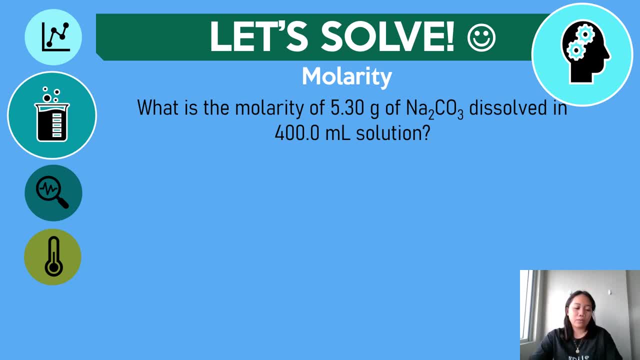 As well as the mole of your solute. it is also not given, because the given is only the mass of your particular compound, Which is in this case sodium carbonate. So write down first the formula for you to identify. So write down first the formula for you to identify. 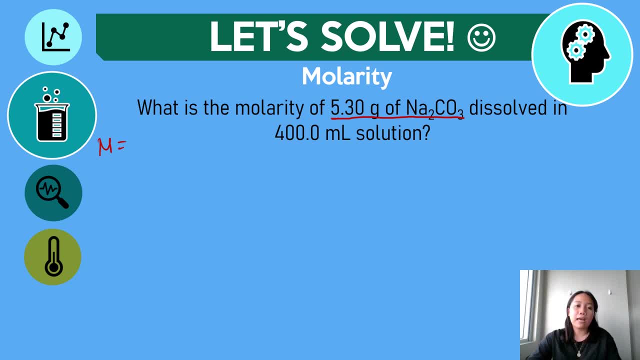 what are the variables that you will be needing? So, molarity: you have mole of your solute divided by the liters of your solution. And what is the mole of your solute? Again, it's not given. Do you have the liters of your solution? No, it's not given as well, So we need to identify them. 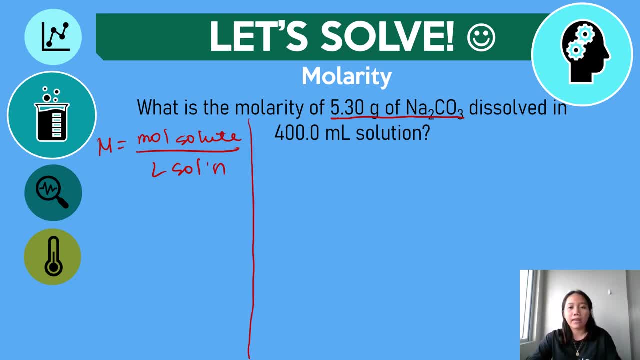 individually. So what particular value are we going to use here? Since we have 400 ml of solution, we know that it's for the solution, so we're not going to use that for the mole of your solute. You have 5.30 grams of sodium carbonate dissolved in, meaning sodium carbonate is the one that is. 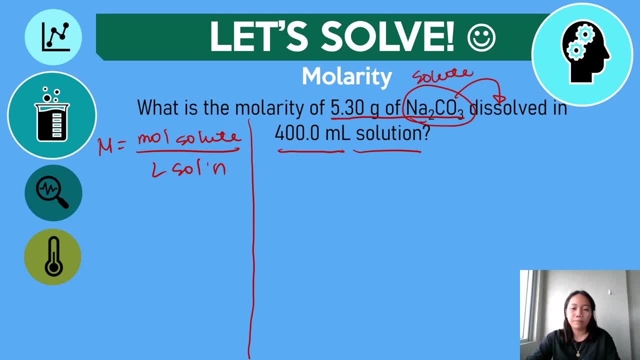 being dissolved. That means this will become your solute And since that is your solute, you will now have 5.30 grams of your sodium carbonate. Okay, and you're going to use the concept again for you to be able to convert your grams into the number of. 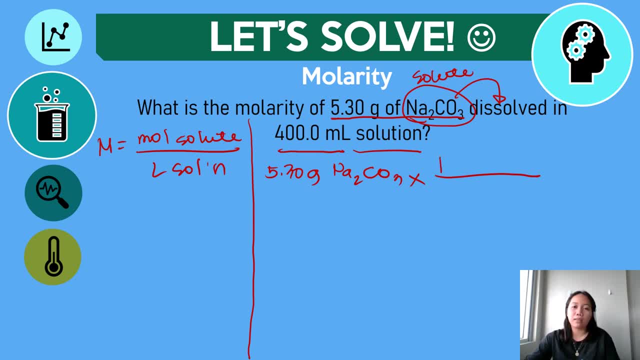 moles. So find the molar mass of your sodium carbonate. In every one mole of your sodium carbonate you will get 105.988 grams of sodium carbonate. Now you cancel grams and you will now have the number of moles, which is in this case, 0.0500 mole of sodium carbonate. Of course, 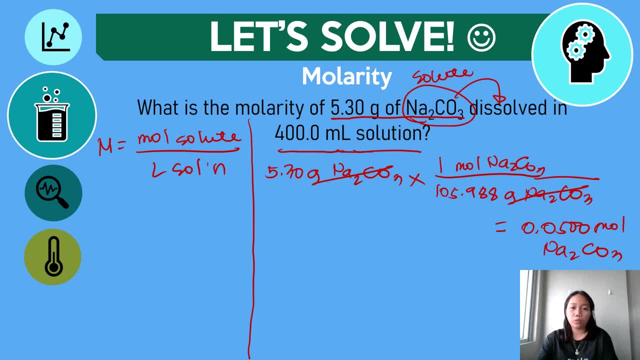 since the given solution or volume of your solution is actually in ml, still need, or you need, to convert your ml into liters muna. So you have 400.0 ml of solution multiplied to. since your ml is in the upper side, you need to have it in the denominator of your 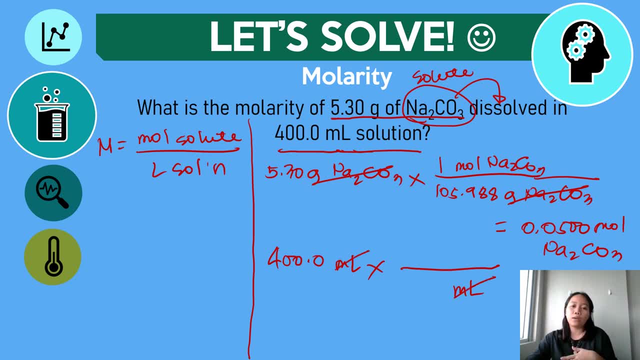 conversion unit for you to cancel the ml. And of course in every one liter you have 1000 ml And if you're going to divide that one you'll get a value of 0.400 liters. Now can we solve for the? 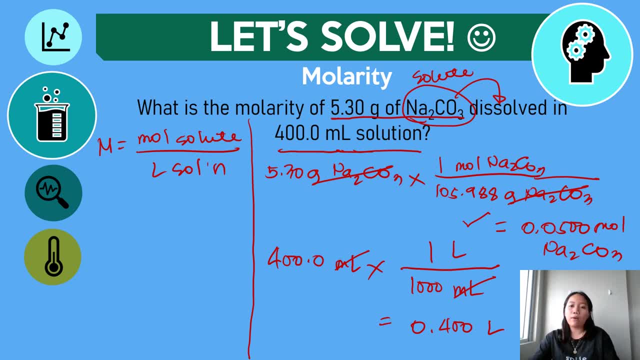 solution. Yes, because we now have the number of moles of your solute as well as the liters of your solution. So the mole of your solute is 0.0500 mol divided by the liters of solution, which is 0.400. 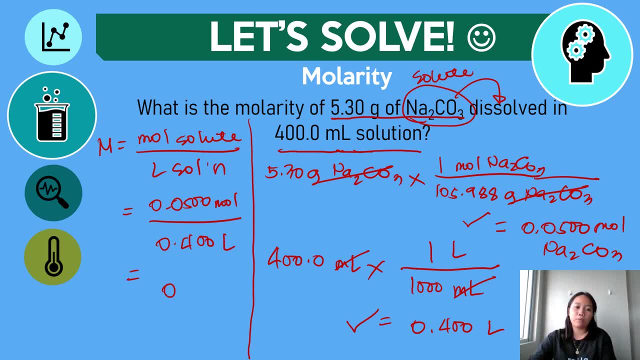 liters and you will get a value of 0.125 molar Box. your final answer: Check for the significant figure. It contains three significant figures. Go back to the problem. the least significant figure is 3. significant figures as well. 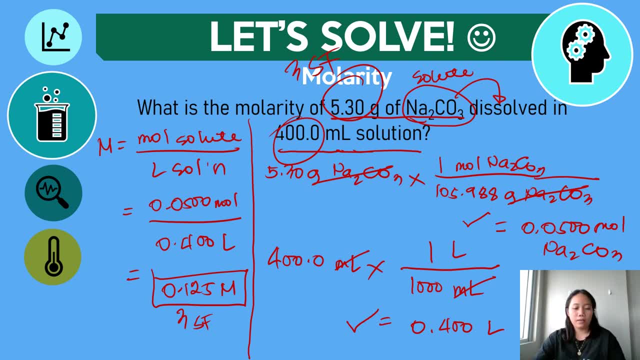 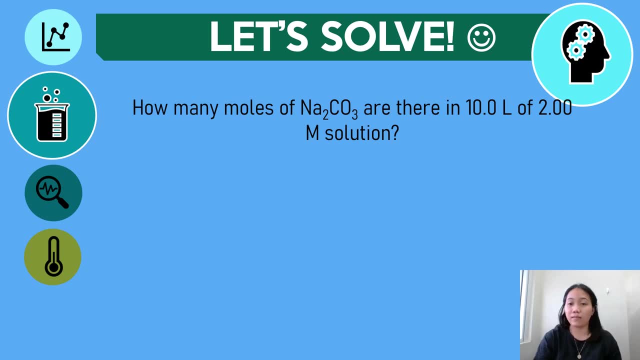 So your answer now is correct. Okay, let's have another example with a molarity, with molarity as one of our concentration units. So we have here: how many moles of sodium carbonate are there in 10.0 liters of 2.00 molar solution? 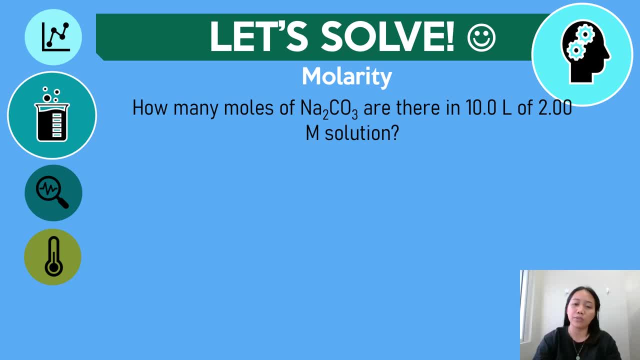 Now, in this case, I have mentioned this one in the previous slides, wherein I told you that, in molarity, it's not always the molarity that is unknown. It could be also the other variables that are involved in the solution, which is, in this case, the number of moles. 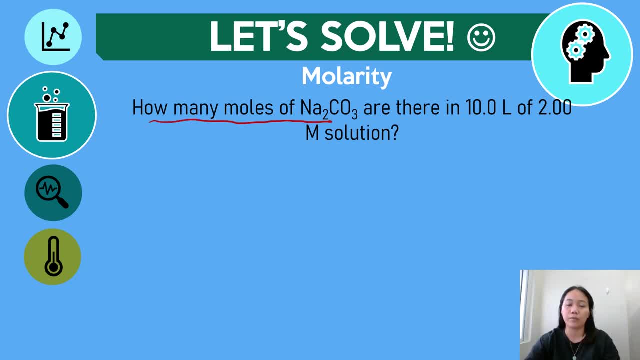 Okay, you are asked how many moles of sodium carbonate are actually in a 10.0 liter of 2.0 molar. So, as you can see, the molarity is already given and the volume of the solution is also given. 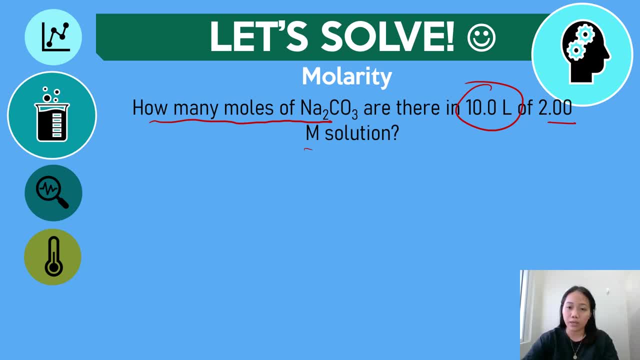 Now the asked question is: how many moles of sodium carbonate? So all we have to do is to derive our formula. Since our formula is, molarity is equal to the mole of your solute, and that would be divided by liters of solution. 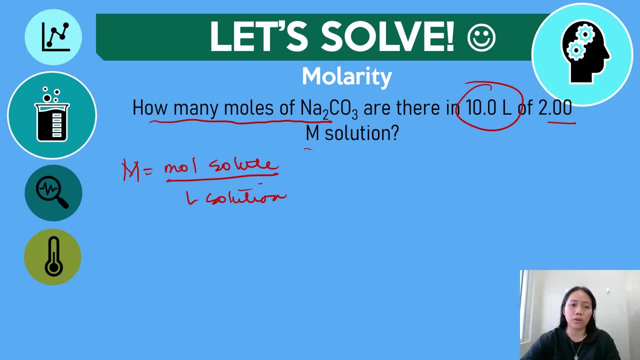 then all you have to do is to cross, multiply, because you have the mole of your solution and then you have the mole of your solute, as the unknown is equal to the molarity times the liter of your solution. Now, if you're going to recall your mole of solute, or, sorry, the molarity, okay, the unit for your molarity is actually mole over liter. 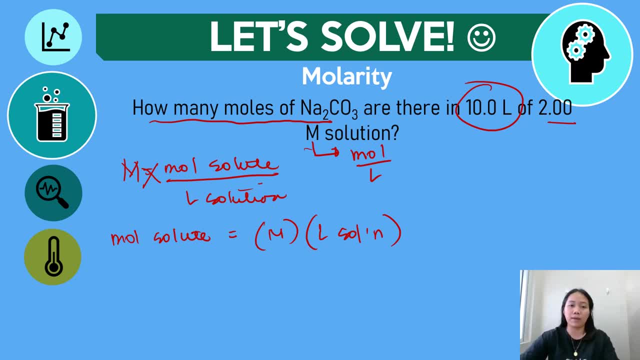 because that is the formula: the mole of solute divided by liters of solution. So that would be the unit that we are going to use here in the molarity for us to be able to cancel out the liter solution and for us to be able to cancel out the liter solution. 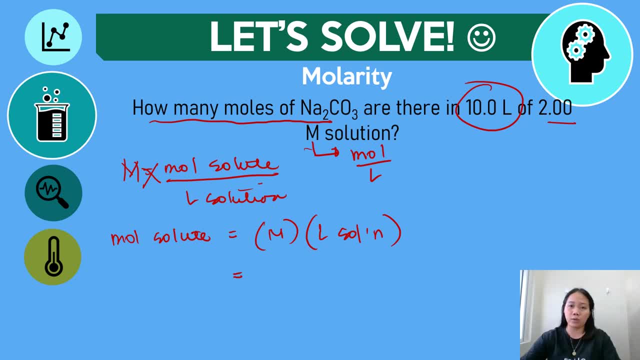 And for the mole of your solute to stay, because that is the unknown. So you have 2.00 mole all over liters times. you have the liter of solution, which is 10.0 liters. so cancel out liters, then you'll get 20.0 liters, I'm sorry. mole of sodium carbonate. 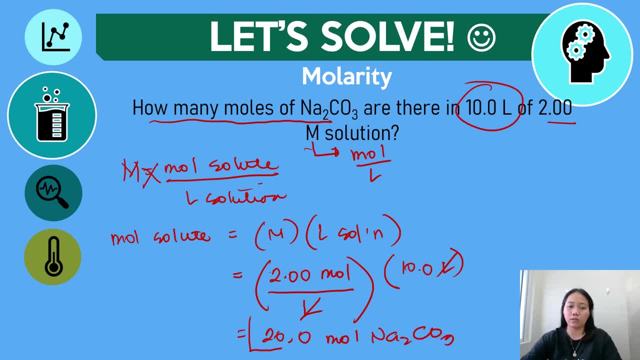 And since that is the unknown, then our answer is already correct. By the way, check for the significant figure. As you can see, we have 3SF as our least significant figure in the problem, so our answer should also contain 3 significant figure as well. 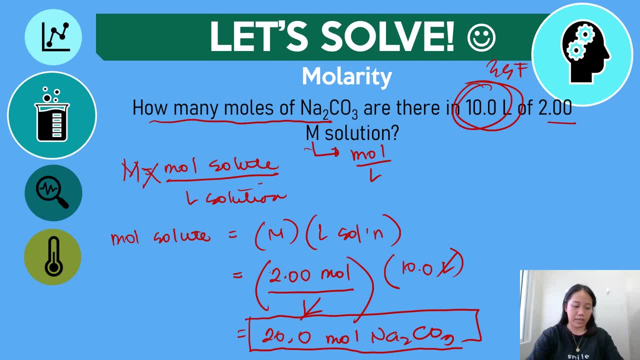 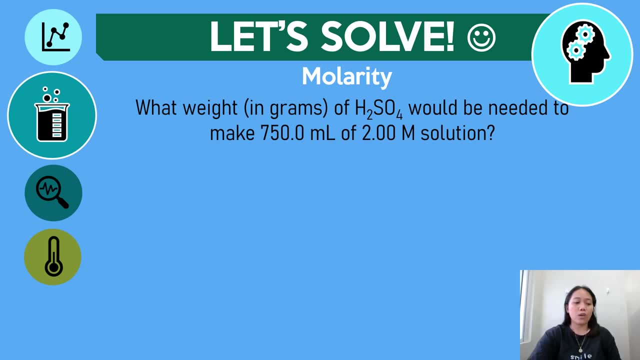 So you have 20.0 mole of sodium carbonate. Now let's have last example of our molarity. So a while ago we solved for the molarity, or the moles, of your solute. okay, given that you have the molarity as well as the liters of your solution, 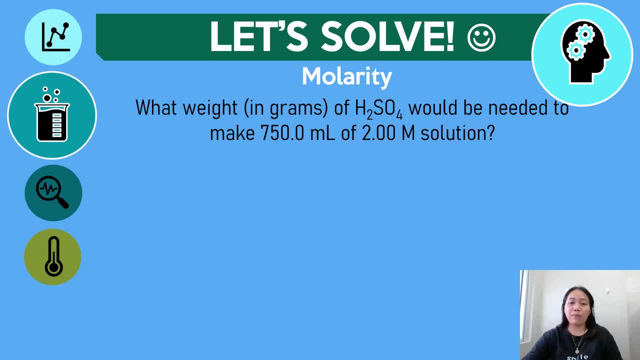 Now, in this case, you were also asked by how many, or what is the weight of your solute in grams? Kanina po, you were asked what is the mole of your solute, but this time you were asked how many grams are there? 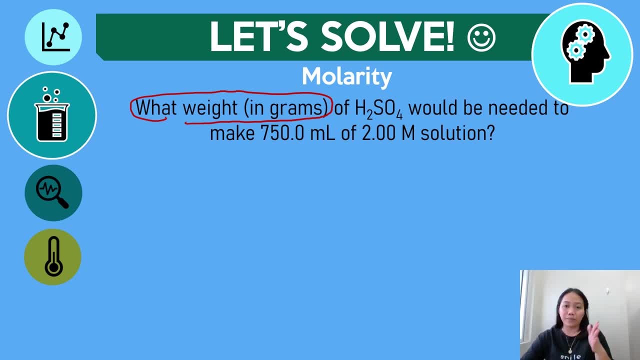 So you will see that the process is just the same, it will be just a little longer. So what weight in grams of sulfuric acid would be needed to make a 750 ml 2.00 molar solution? As you can see, your solution as well, or the volume of your solution, is not in a liter form. 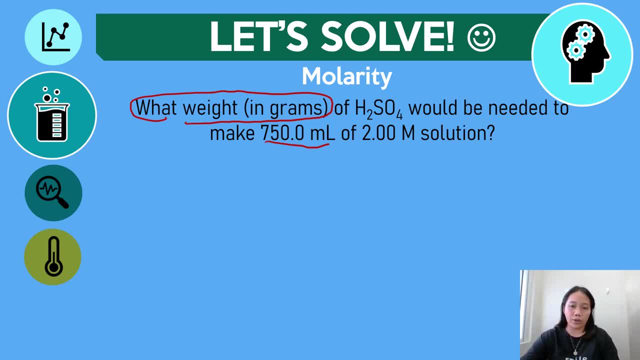 So you need to convert that one later on. But let's start, of course, by writing the formula for us to know ano yung mga kailangan nating variables. So molarity is equal to the mole of your solute. 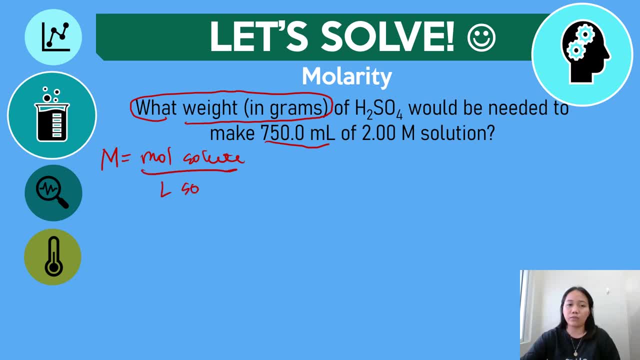 So molarity is equal to the mole of your solute divided by the liters of your solution. And because the unknown is the weight in grams of your solute, all you have to do is to make sure that you solve for the mole of your solute. 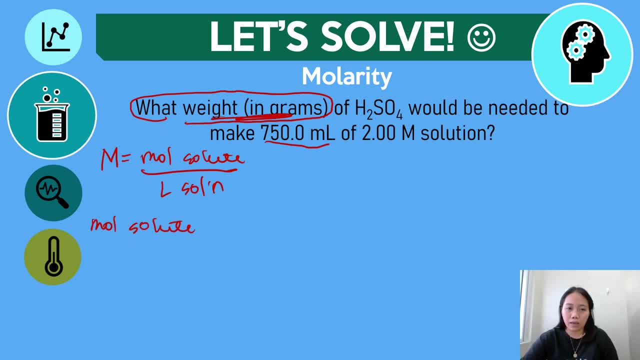 Kasi, of course we just have the value of the liters of your solution and the molarity as well. So wala tayong choice, actually, but to solve for the mole of your solute, And that would be molarity times the liter of your solution. 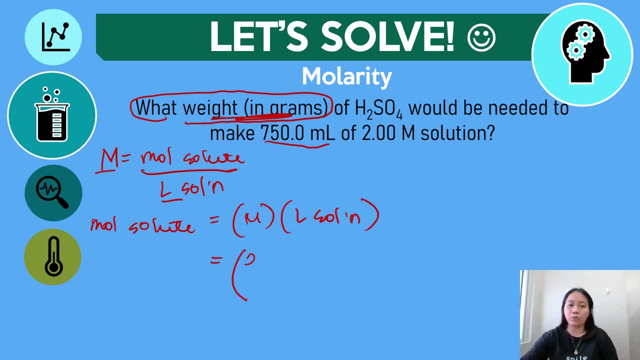 So molecularity is 2.00, that would be 2.00 mol over liter, And because the liter of your solution is not yet in liters, you have to convert 750.0 ml into liters. that would be times ml in liters. So 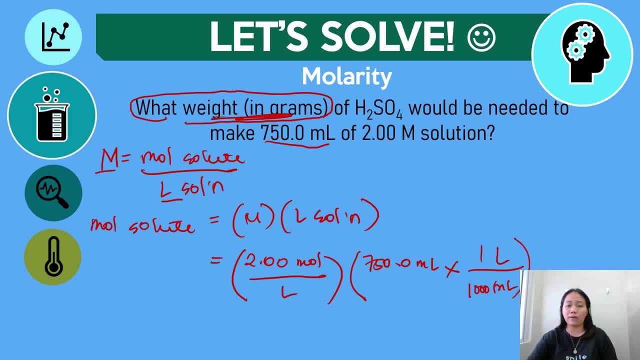 1 liter over 1000 ml. So you cancel out ml now you now have liters, So cancel out liters, because the anone is a number of moles and the number of mole will be 1.50 mol of sulfuric acid. 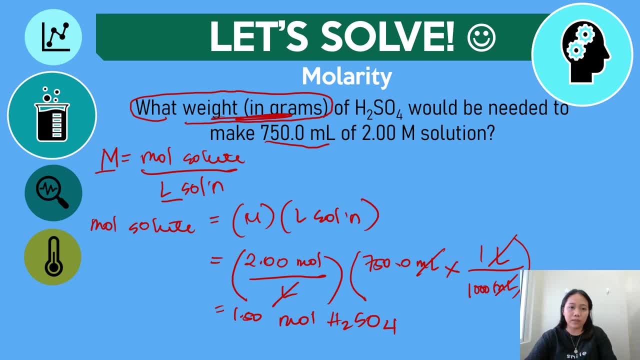 So we are not just done yet, because what we actually have is the number of mole of your solute. If you're going to read the problem again, the ask question is the grams of your solute. So what are we going to do now? We are going to apply again the mole concept wherein you're 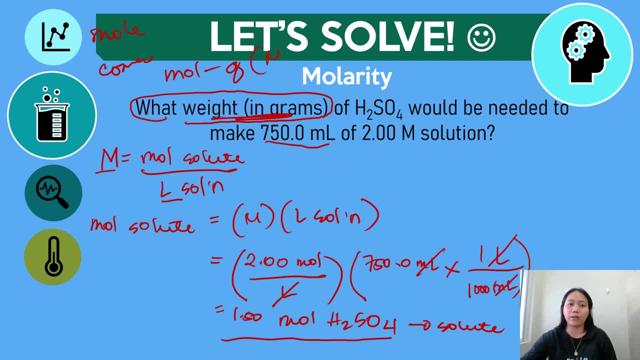 going to apply the number of moles of your solute. So what are we going to do now? We are going to change the mole into grams by using your molar mass. So you have now 1.50 mol of your sulfuric. 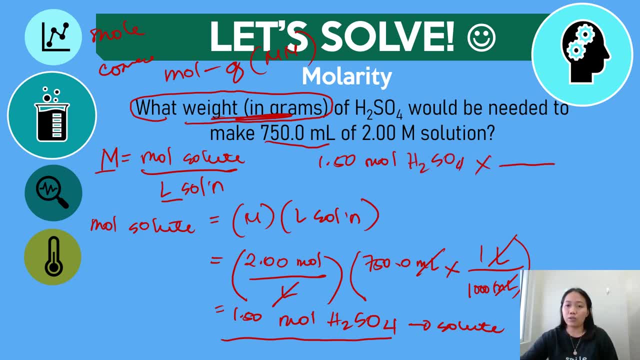 acid. that would be times. since your mole is in the upper part, it's in the numerator, in your conversion factor. it should be in the denominator for you to cancel out the number of mole. So cancel mole. and of course the anone is in grams, so you have grams of sulfuric acid And in 1 mol. 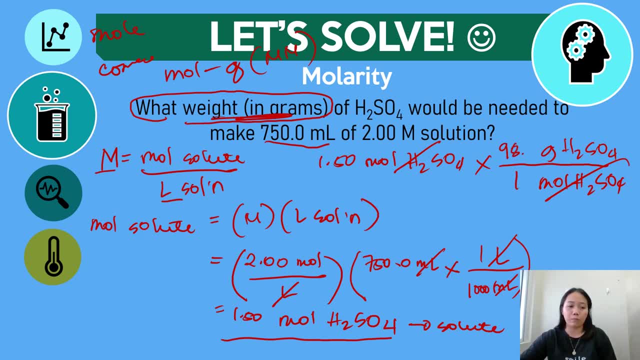 of sulfuric acid. you have 1.50 mol of sulfuric acid. So you have 1.50 mol of sulfuric acid. So you have 1.50 mol of sulfuric acid. We know that its molar mass is 98.072.. Now, if you are having a, 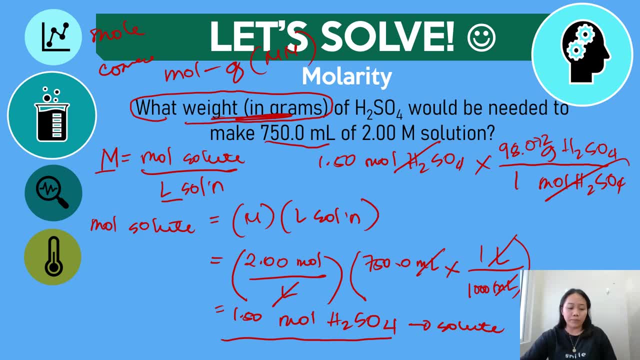 hard time in identifying that molar mass. kindly pause the video and solve for the molar mass of the sulfuric acid first, Then you can resume. So if you're going to have the answer, or if you're going to solve that one, your answer will be 147 grams of sulfuric acid. Why not 147 grams of sulfuric acid? 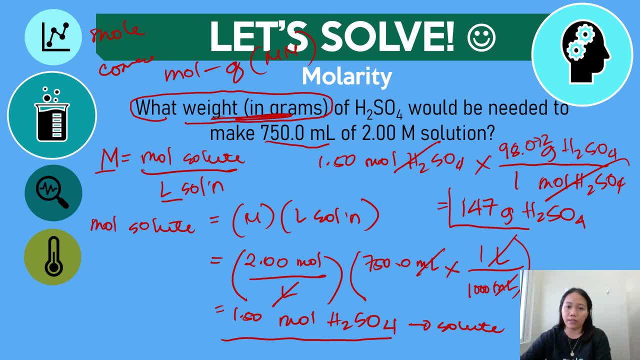 147.108, because we have three significant figure. that's why our answer should contain three significant figure as well. So you have 147 grams of sulfuric acid. Then that answers the question or the problem that we have here for molarity And that is the end of the different. 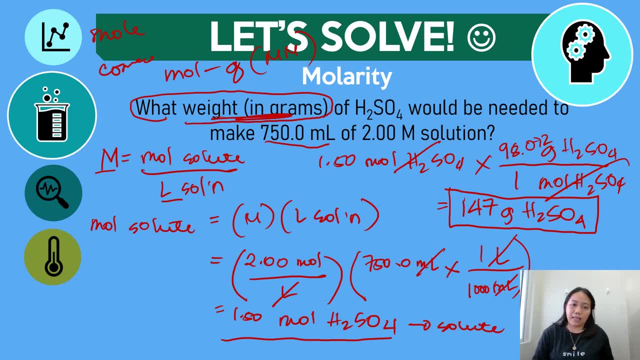 problems. okay, involving molarity. Let us now proceed to the alveolar. The alveolar concentration unit- that is personally for me- is the hardest, because most of the time the given is not actually the variables that will be used in the formula. So you need to make sure. 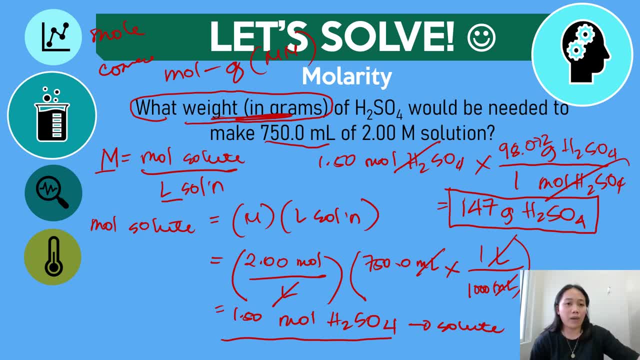 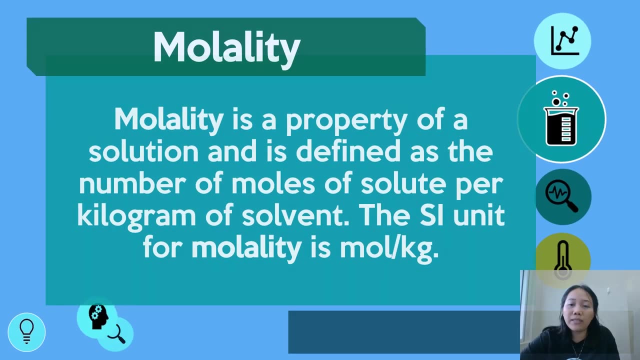 that you understand the basics of solutions for you to be able to compute for molality. Now let's proceed to molality. Now let's proceed to molality. Molality is denoted as mol letter M, okay, and it has a unit of mol per kilogram, because its formula is actually mol of your solute divided by the kilogram of its solvent. 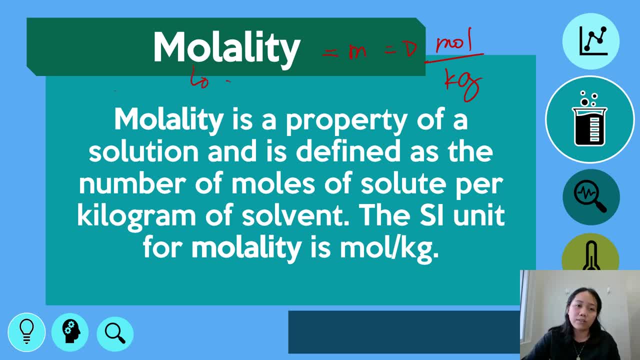 So we call this one as molal concentration: molal. If molarity is molar with an R, okay. molality is molal with an N, okay. So those are the difference between the two And also they have this different formula, of course. 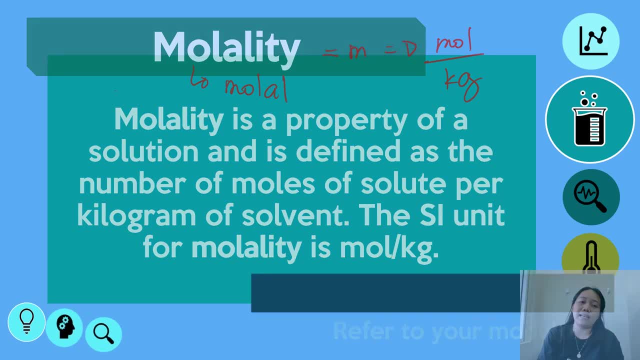 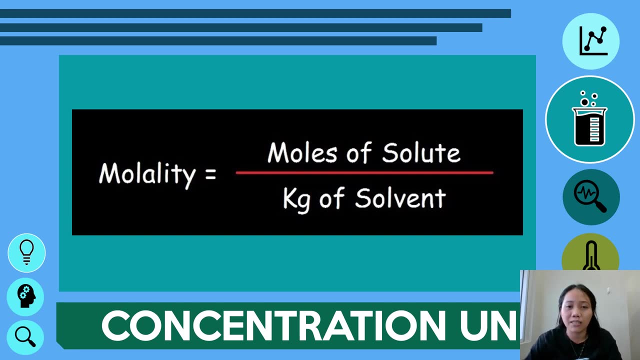 So its formula is: molal concentration is equal to the most of your solute divided by the kilogram of your solvent. Now this is a bit tricky because this is not always given in the problem. That's why the solution will be will take you a little bit longer to solve. 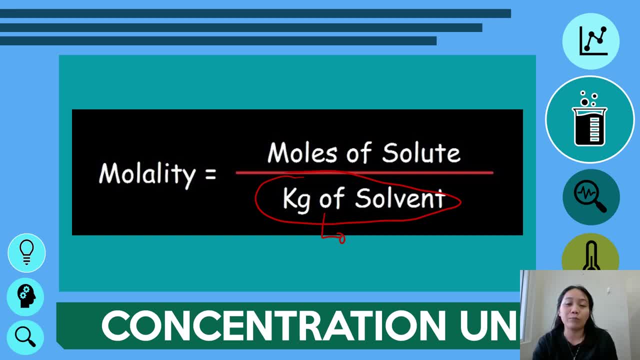 That's why the solution will be: will take you a little bit longer to solve. That's why the solution will be: will take you a little bit longer to solve, But of course, kapag na-master mo naman, but of course kapag na-master mo naman, then you can havet it or you can have the answer din na naman at the end. 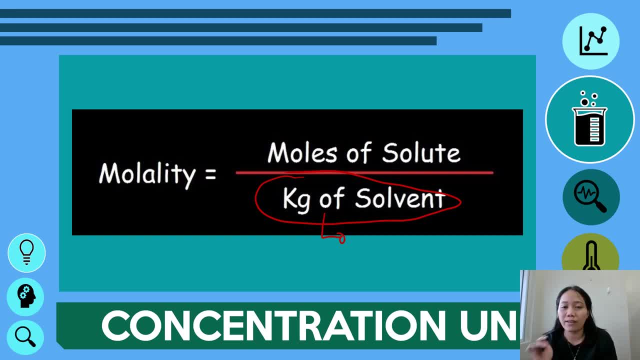 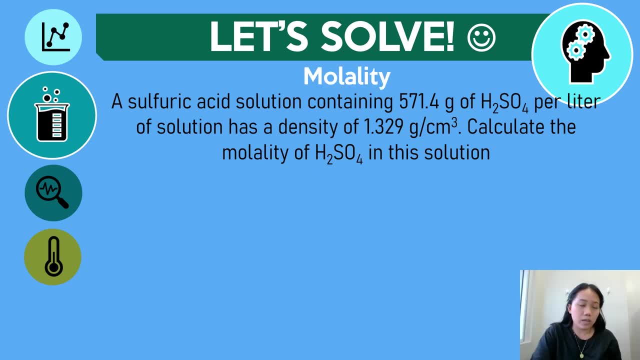 So let's try now to solve one molality problem. Okay, now let's solve for D a problem regarding molality. So we have here a sulfuric acid solution, So we know that a solution contains sulfuric acid and water because it is sulfuric acid solution. 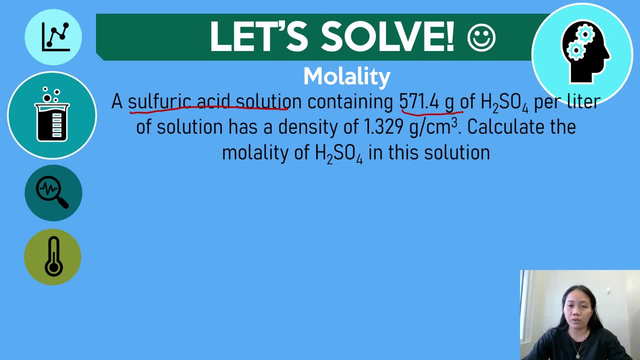 It contains 571.4 grams of sulfuric acid. So that means this value that we have here is actually your solute per liter of solution. That means in this case, in our problem, we have 1 liter of solution And the solution has a density of 1.329 grams per cubic centimeter. 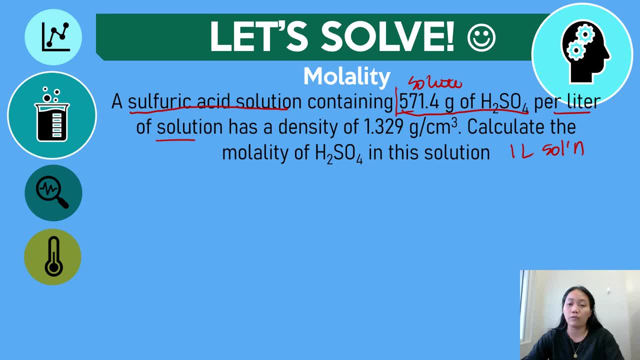 Now the problem is for us to calculate for the molality of your sulfuric acid. So write down first the formula of your molality, That's: molality is equal to the mole of your solute divided by the kilogram of your solvent. 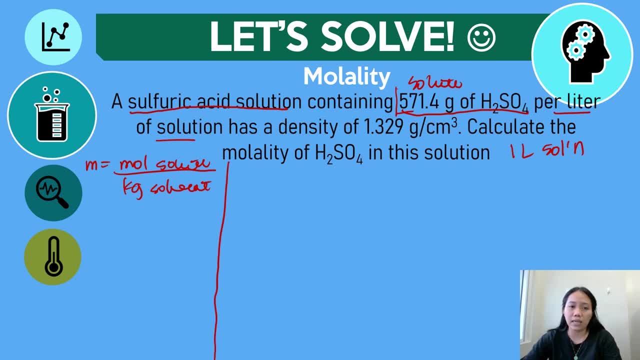 So in this case you will be needing the mole of your solute. And how are we going to do that? We only have one value here that is actually our solute, and that is in grams, And we know how to convert grams into mole. 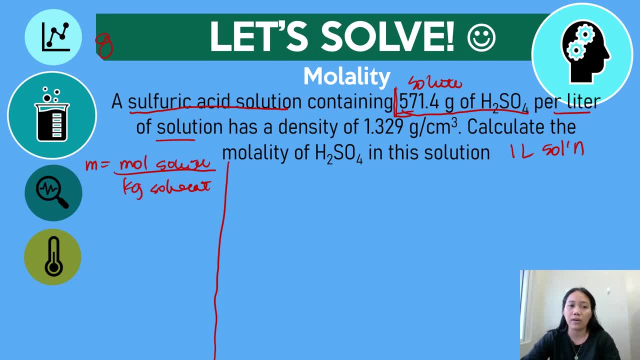 Because we know that we have the mole concept, wherein all you have to do is to change grams into mole using the molar mass. So you have 571.4 grams of your sulfuric acid And since grams is in the numerator part, you have to have the grams in the denominator part of your conversion unit for you to be able to cancel now grams. 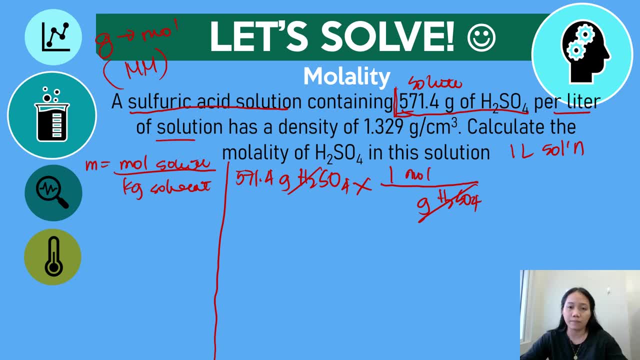 So in every one mole of your sulfuric acid. Okay, we know that it has 98.072 grams as a molar mass, As its molar mass, So you have 5.8223 moles of your sulfuric acid. 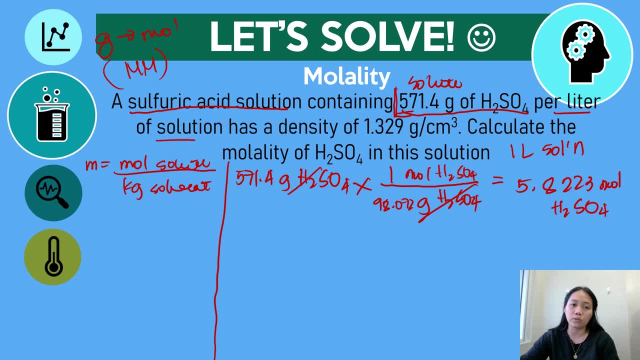 So we're not done yet, because what we actually did is to solve for your mole of solute only. Now let's solve for the kilogram of solvent. Now this will be a little bit tricky because, um, um, To be honest, kilogram of your solvent, or any solvent or in any component in the problem, is not actually given. 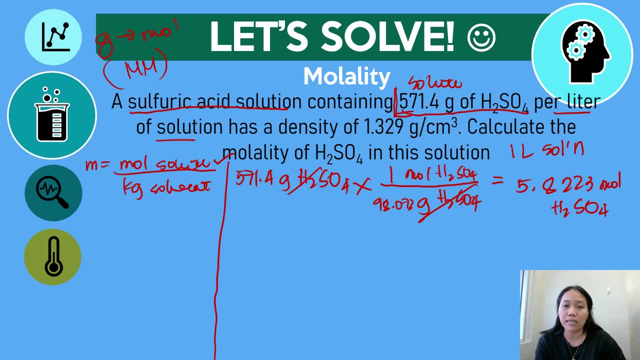 What is given to you guys is actually the density of your solution, So we need to make sure that we are going to use this density in a maximum way, And that would be 1.329 grams per cubic centimeter. The other given that we have is the density of your solution. 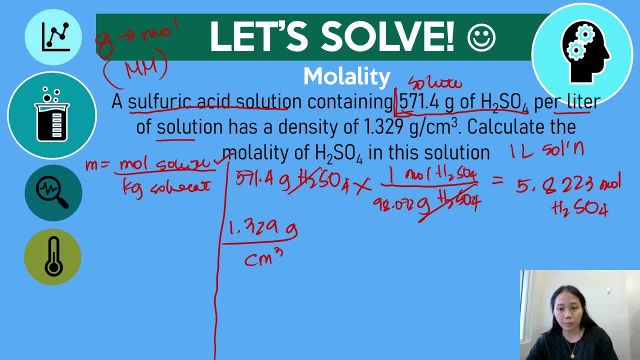 The broken piece is considered a property of maintenance, but the more that we're exercising the possibility of that 들어� patreon, And recall that in the problem as well, the density is actually the density of your solution. So, since both of them are actually the solution itself, maybe we can device a way on how are we going to get the gram here? 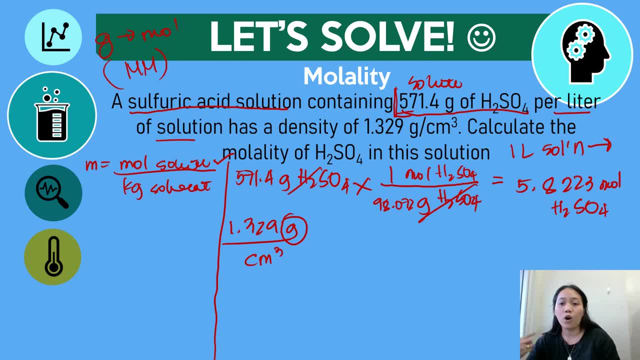 For us to be able to know what is the mass of our solution. But later on we are onативated that this solution is BECOMING a bit over-sooly. Later on we are going to solve now for the mass of our solvent, because we already have the mass of your solute in the problem. 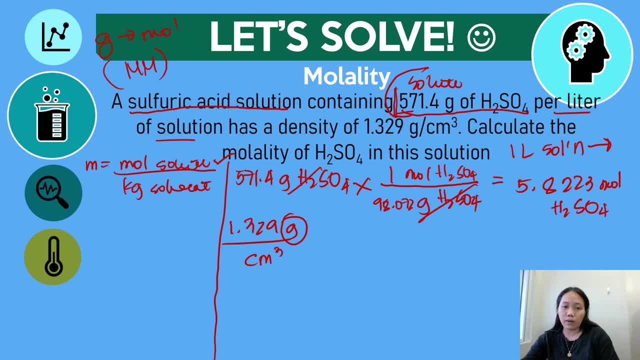 So later on I'll explain how. So let's have this one first, Excuse me. So you have centimeter cube Again. the goal is to have the grams na lang po Si, grams na lang po dapat ang matitira. 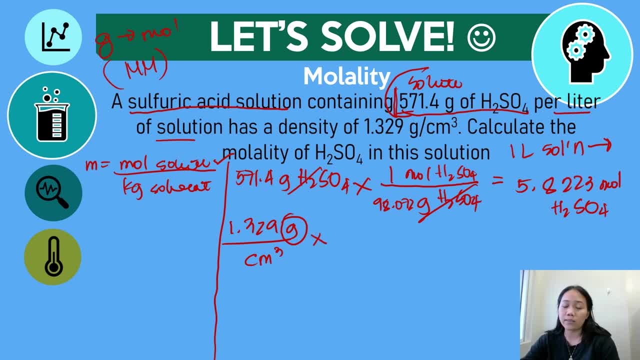 So you have times. Of course we need to convert centimeter cube into liters, because the given volume of your solution is in liters And that would be in every 1 liter of solution there is 1,000 cubic centimeter. 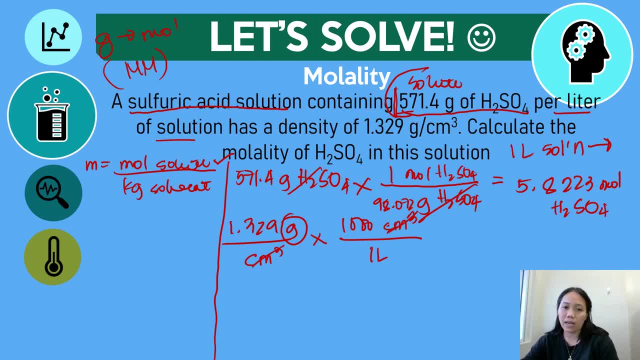 So you can now cancel cubic centimeter. Okay, Still, we have now liters, But we know that the solution it contains 1 liter of solution, So that means all you have to do is to cancel that liters. Now we have grams. 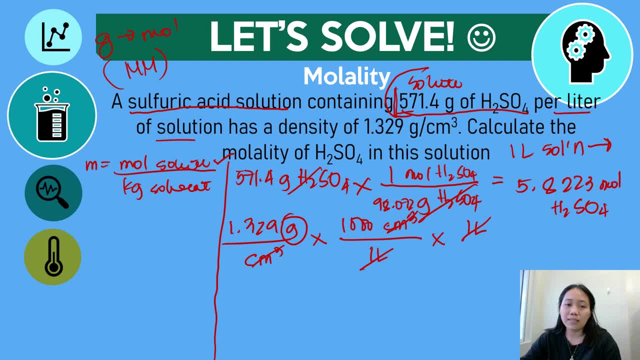 Unfortunately in the problem, since the given is in grams and we need our kilogram in solvent, we need to convert again the grams into kilogram. So we know that in 1 kilogram you have 1,000 grams. 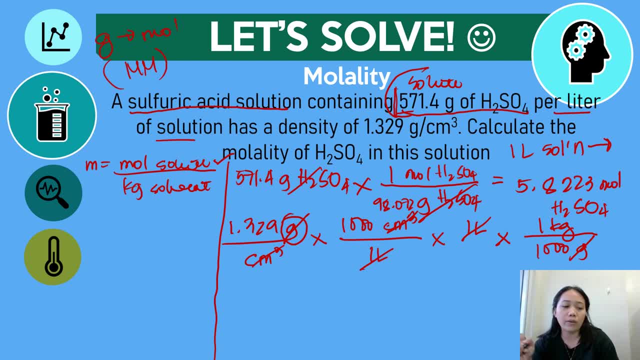 So cancel now grams and you will now have your kilogram. So the kilogram of your solution here is 1.340.. 229 kilogram solution. Please don't forget to label, because you might get confused as you go along with the process, especially if wala hang label yung mga sagot ninyo. 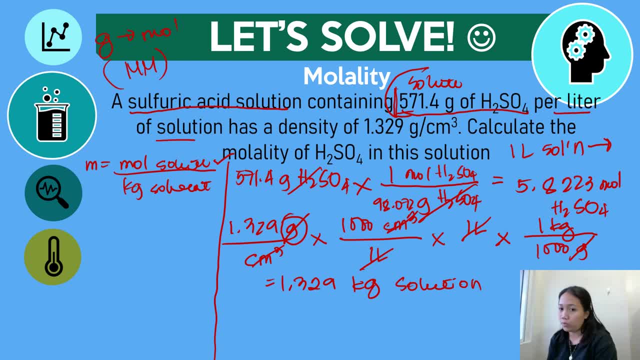 So we have 1.329 kilogram of your solution. What is the next step? We know now that previously in our discussion we know that a solute added to a solvent will give you a solution. In this case, we have now the solution. 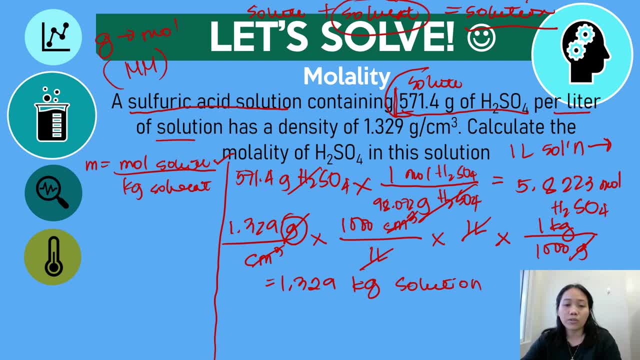 So for us to solve for your solvent, the amount of your solvent in kilogram, you need to be able to know what is your mass in solute. Okay, For you to solve now your solvent- you are going to subtract solution, the mass of your solution in kilogram and the mass of your solute in kilogram. 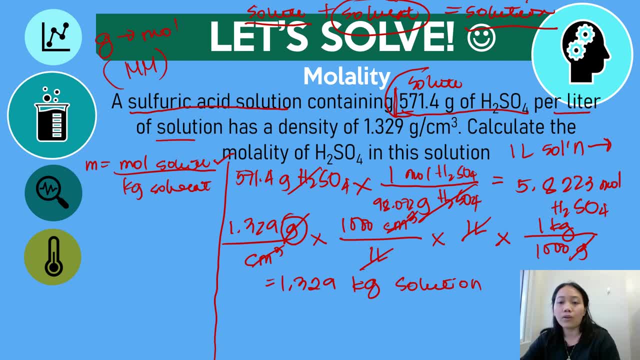 But we don't have the solute- Okay, The mass of your solute. So we have to convert this one first. So you have 571.4 grams of sulfuric acid times and every 1 kilogram you have 1,000 grams and that would give you cancel grams, 0.5714 kilogram of your solute. 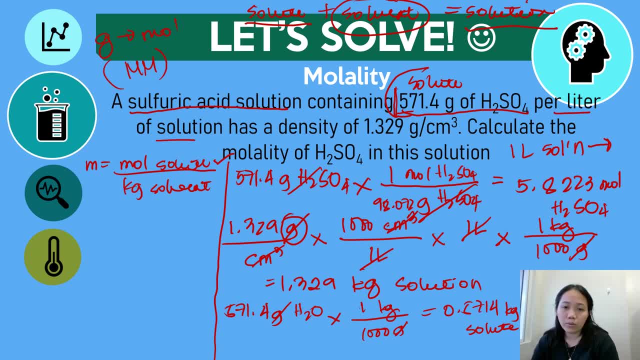 Okay, So now we know that your solution contains 1.329 kilogram And your solute has a 0.5714 kilogram of sulfuric acid. So how are we going to solve for the kilogram of solvent? 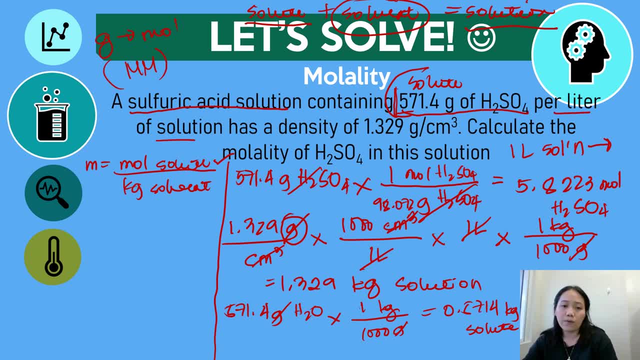 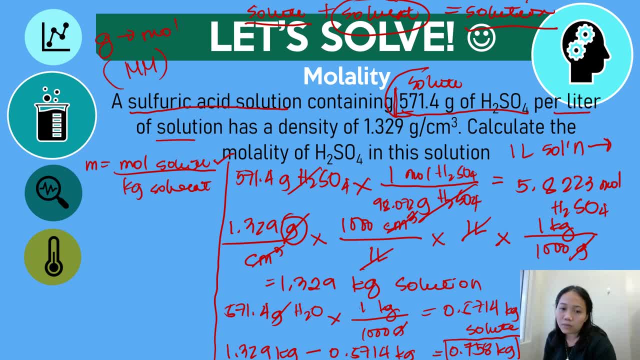 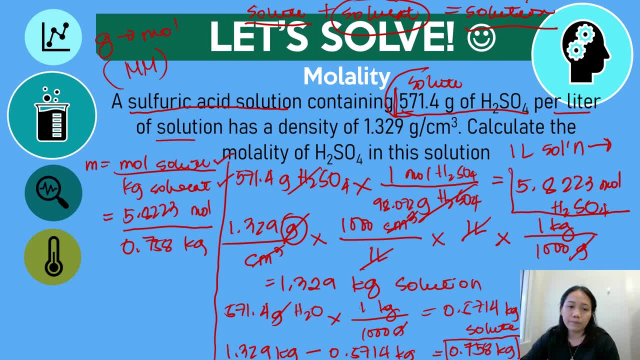 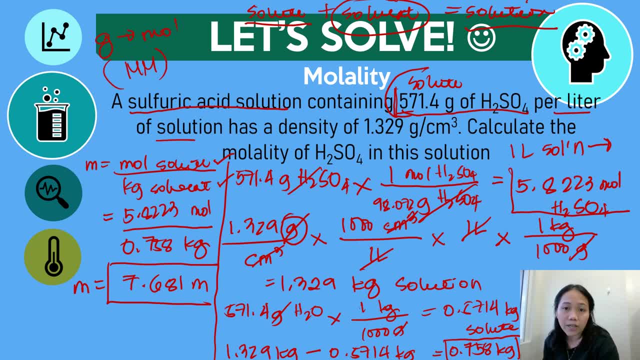 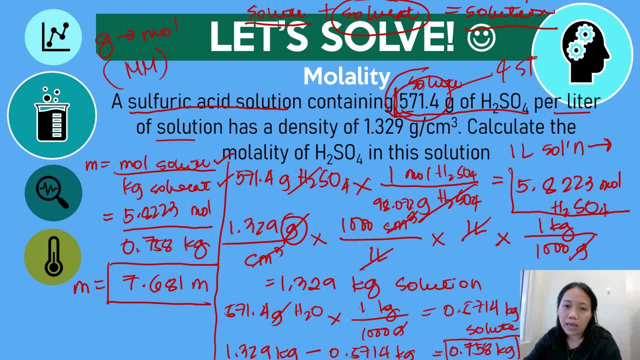 This value here contains 4SF and this value here also contains 4 significant figure, And because the least significant figure in the given values in the problem actually is 4 significant figure, so your answer should contain 4 significant figure as well. So that is for the first problem regarding molality. 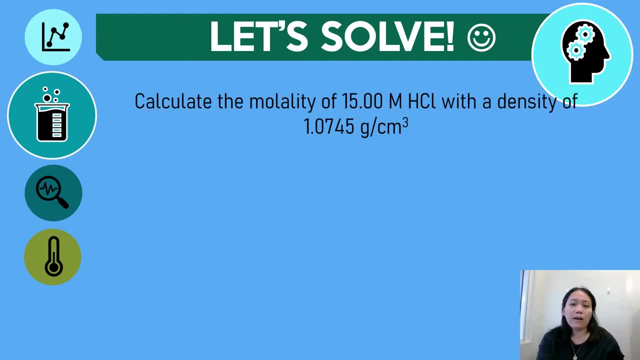 Now let's have another one. Okay, Now, this is actually just the same with what we did a while ago, but it's a little bit tricky in a way, because the given is actually the molarity. Okay, You are given the molarity, but you are asked: for what is the molality of that particular? 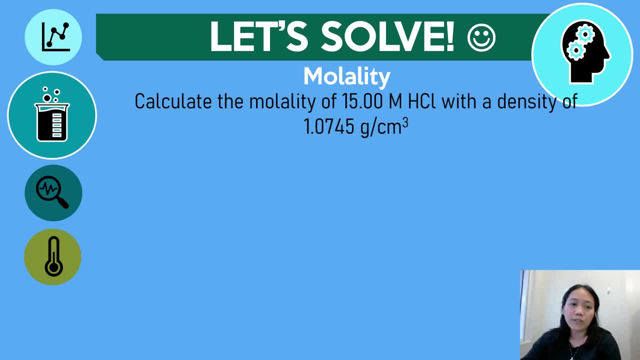 solution containing that molarity. So don't forget to write first your formula, which is mol. Sorry, That is molality. Okay, So small letter M. So M is equal to the mole of your solute divided by the kilogram of your solvent. 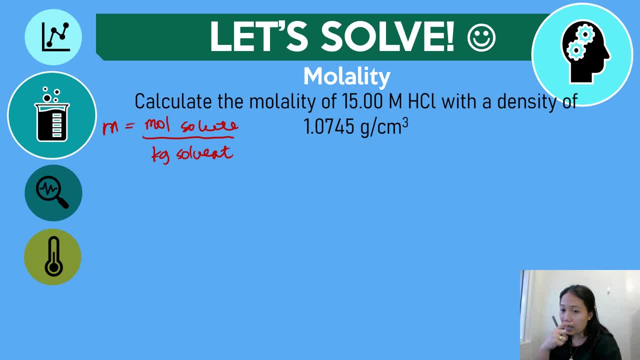 So we need first the mole of your solute, Okay, And identify as well the kilogram of your solvent for us to solve for the molality. So what is the first thing that we need to do? We need to identify what is your solute and what is your solvent. 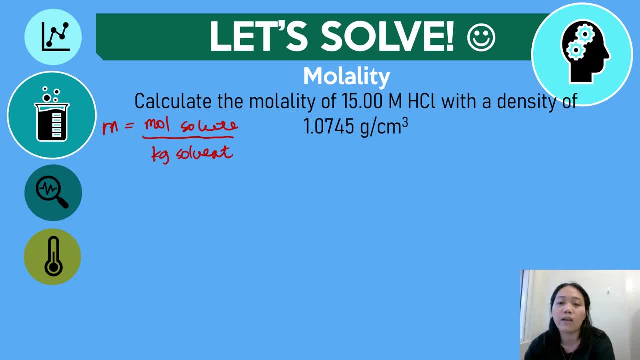 Okay, And identify the solvent in the problem, as well as your solution And, of course, the other problems that will help us, or the other given, rather the other given values that would help us in solving for the molality in this problem. So we have a 15.00 molar HCl. 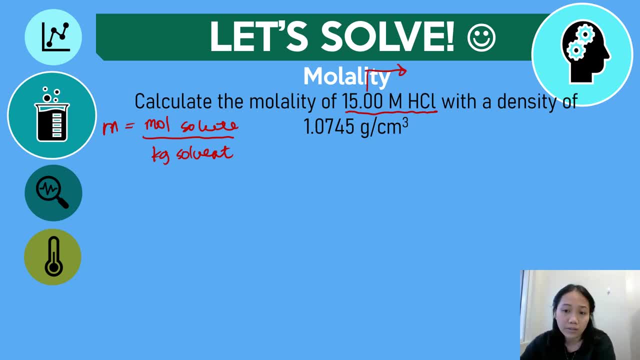 But if you're going to convert that 15.00 molar of HCl, you will get 15.00 mole over over L, Because recall that the formula of your molarity is mole of your solute divided by the liters of your solution. So in that case, what we have actually here, the 15.00 mole, is actually 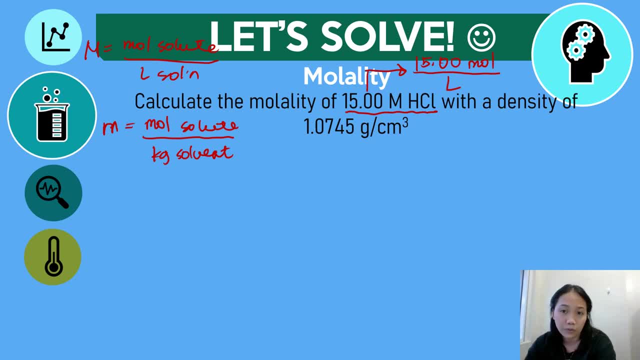 the mole of the solute, But of course we need to solve it first. So we need to assume that in this case we have one liter of solution. Okay, we will use this. we will use this particular value, which is 15.00 molar, which is converted into 15.00 mole per liter, based on the formula of: 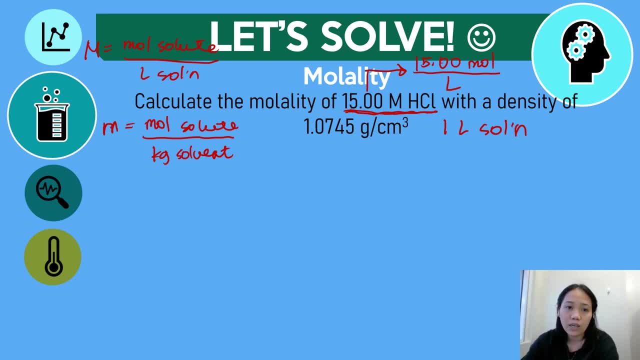 your molarity. So now you have 15.00,. okay, that is 15.00 mole over liter. Since we assume that there's one liter of solution, we have 15.00 mole per liter. So now we have 15.00 mole per liter. 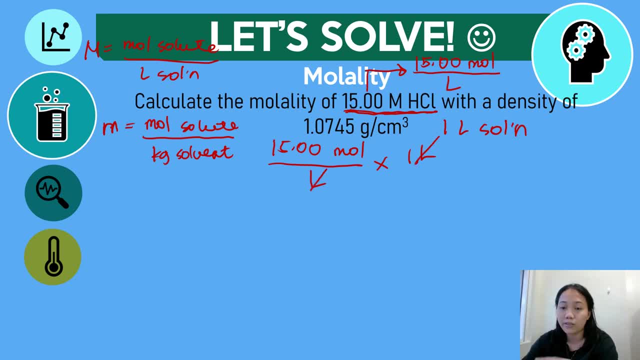 We can now simply multiply it by liters to cancel the liter, And now you will have 15.00 mole of your HCl. And what is your HCl in the problem? It's actually your solute. And because you now have 15.00 mole of HCl, which is your solute, then your numerator is already done. Let's proceed now to 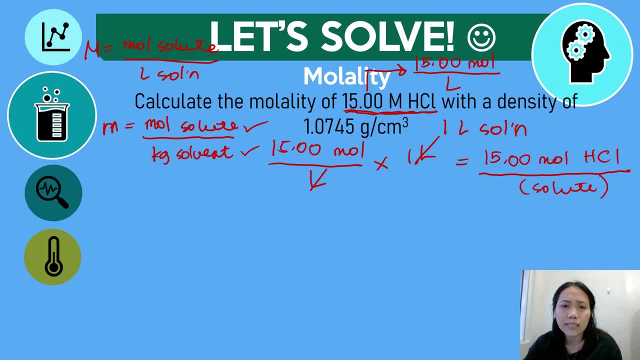 the kilogram. Okay. so since our given is actually in density, we will just do, or we will just follow what we did a while ago in the previous problem, wherein we are going to solve for the density. Okay, you have grams over. 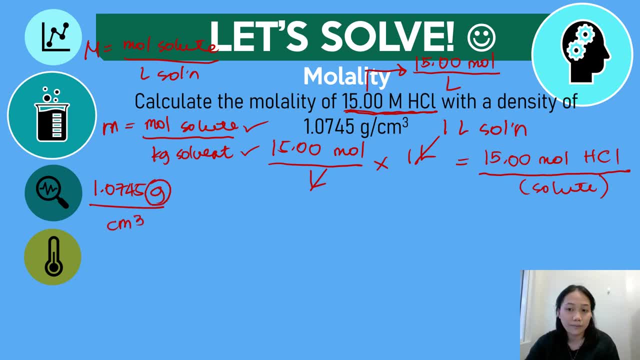 cubic centimeter. we are going to solve for the grams here. Okay, so we need to convert this one into 1000 cubic centimeter over one liter to cancel cubic centimeter and multiply it again to one liter, because there's a one liter of solution that we assumed a while ago And now you can actually. 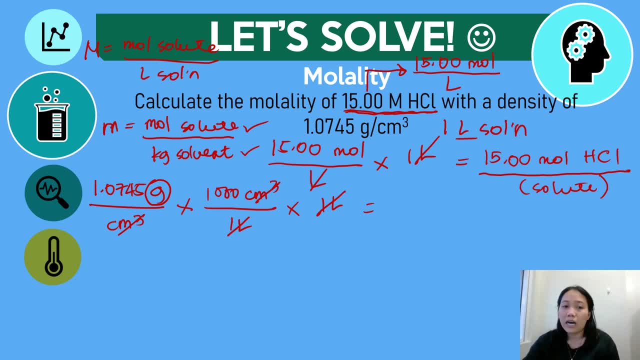 have now the grams of your solution because, remember, this density is the density of your solution, Density of your solution. Don't forget that. So we now have the grams, but we need the kilogram because we need the kilogram of solvent later. So you need to convert now the grams. So in 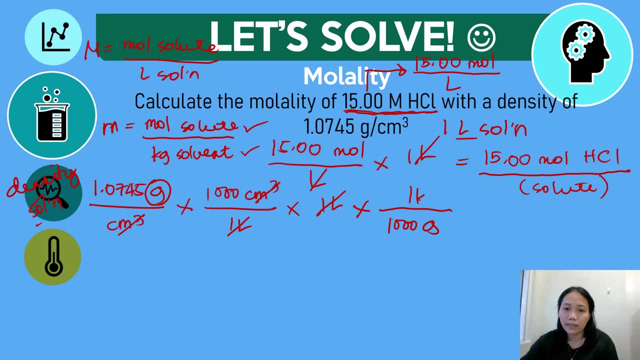 every 1000 grams. okay, it is the one kilogram, So you cancel grams and now you will get 1.0745 kilogram of your solution. Don't forget that, because it's your solution Now, just like the previous. 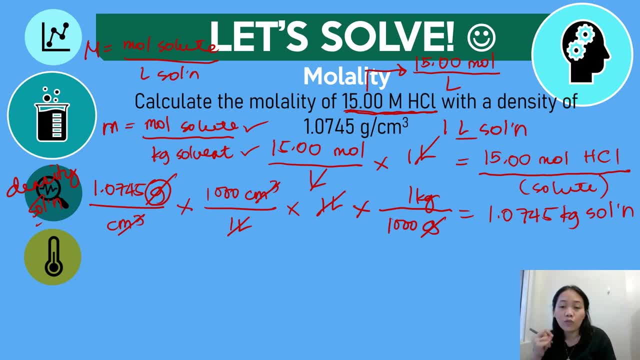 problem. we need the kilogram of your solute. Do we have a gram or any value that we could use in the problem for us to be to solve for the density? Okay, so we need the kilogram of your solution. So we need. 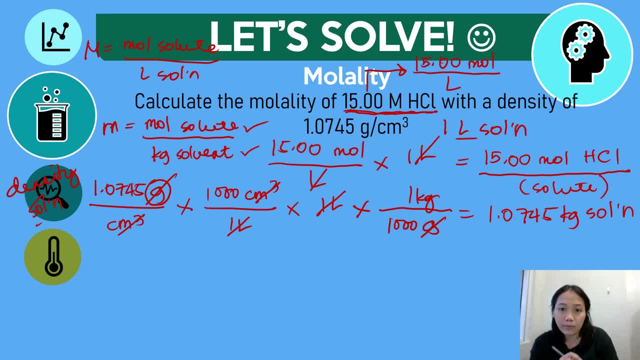 to solve the kilogram of your solute? Yes, we do, And that is the 15.00 mol of HCl. That 15.00 mol of HCl will be used for you to convert it into gram And since it's mole, into gram, again, it's the mole concept where you're. 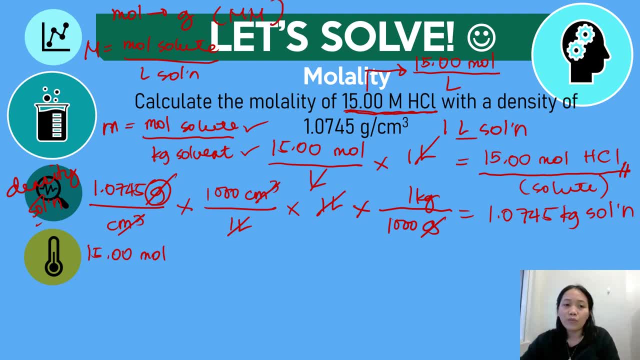 going to use the molar mass for you to solve for the grams or the mol of the particular substance. in this case we need to convert mole into grams, so you need to put mole in your denominator for you to be able to cancel it. and this is mole of hcl. so in every one mole of hcl. 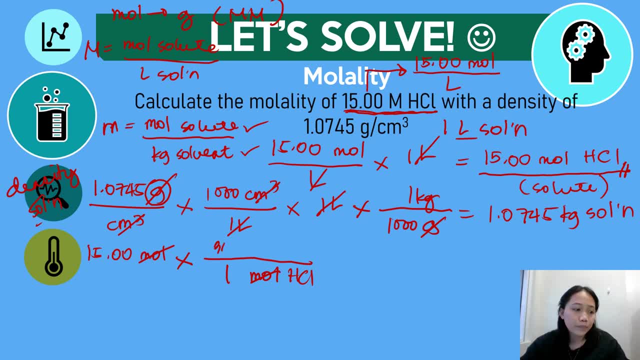 we know that its molar mass is 36.458 grams of hcl. okay, and we know dahil naka grams pa siya. it's not the final one, because we need to convert it first into kilograms. so you have gram and you have one kilogram. cancel gram and now you'll have the answer: 0.5469 kilogram of hcl. 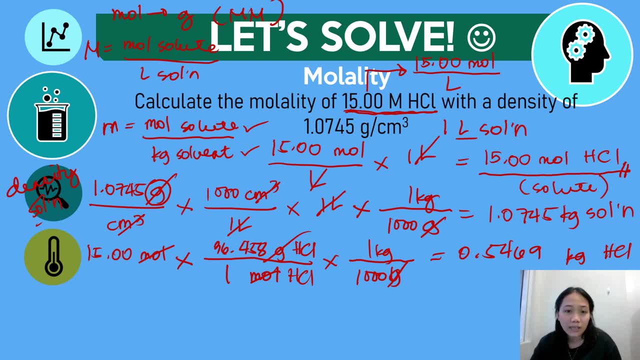 which is your solute. so can we solve for the kilogram of solvent? yes, we can. so you have now 1.074, 745 kilogram of solution, okay, minus 0.5469 mole, or kilogram plus, rather, of your hcl, which is your solute, and you will be given with an answer of 0.5276 kilogram. 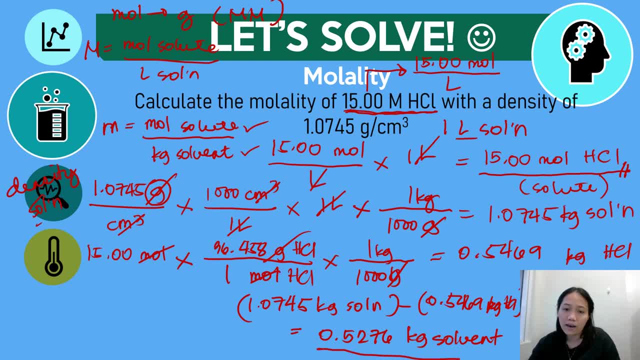 of your solvent. so you now have the solvent. so can we solve for the molality now? yes, we can, because we already have the mole of your solute and we already have the kilogram of your solvent. so m m is equal to what is the mole of your solute. it is 15.00 mole all over the kilogram of your solvent. 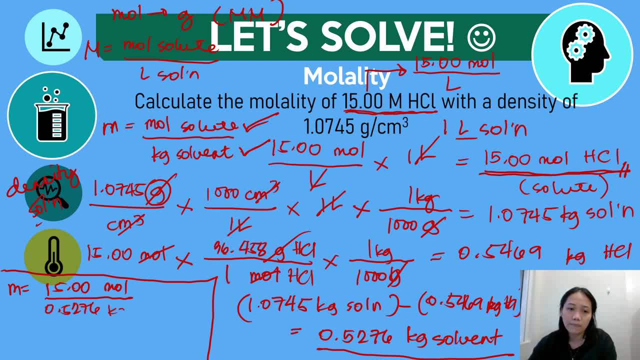 which is 0.5276 kilogram. and now you will have the answer: 28.43 m or 28.43 molal with an m. so we have four significant figure because, going back to the problem that we have to solve for the molality of the solvent, so we have four significant figure because 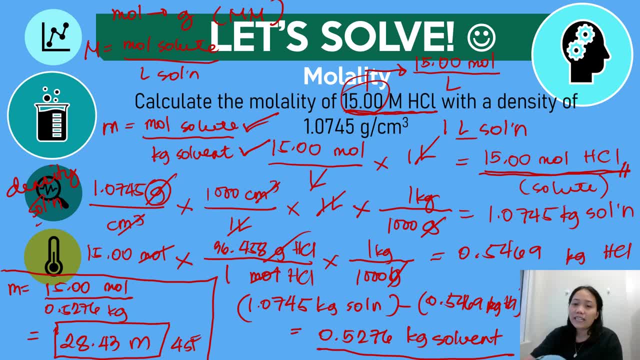 going back to the problem that we have to solve for the molality of the solvent. so we have four. least significant figure is four. so your final answer is 28.43 molar of solution. yeah, okay, so we're done already with the second problem. let's proceed to. 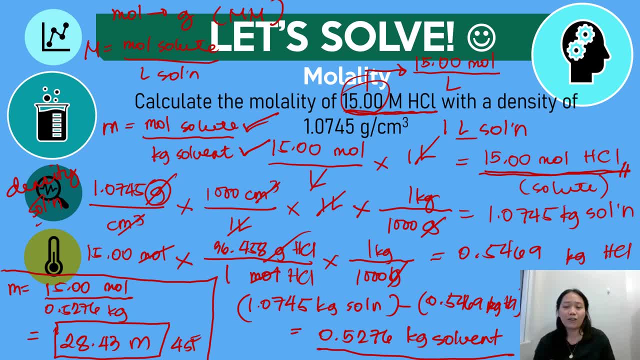 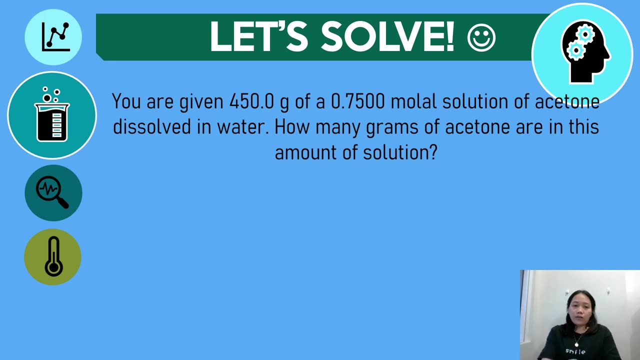 the last one, okay, before we proceed to the last concentration units, which are ppm and ppb, and let's see if we could also have the ppt or the parts per trillion. okay, let's last problem. okay, there you go. you are given 450 grams of a 0.75 molal solution of acetone. 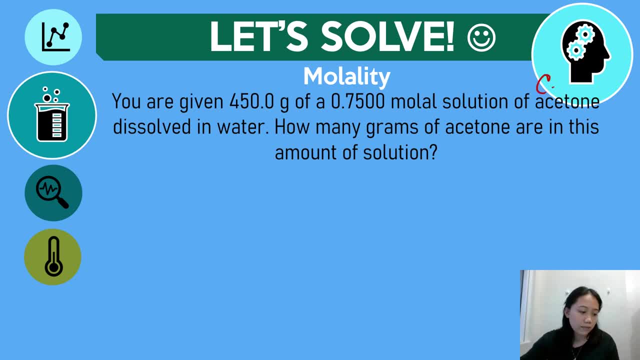 dissolved in water. so acetone guys is c3, h6. oh, okay, we could have. uh, we already have the formula dissolved in water. so that means your acetone already is your solute and your water here is your solvent. how many grams of acetone are in this amount of solution? 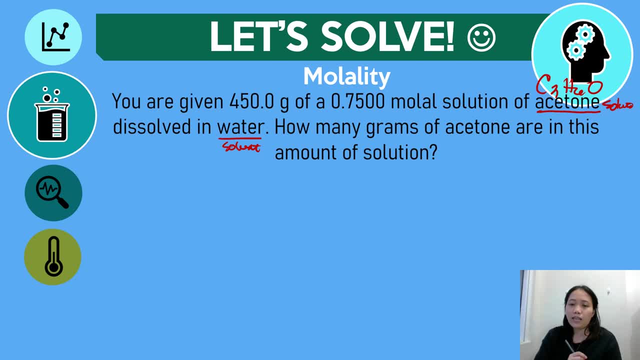 this problem is very, very tricky. okay, it's a little bit more tricky than the other problems that we have in molality. why? here's the thing: if you're going to read the problem again, okay, you will gain two different situation. okay, you are given 450 grams. that means you have a particular- let's see, one kilogram of a 0.75. 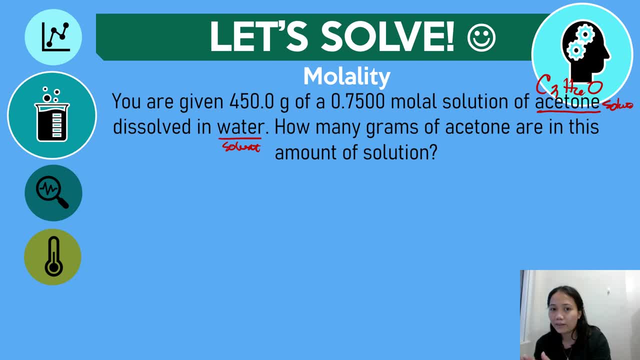 molal solution. you have one kilo of it and you are only given 450 grams. okay, and that is a molar solution of acetone dissolving water. the question now is how many grams of acetone does of acetone are in this amount of. 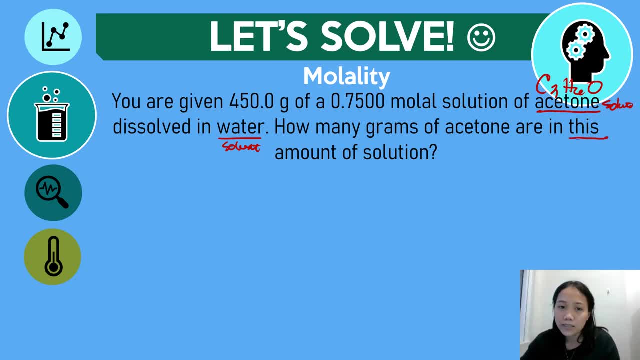 solution. What particular value is this question asked in this question is telling us or asking us: Yung sinasabi niya ditong this amount. What particular amount is this problem talking about? It's the 450.0 grams. Tinatanong po niya. let's say it. 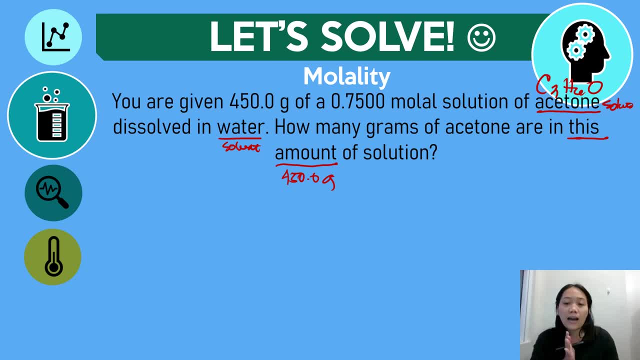 in Tagalog. tinatanong po niya kung ilan ang acetone, ang gram mo ng acetone, which is your solute, sa isang 450 grams, na kinuha mo sa isang 0.75 molal solution. 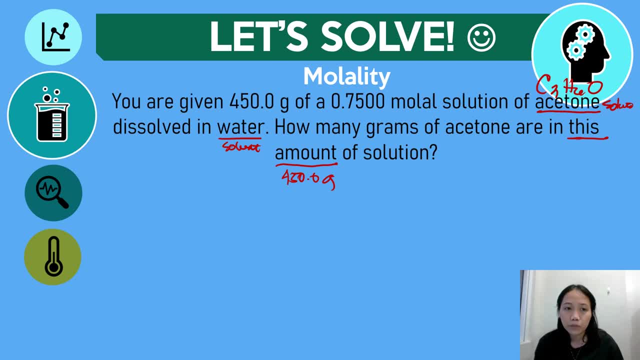 Para mas maintindihan po ng lahat, dahil medyo mahirap siya, isipin nyo lang, meron kayong coke sa ref, Ang coke na yon. it contains 1.5 liters Kumuha ka ng isang baso. 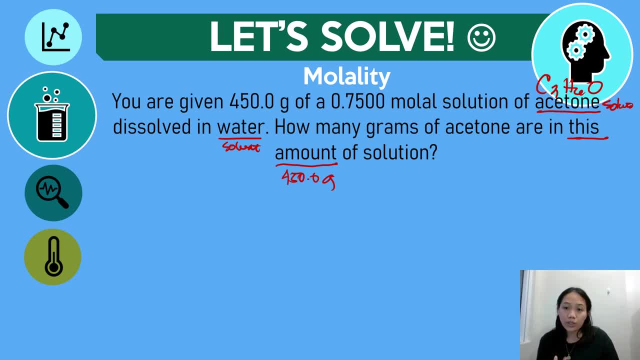 Kumuha ka ng isang baso ngayon. Of course, ininom mo. you take that one cup of coke, Pagkainom mo. the sugar level na ininom mo sa isang baso, is it the same? 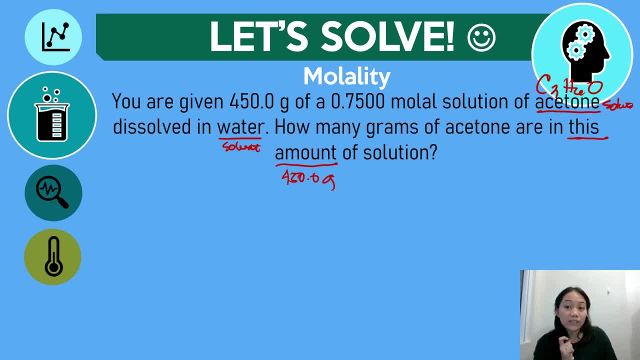 in the sugar level of, or the sugar content, rather sugar content, hindi level Sugar content. nung ininom mo na sa isang baso, compare dun sa isang litro pa na natira or 1. something. 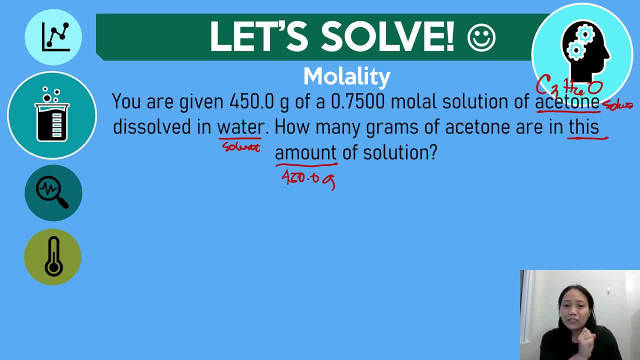 liter? Of course hindi Okay. So ibig sabihin, because you get only 450 grams of your acetone in a particular container, na siguro 1 kilo or whatever, because you have that, yung 450 na nakuha mo, it will. 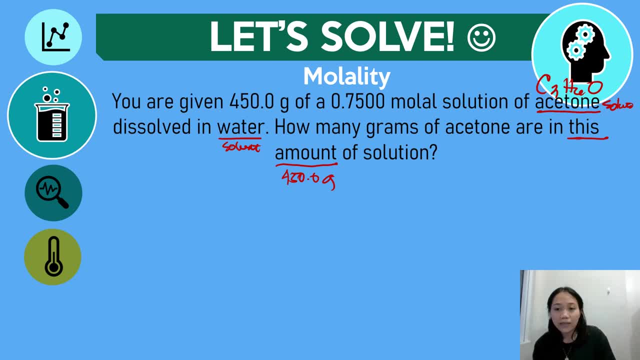 have different amount of acetone, Kahit na pareho sila ng molal. Okay, So that is the idea. So ang tinatanong po ng problem is how many grams of this acetone, of this particular acetone? 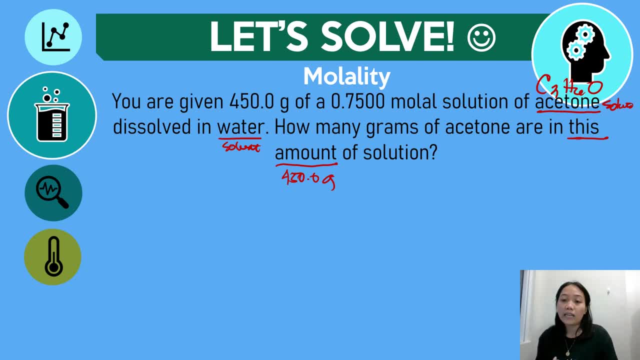 is in the sample na kinuha mo, which is 450 grams. Now let's solve. Okay, We know that molality is equal to the mole of your solute divided by kilogram of your solvent. Of course we need 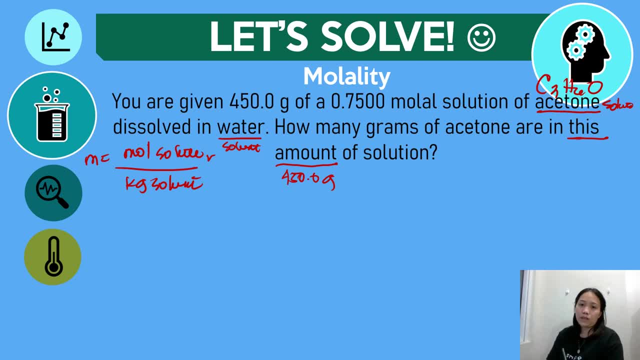 the mole of your solute. But um how many grams of your acetone? by the way, basta nandyan lang yung formula na yun. We will be needing that one later on. But let's focus first on this value. 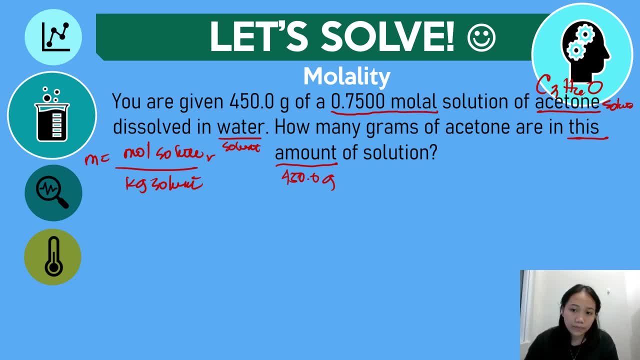 The 0.75 molal solution. If you're going to write it just like what we did a while ago in molarity, you will have 0.7500, 0.7500 mole over 1 kilogram. What does it mean? 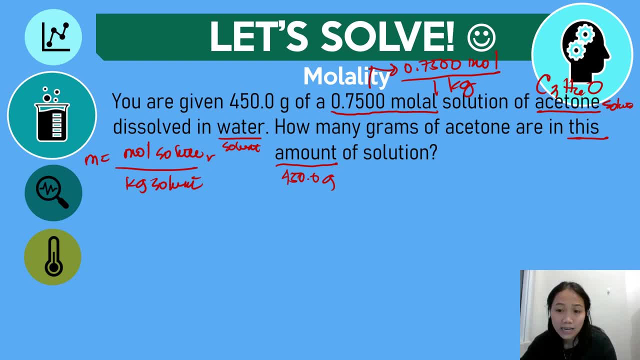 Okay, We are now going to assume, based on that molality, we are going to assume that we actually have 1 kilogram of solvent Ulitin ko solvent lang po, Because if you're going to recall the formula of your 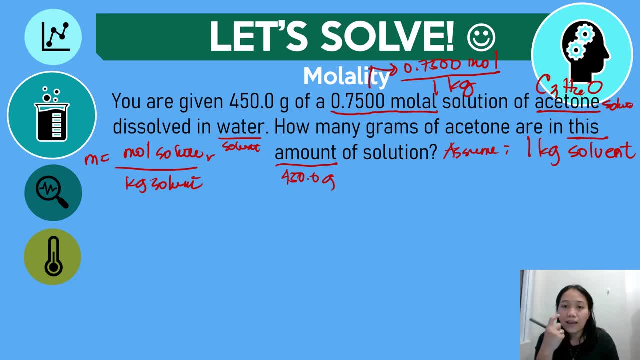 molality, that is mole of your solute divided by kilogram of your solvent. That means in that particular molal of solution you have 0.75 mole of solute in a 1 kilogram of solvent. So nag-assume tayo ngayon that we have. 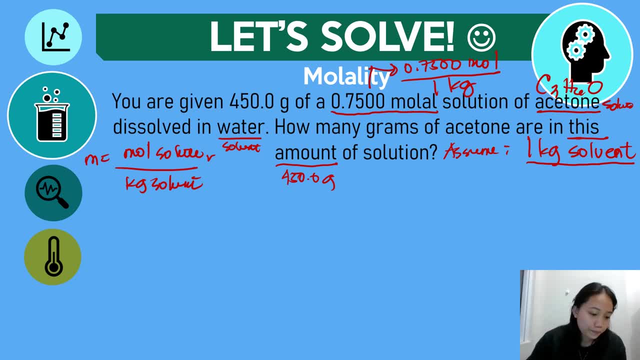 1 kilogram of solvent. What is the next step? We are now going to identify the number of mole of your solute. Okay, So the number of mole of your solute is, let's see, you have 400,. 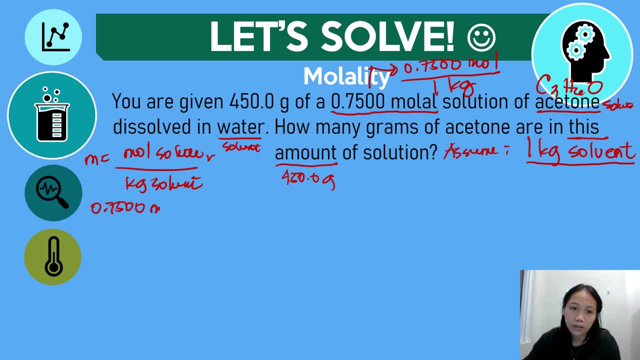 sorry, 0.7500 mole of solute over kilogram And that we know we have 1 kilogram of your solvent, So we cancel out now kilogram And you will now have 75.75 mole of your solute. 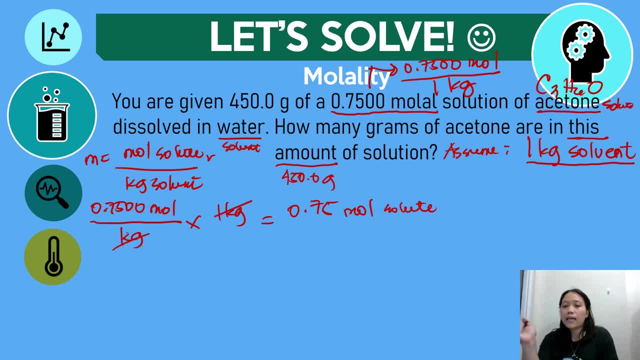 Okay, Mole of your solute. Okay, Let's take it aside first, because we will be needing that one later on. Now, the next step is for you to identify the kilogram of solution. na kinuha mo. Okay, Remember ha. 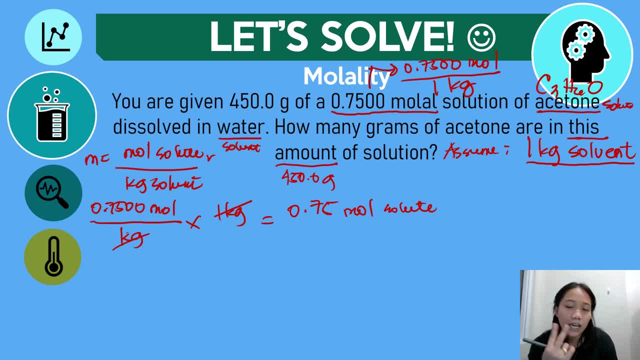 I told you a while ago, we have two situations here. Yung natira okay At yung kinuha mo, which is the 450 grams of 0.75 molal solution. So dahil kumuha ka ng 450.0 grams, okay, that is now your new solution, yung meron ka. 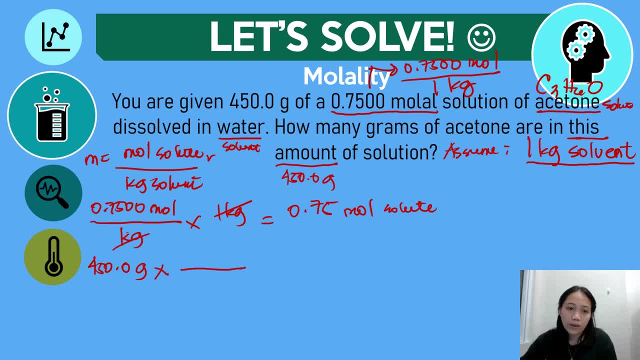 So convert that one into kilogram. So you have now, in every 1,000 gram you have 1 kilogram. All you have to do is to cancel the grams and now you have 0.450 kilogram. 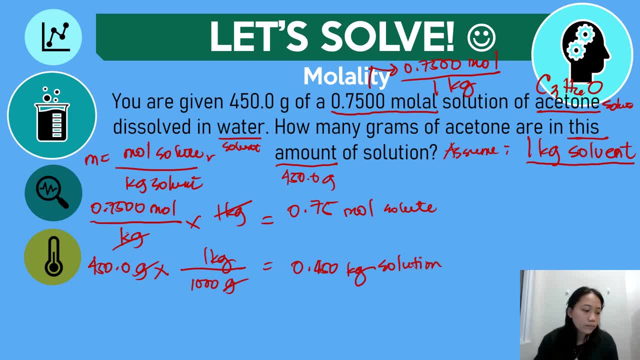 And that is the kilogram of your solution. Next, let's identify the kilogram of your solute, Because we need that for us to identify the number of acetone na meron tayo dun sa 450 grams. So what particular value ang pwede natin gamitin? 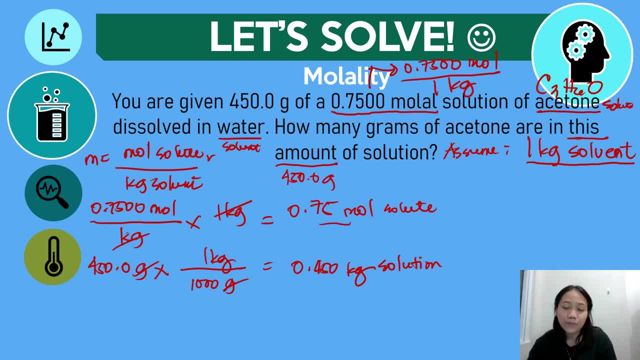 We can use this one because it's the mol of your solute. Again, you are changing a mol into grams. that means we are following mol concept And we will be needing the molar mass of your solute, which is, in this case, acetone. 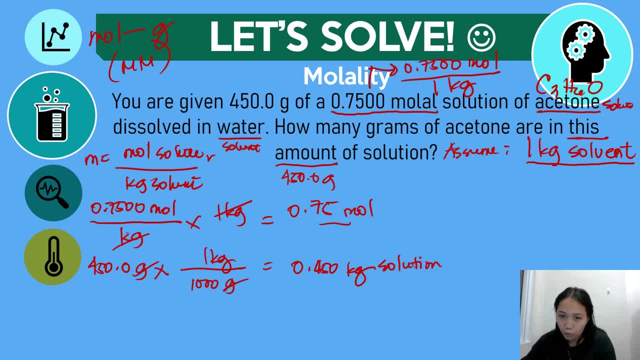 And that would be C3H6O, That is acetone C3H6O, And we're going to multiply it. Okay, in every 1 mol of your acetone molar mass is 58.08 grams of C3H6O. 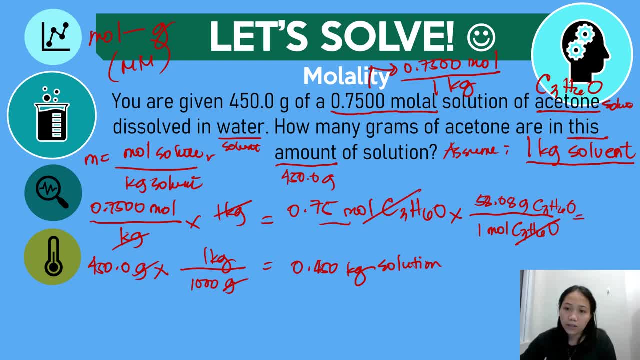 You cancel now the mol And you will get an answer of 43.. 53.56 grams- okay, grams- of your solute, which is C3H6O. Okay, that is your acetone. Now, what does it mean? 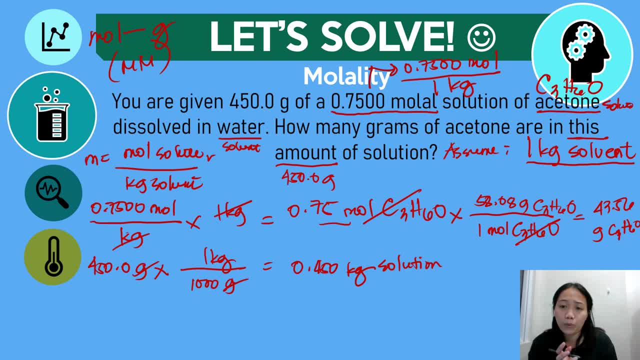 Okay, anong makukuha natin dyan sa 43.56 grams. We need to identify now what is the total number of grams? okay, of our solution. Okay, so we know We have 1 kilogram of solvent. 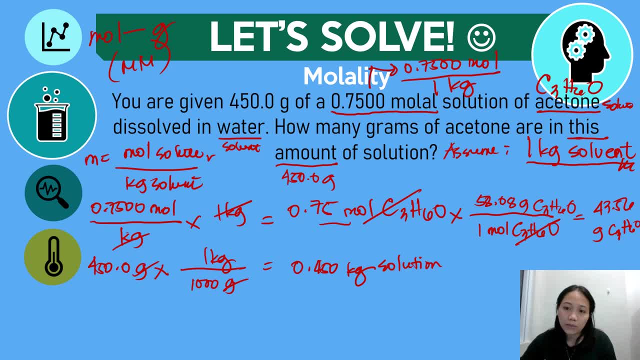 Okay, we have 1 kilogram of solvent, So dahil naka-grams tayo dito. we can just simply change that 1, the 1 kilogram of solvent. So you have 1,000 grams and that is your solvent. 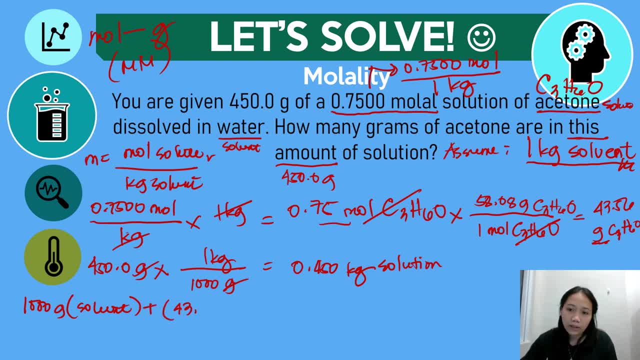 Plus, you have 43.56 grams of your acetone, which is your solution, solvent. Sorry, your solute, rather Your solute, that is the acetone, And you will, And you will get a value of 1,043.56 grams of solution. 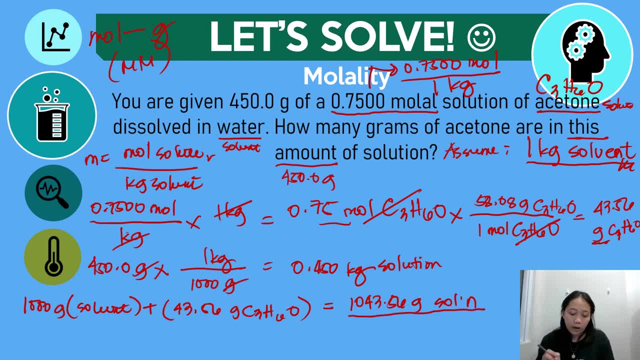 Bakit po siya importante? Ito na yung pinaka-importanting part. As I've told you a while ago, kumuha ka lang ng part, kumuha ka lang ng 450 grams sa isang 0.75 molal. 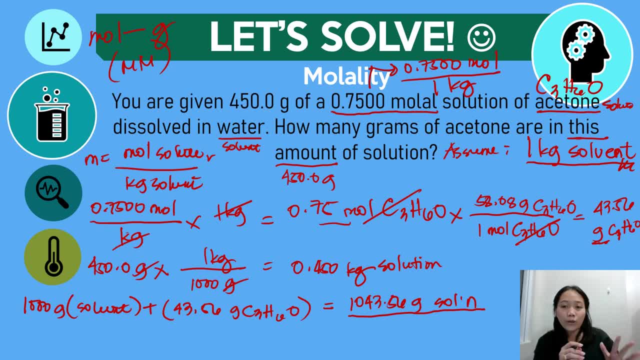 Hindi natin alam kung ilan yung pinagkuhanan mo. Ngayon we identified it already. Ibig sabihin, kunwari sa isang container you have 1,000.. So you have 1,043.56 grams ng solusyon. 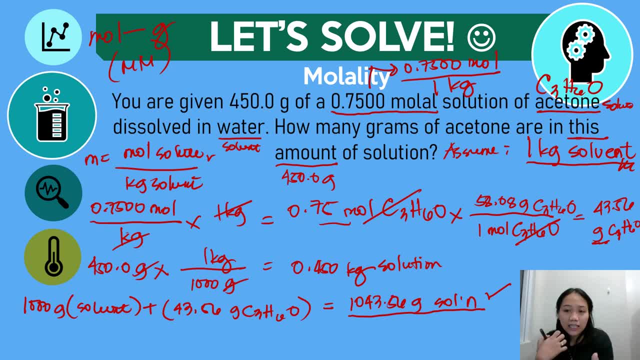 Kumuha ka ngayon ng 450.. Paano mo ngayon malalaman what is the amount of your acetone? All you have to do is to divide. okay, Amount of your Amount of acetone C3H6O is equal to. 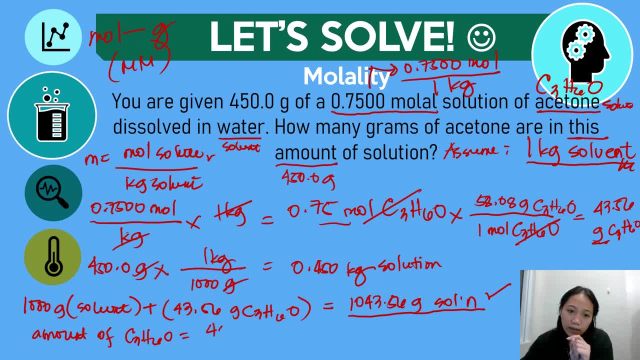 Kunin mo ngayon yung kinuha mo. You have now 450.0.. You divide it, Doon sa nitira yung total. Okay, Yung total, Kinukuha natin yung percentage niya. 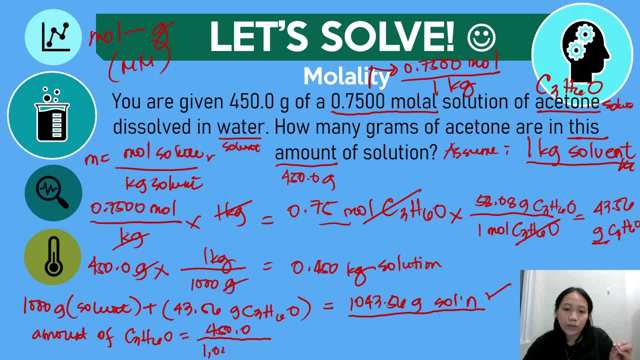 Kinukuha natin yung percentage, So you have 1,043.56 grams For you to cancel now grams. So ang nakukuha na natin dito is yung ratio nung nakuha natin na acetone. 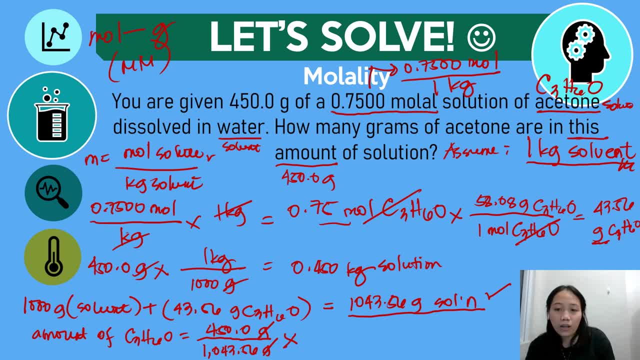 And you have to multiply it to the mole, or, sorry, to the grams of your acetone, Which is 43.56.. And this is that value. So if you're going to multiply that one and you have to solve, the answer would be 18.79 grams of acetone. 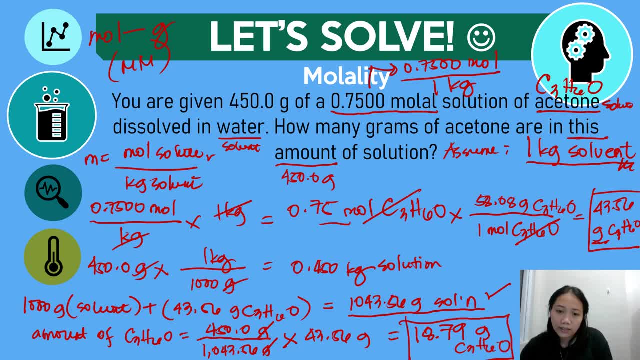 So this answer, the 18.79 grams of acetone- is the amount of acetone which is in the 400, which is in the 450 grams na kinuha mo. So kung kukuha ka ng sample na 500 grams. 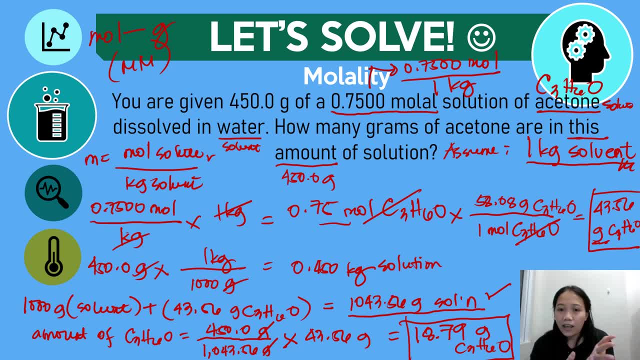 maiiba din yung number of acetone na naandoon. Pag kumuha ka naman ng isang kilo out of 1,043.56 grams, so maiiba din yung number of acetone na nandoon. 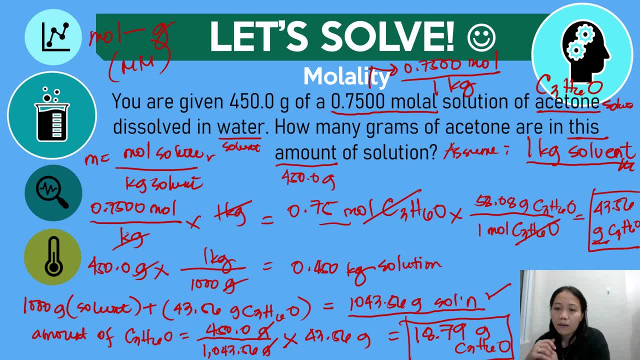 Okay. So, just like yung example ko kanina, that the amount of coke or the amount of sugar na nandoon sa coke, na ininom mo sa isang baso, is quite different from the number of sugar particles or the amount of sugar particles. 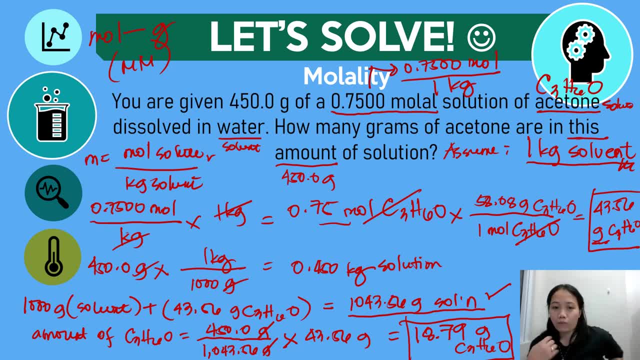 In the coke na natira doon sa pinangkuhaan mo. So yun yung pinaka-idea neto. So see, it's quite critical. That's why you need to make sure that you understand the whole idea of solution. 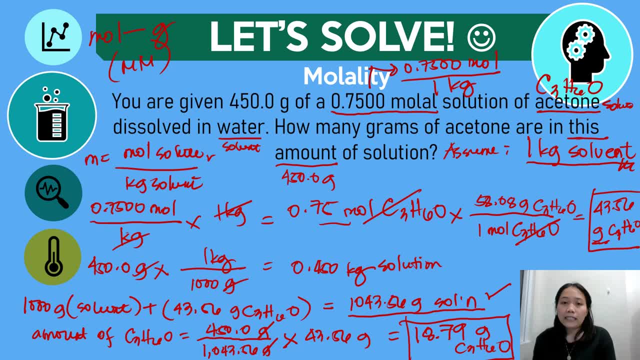 But just don't forget that you have to remember. you have to remember that a particular solute added to a particular solvent will always give you a number of solution. So what if that is the mass of your solute? all you have to do is to add it to the mass of your solvent. 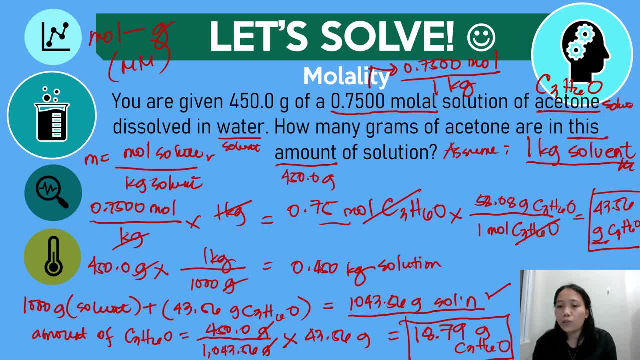 for you to get the mass of your solution. That is always the idea. So if you're looking for the kilogram of your solvent, then all you have to do is to look for the kilogram of your solution and the kilogram of your solute. 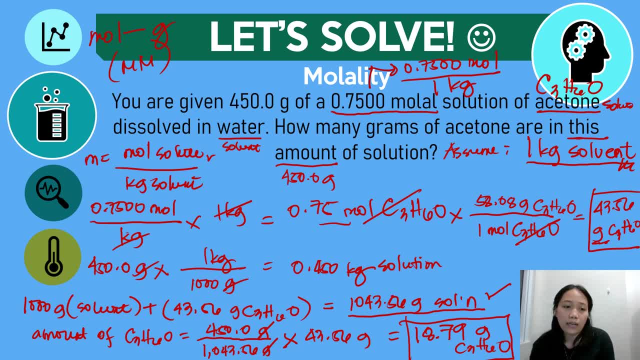 for you to subtract those two values and you will get the value of the kilogram of your solvent, And so on And so forth. So, as long as you know how, paano siya paiikutin or paano, paano atakihin yung problem, 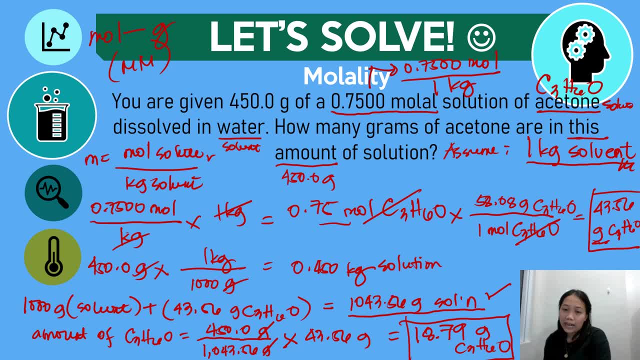 then you're good to go. So that is for molality, And that would be the end of the most talag na ito, a complicated part of the concentration unit That is molality, Simulality, lang yan. Now let's have the last part. 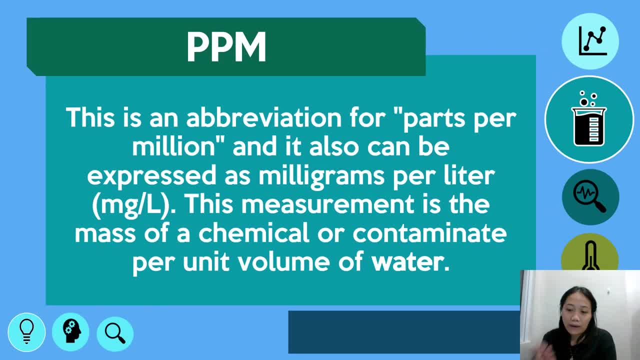 The one that I told you about. Okay, PPM, PPB and the PPP. So this particular unit of concentration is the one that will be used for you to express very small amount of concentrations, So these are widely used in testing. 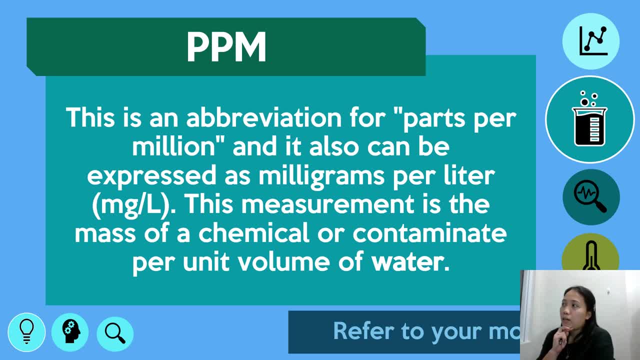 of, let's say, antibacterial properties. It could also be for antifungal, antimicrobial, any other products, let's say biomolecular activities, or um biochemical, ayun biochemical-related activities. You will be using the PPM. 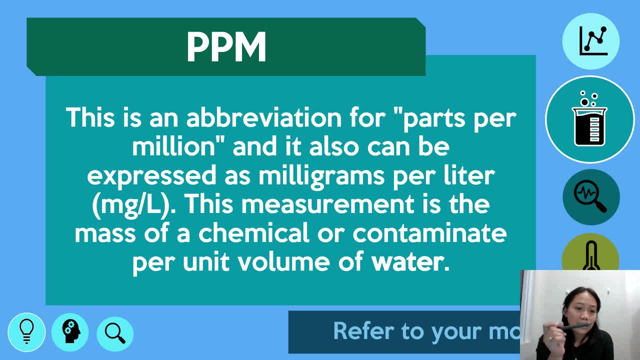 the PPB and the PPT. So if you're going to read some of your RRLs in your upcoming capstone, you are going to encounter the PPM, PPB and the PPP, Most likely the PPM. 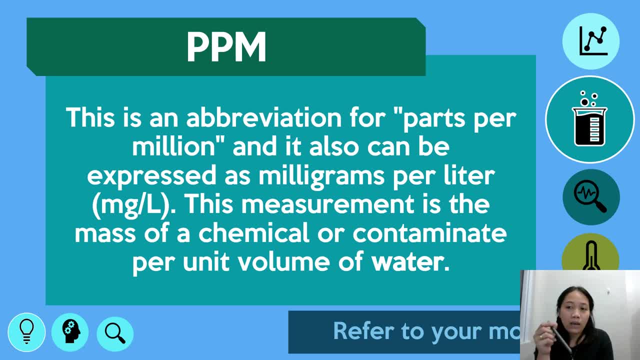 Medyo hindi naman na inaabot ng PPB sa mga ganong klase ng research. so yun ppm denotes our is an averbation, or four parts per million, ppb is parts per billion and ppt is parts per trillion. so of course sobrang liit na nun talaga ni ppt. okay now, um, most likely si ppm naman. 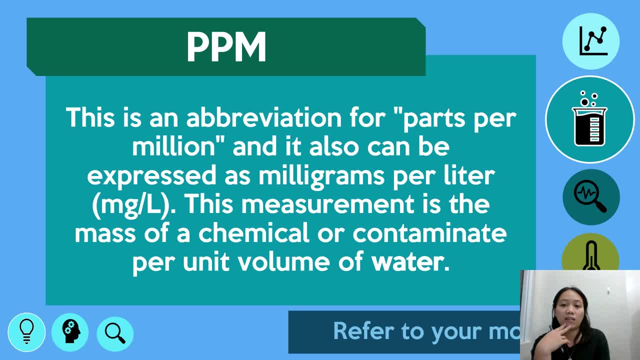 okay, hindi lang siya sa biochemical, it's also used in industrial researches, such as identifying the contaminants in a particular water. so take, for example, kukuha ka sa ilog pasig. so siguro may mga nakaisip ng ganitong research, kukuha ka ng amount of water dun and oh. 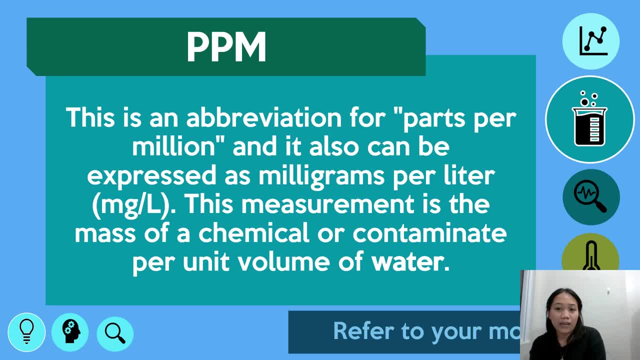 yeah, you're going to find the contaminant, let's say lead, okay, the lead content of the water. then you're going to use ppm because, of course, that is just very small amount, small amount lang, yung lead na nandoon, which is yun yung kailangan. hanapin mo. 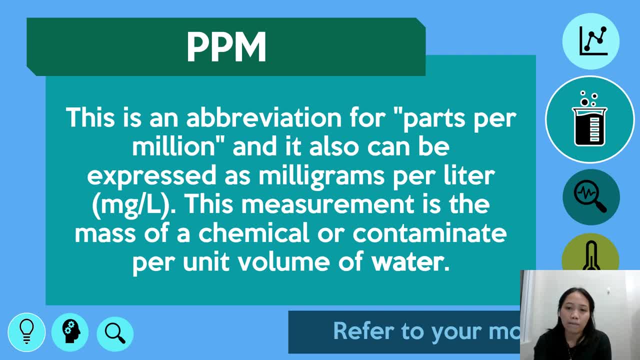 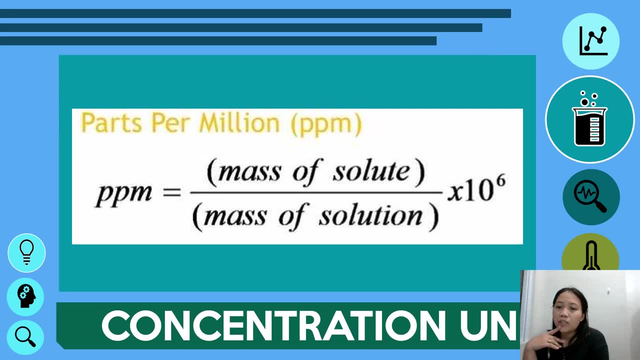 so that's it, that is ppm. now the formula for ppm. ppb is just like um percent by mass, it's mass of your solute divided by the mass of your solution and multiply it to 10 raised to 6.. 10 raised to 6 kapag ka ppm, because there 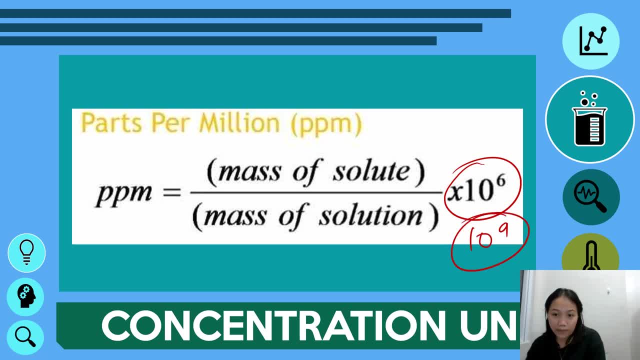 is million, 10 raised to 9. kapag billion, that's ppb, and for ppb that would be 10 raised to 12.. okay, and that would be just very easy, because some of the problems involving ppm is actually just giving you the values. 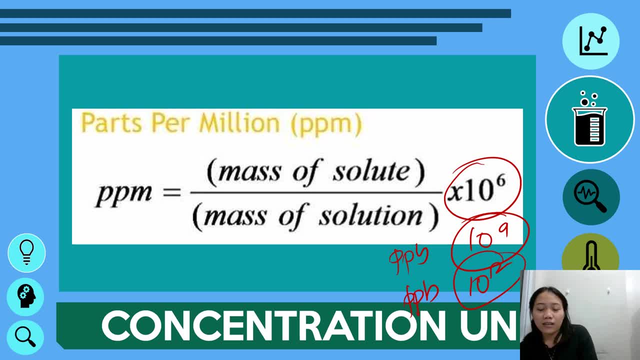 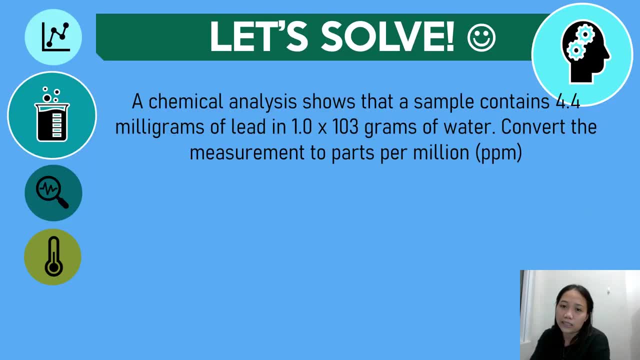 tapos directly is a substitute, malasha sa formula, then you're good to go. so take for example this one you have. a chemical analysis shows that the sample contains 4.4 milligrams of lead in 1.0 times 10, raised to 3 grams of water. so 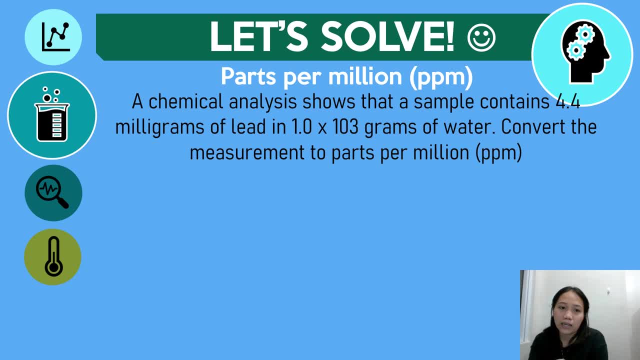 see um, you are identifying the contaminants, the contaminant which is, in this case, lead, in a particular amount of water. so convert the measurement to parts per million. so all you have to do is to write down the formula. so the formula is: ppm is equal to the mass of your solute, which is, in this case, we know is lead. 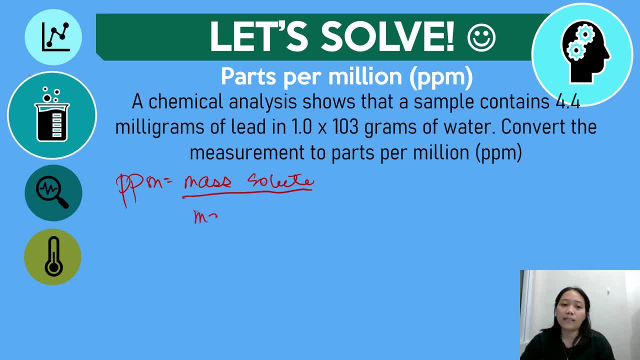 okay, divided by the mass of your solution, okay, times 10, raised to 6.. so the mass of your solute is actually 4.4 milligrams. okay, so you need to convert that one first into grams. so just the movement of zeros, kasi it's actually in the linear. 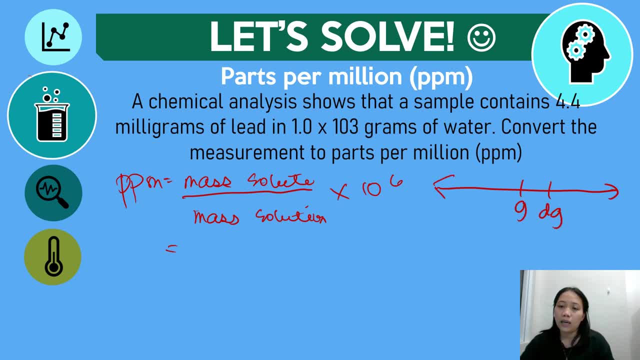 if you are going to recall, you have grams, that dc grams, you have the number nandito cg, the centigram and the milligram. so because you have a, grams are in milligrams given and you have the other as in grams, kailangan pagpareho mo sila, so it's. 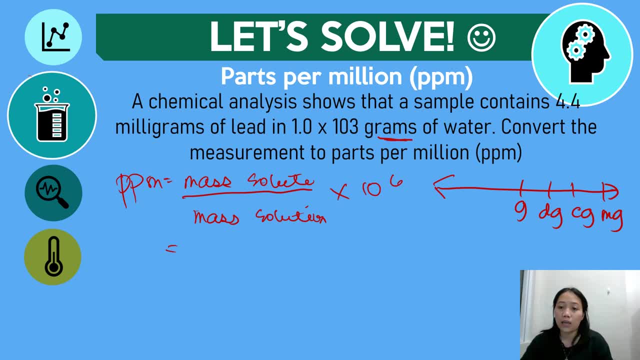 either i kukonvert mo to into milligram or si milligram ang i kukonvert mo into grams. let's choose the second one. so all you have to do is to move three uh three decimal points. say you will have 0.0044 grams of lead divided by the mass of your solution. 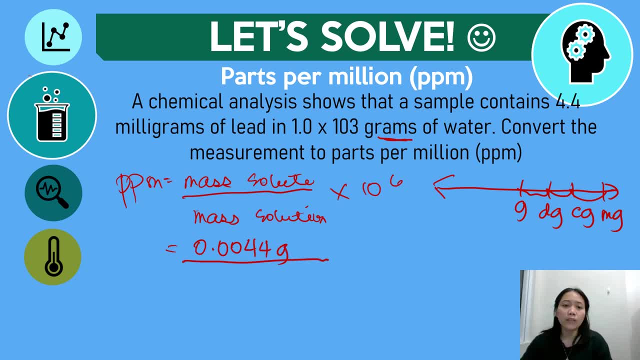 so again, mass of solution ang meron po tayo y grams ng water at grams ng lead, which is the solute. so you have to add the two 0.0044 grams plus you have 1.0 times 10, raised to six grams as ya general і gams. introduce mo po ang. 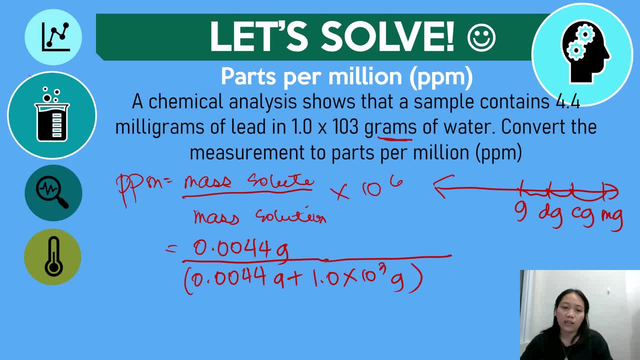 times per gram to three grams of water, and if you're going to solve for that, the value that you will get is 4, 4 ppm and kahit naka whole number yan. that is very, very small. okay, because you have parts per million. okay, so we use 44 because we need two decimal places. 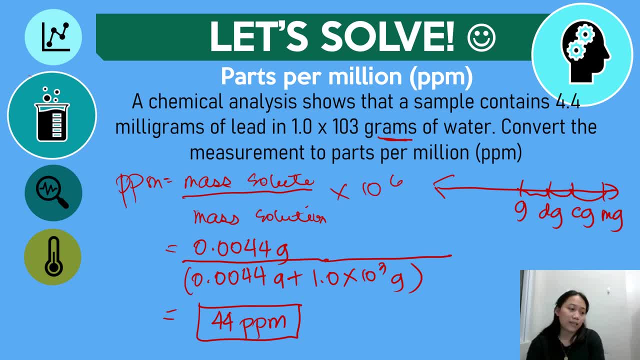 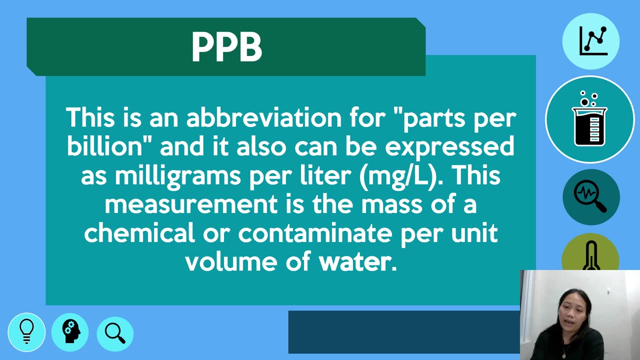 okay, because the least decimal places in the given is two. now another problem, which is the last one: the ppb. wala pala akong ppt example, but that would be easy lang, as long as alam nyo kaano yung multiplier. that would be 10 raised to 12. so ppb is the abbreviation for parts per. 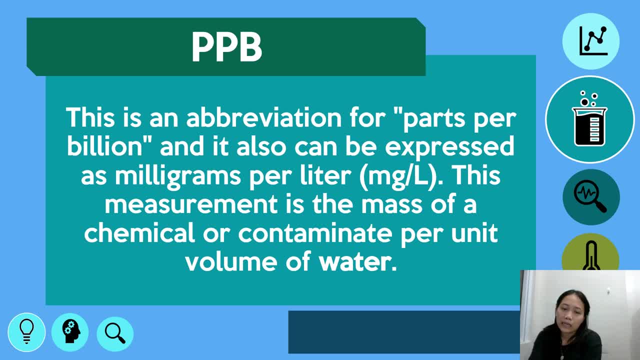 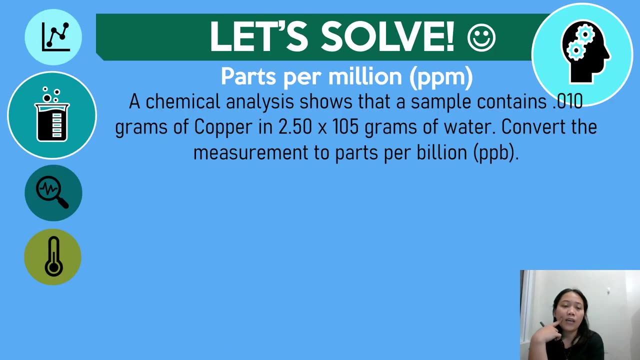 billion. ito naman sa very minimal amount lang ng contaminants. um, let's say, hindi naman contaminants, pero the amount of algae sa dagat you could actually use ppb, ppb there. okay, then let's have this problem. so you have 0.10 grams of copper? okay, a chemical analysis shows: 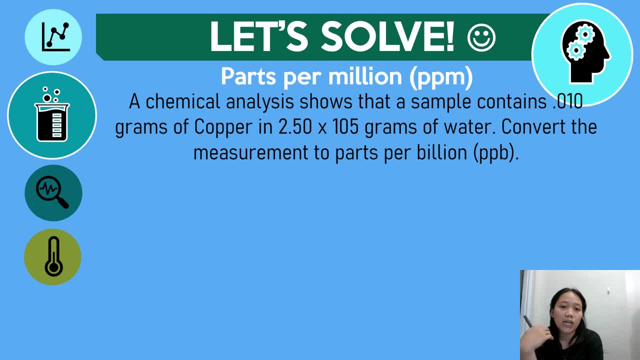 that the sample contains 0.10 grams of copper in 2.50 times 10, raised to 5 grams of water. convert the measurement to parts per billion, so of course that is just ppb. okay, ppb is equal to 0.10, 0.010, rather grams. 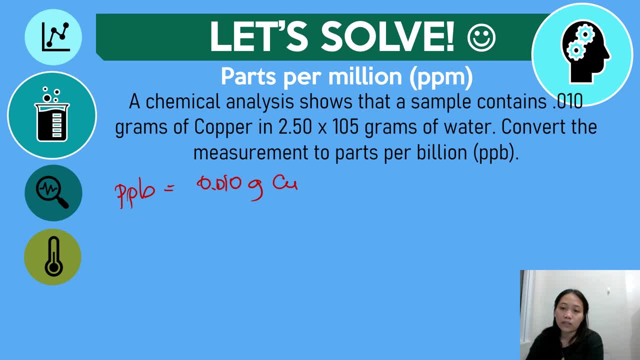 of copper. okay, it's already in grams. both of the values are already in grams, so no more conversion over 0.010 grams plus 2.50 times 10 raised to 5 grams of water, times 10 raised to 9, because this is billion, and you will get a value of 4.0 times 10 raised to 2 ppb, and that would be the answer. 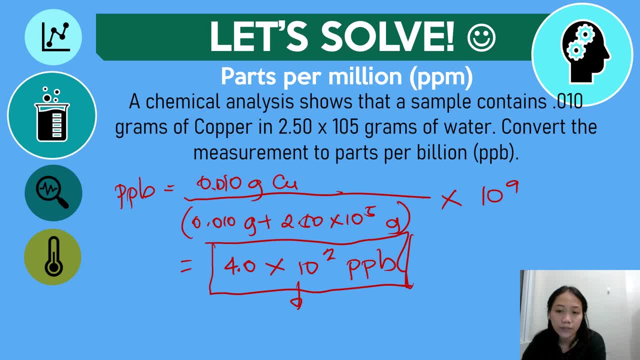 so all you have to do is to box the final answer: identify the number of significant figure. in this case, you have two significant figure, because you have 0.010. okay, so you have 2sf and your answer is 4.0 times 10 raised to 2 ppb. 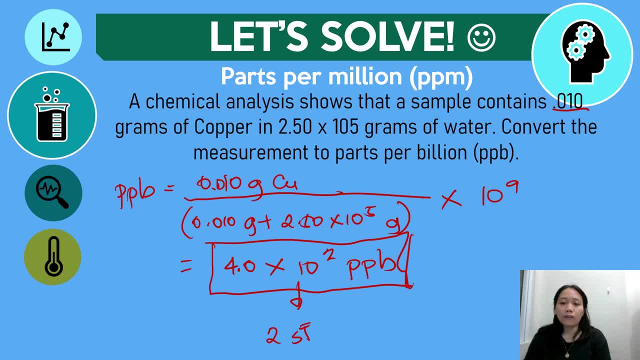 then that would be the end of our pre-recorded video involving concentration units. now, if you still have questions, you can reach me in the consultation period by 1: 30 to 2: 30 every day, from monday to sunday, and i will see you in the next video. bye, bye. 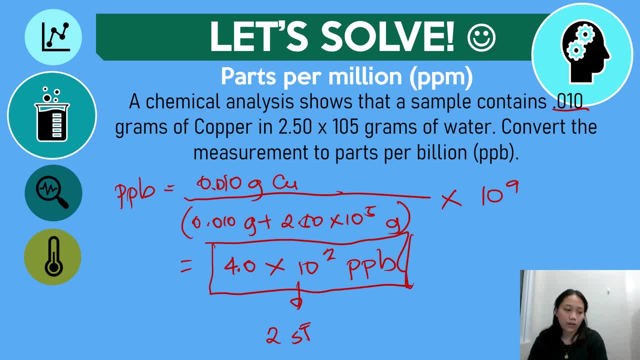 tuesday, thursday and friday, except wednesday because you have your club and advisory. so um, the next topic will be stoichiometry of solutions. i will just create another pre-recorded video for that one, and i hope that this will help you in having your summative test this friday. 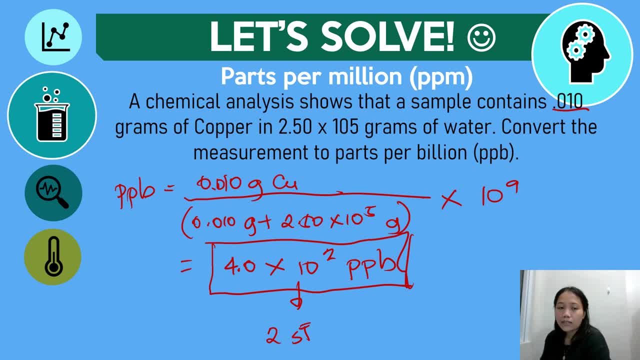 so thank you so much, and i hope that you learned something. goodbye everyone.